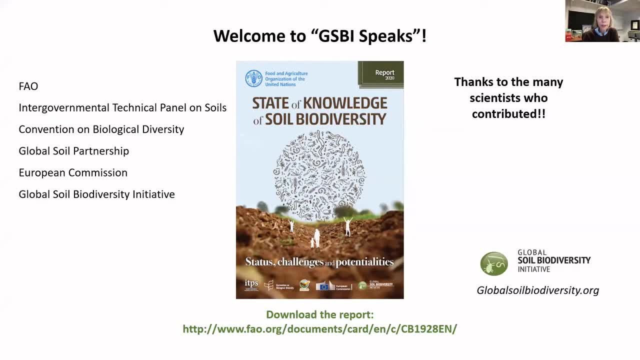 of this report: the Intergovernmental Technical Panel on Soils, the CBD, Global Soil Partnership, the European Commission and, of course, we also had a role. I'd also like to just say that the panelists are all going to be people who have worked. 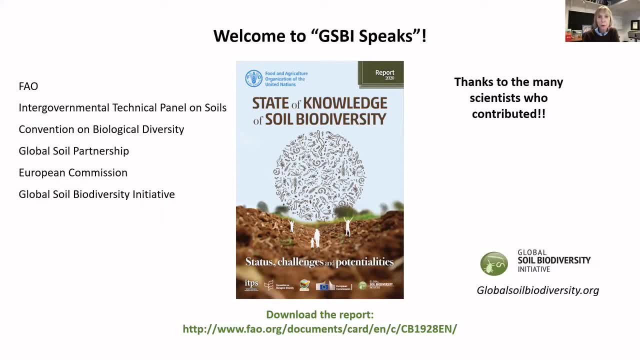 on this report, and so I want to give you some ground rules. I'm not going to spend much more time. I just want you to know that you can use the questions and we will be able to see your questions. We won't answer them by typing on there. We'll probably have 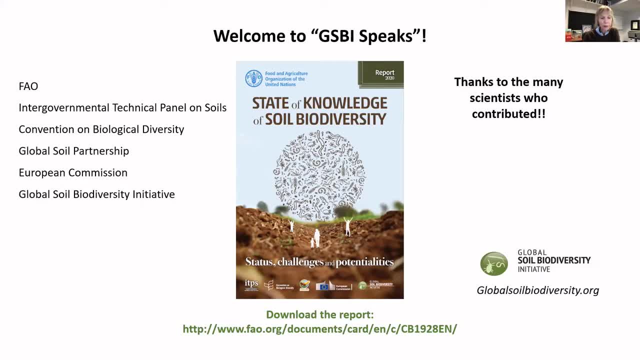 the panelists answer them. but you can look at that and put anything there, and maybe a different one. I'm going to give you a little bit of time. I'm going to give you a little bit of time to identify yourself. That would be very helpful. And if we don't get to your 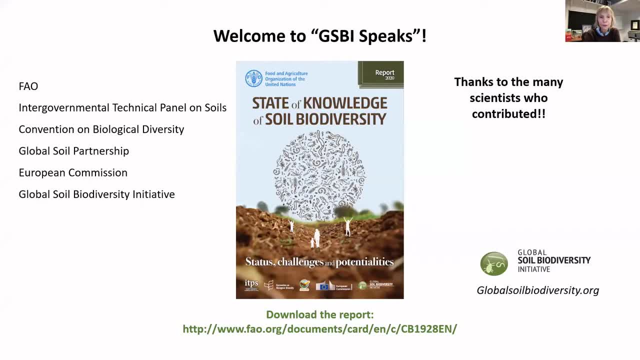 questions. it's just because we've got such a good discussion going, So I'm going to introduce now Kate Scow from the University of California Davis. Many of you may know Kate. She worked also on this report on the state of knowledge of soil biodiversity. 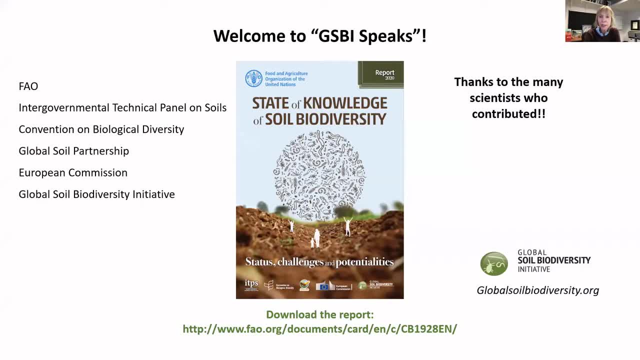 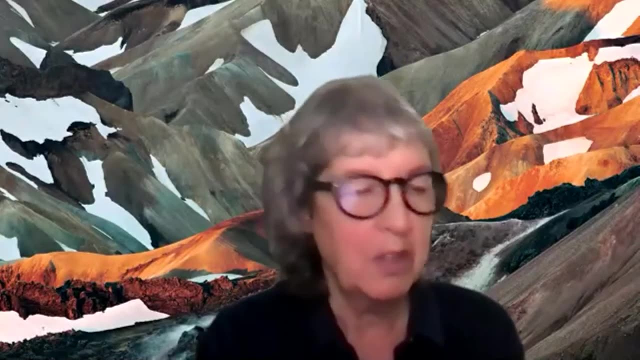 and we're really happy to have her and her expertise here as we see this new panel. She will introduce the panel. Thanks so much. Okay, Good morning for me, but something else for the rest of you. Welcome to the panel And, as Diana mentioned, this is the second. 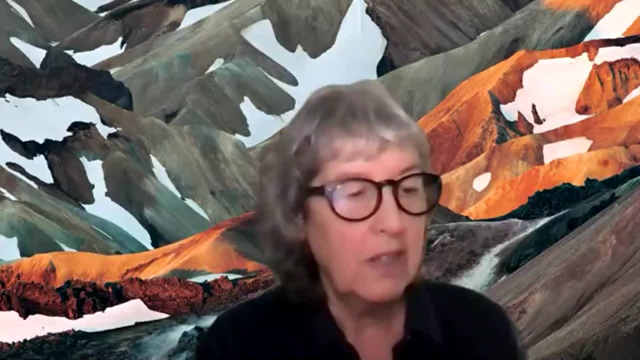 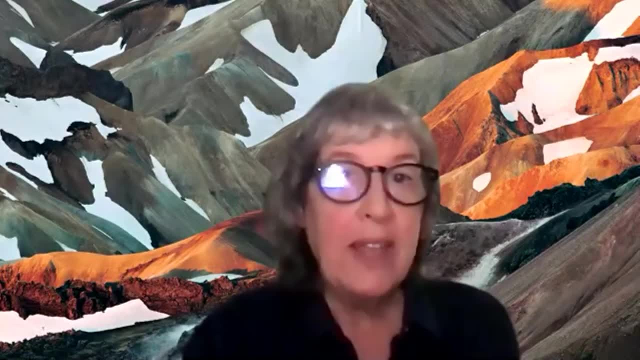 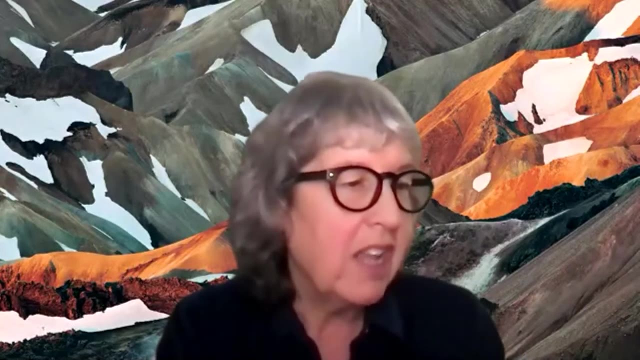 in a series of two webinars that provide opportunities for the coauthors to discuss the report and answer questions about it, And our panel today includes four very distinguished scientists. Charlene Janyon-Sheepers is a terrestrial invertebrate, ecologist and physiologist based. 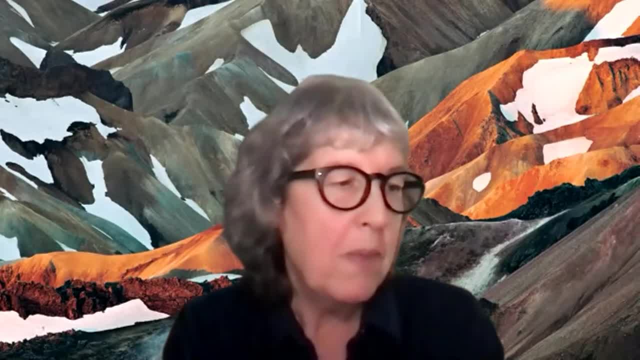 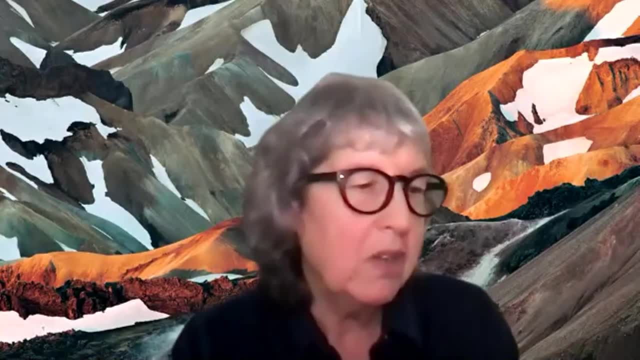 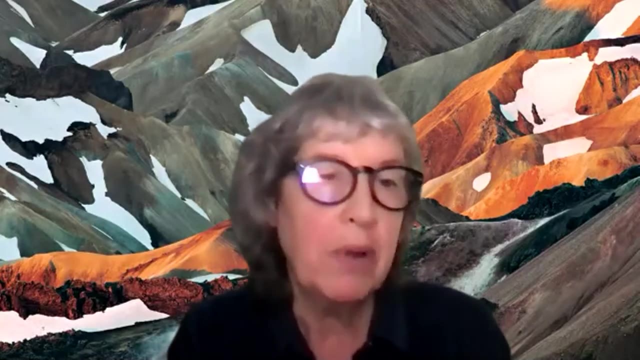 at the University of Cape Town in South Africa. Her main research interests include the adaptation and plasticity of invertebrates to climate change and how these differ between introduced and indigenous species. To answer these questions, she undertakes a multidisciplinary approach incorporating physiology, traditional taxonomy, DNA barcoding and ecology. She worked on chapter. 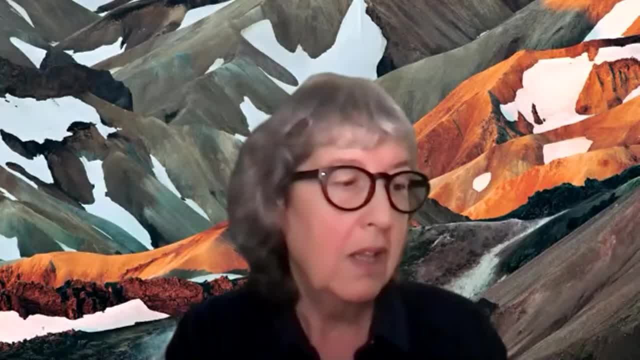 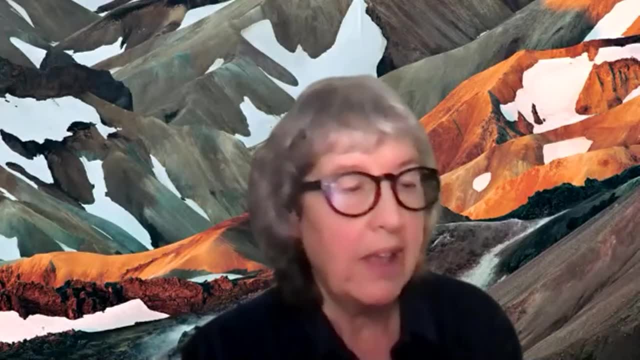 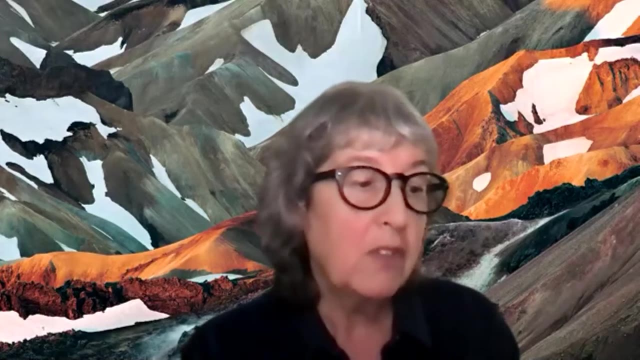 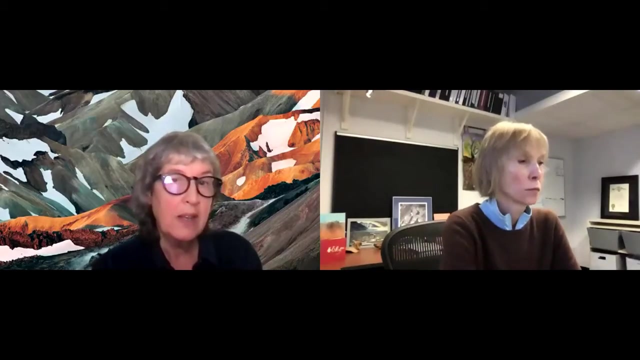 three: ecosystem, function and services. Our second panelist is Dr Junling Zhang, who's a soil microbiologist and ecologist based at China Agricultural University in Beijing. Her main research interests include the diversity and functions of soil microbial communities in agroecosystems, in particular, how soil microbiomes affect carbon and nutrient fluxes. 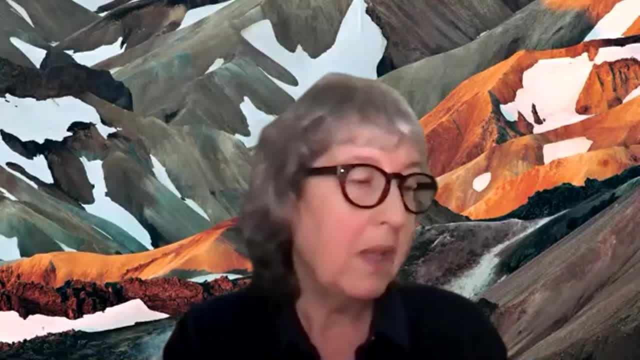 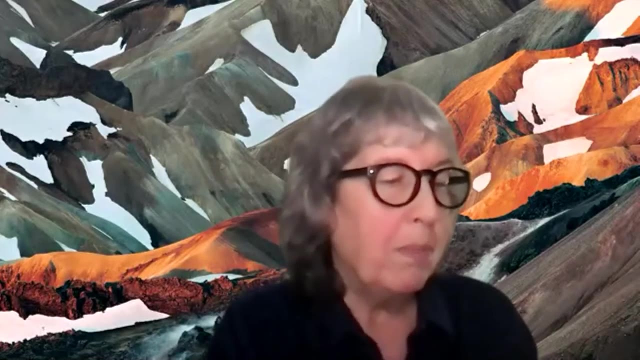 crop productivity and health. Her overall goal is to develop integrated management strategies to build up healthy soils for sustainable agriculture. She was the co-lead author on the Responses and Opportunities, chapter five. Dr Lauren Byrne is a professor of biology and environmental science at Roger. 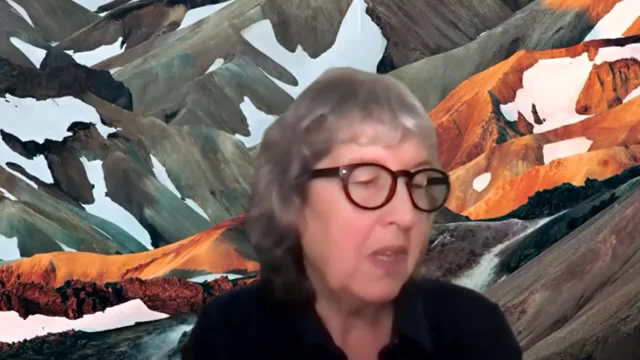 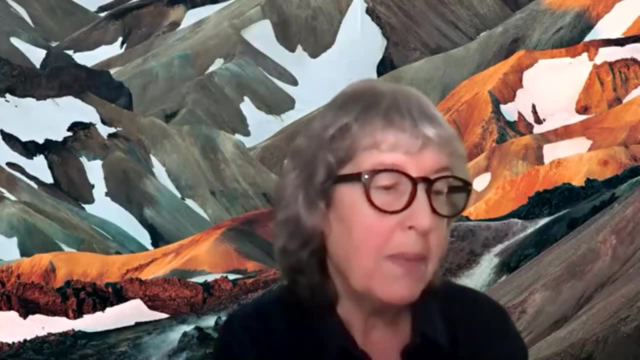 Williams University in Bristol, Rhode Island in the US. He's an urban soil ecologist whose research is focused on the effects of lawn and carbon garden management on soil invertebrates and biogeochemical cycling. With his career at an undergraduate institution, he spends most of his time teaching, including a soil ecology class. 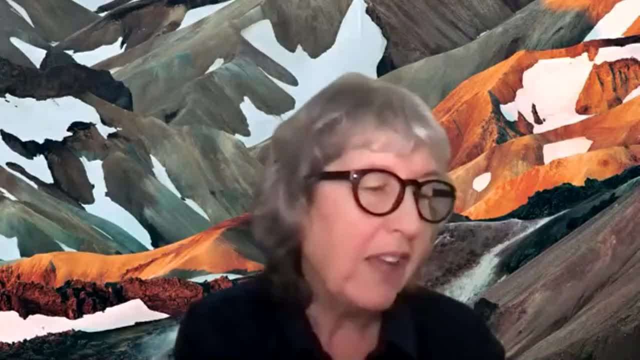 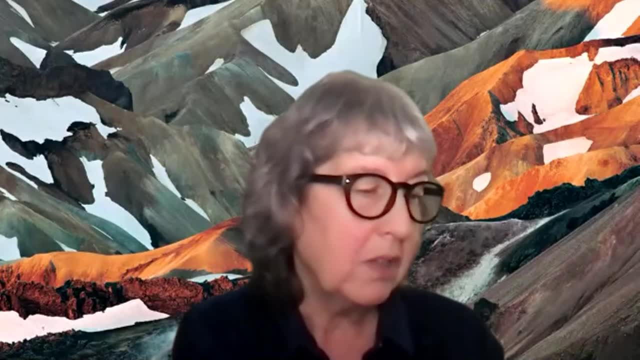 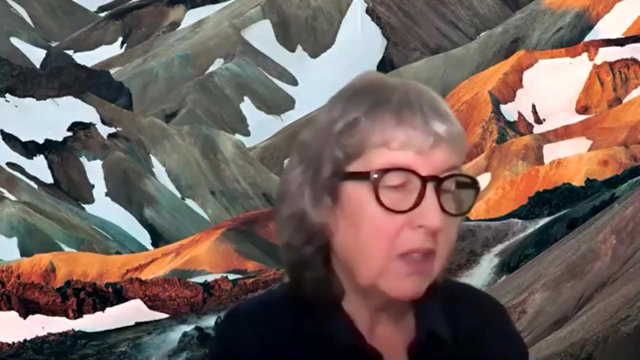 and developing new ideas and lessons for effective environmental education. In addition to editing a book of teaching activities and writing other articles about teaching, he's organized educational sessions at meetings at the Soil Ecology Society, Ecological Society of America and the University of Michigan. Dr Byrne is a professor of biology and 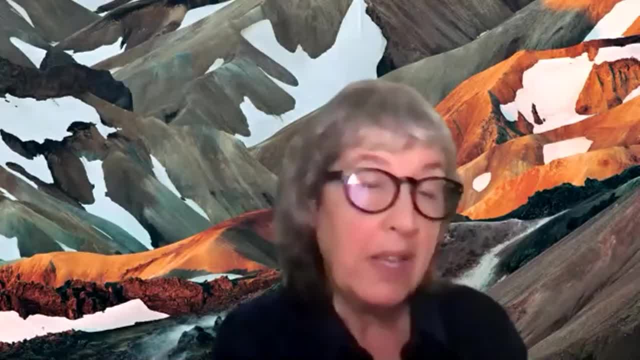 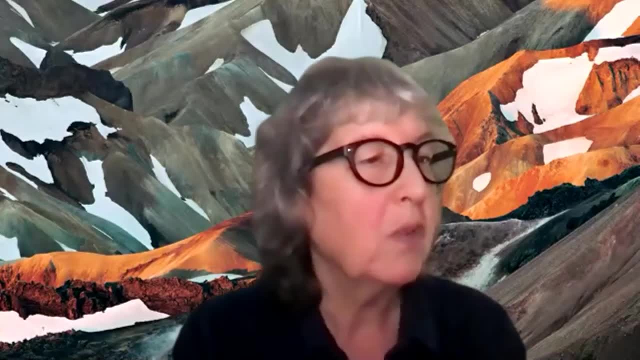 technology at Okay, rock and razem and a study group in Scotland, Byron vita, on soil diversity initiativeふび missoula, He engage s veces en Smart eighth project with a global style bit soil biodiversity initiative. he'll be presenting on outreach and education for soil biodiversity, which is part of chapter 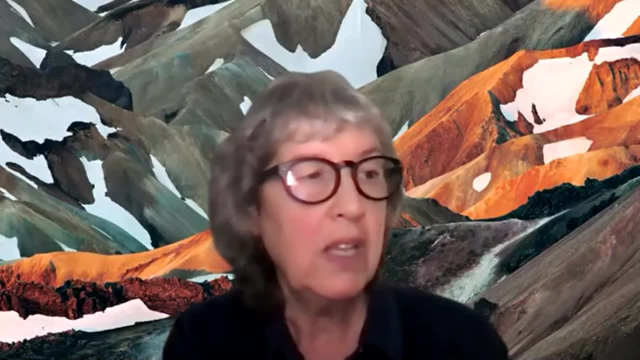 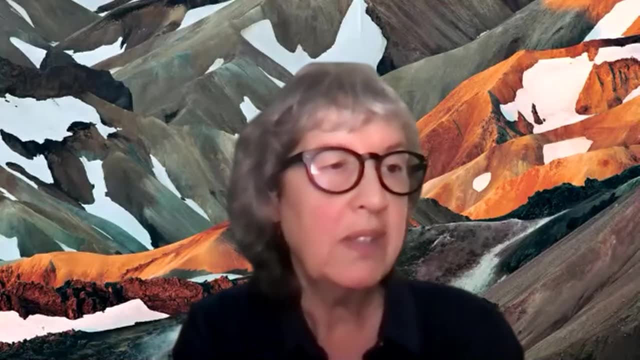 five. And then finally, Dr U howem ban prayers. buten is a terrestrial ecologists based at the Netherlands institute of ecology, who is a professor of functional biodiversity at W соп Ngâcmares university in the Netherlands. Weid, among other thingsabord en From. 2030, a primary Salesforce, and he has a broad interest in soil biodiversity and works on r. yang interpr impartiera includes theравm anteer yakamentomakwaring någonting nodig? downfalle, transportation, deeper generations of fields from local cultures. policy life Hatoum's question n. 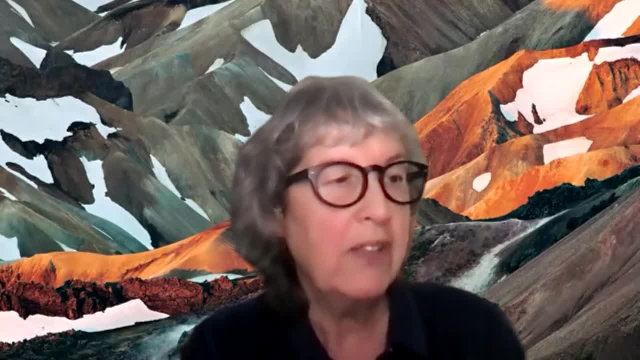 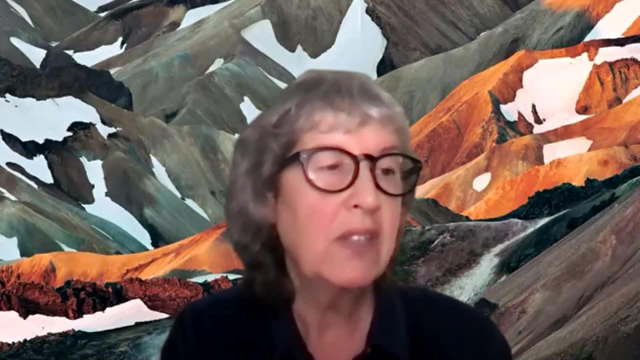 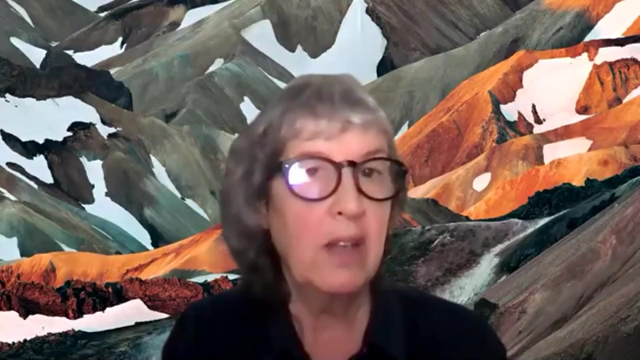 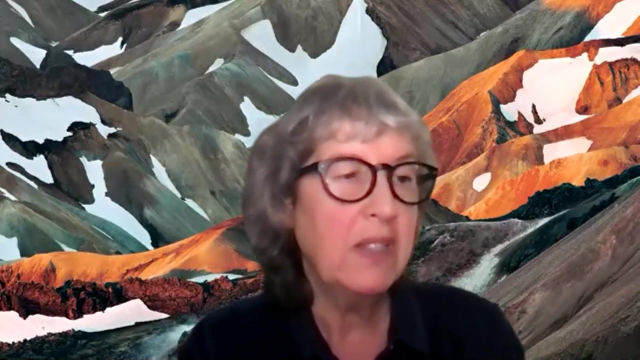 below ground interactions between plants and soil, biota influence, above ground biodiversity and the composition and functioning of ecosystems under climate and land use change. Wim was on the editorial board, so was responsible for the overall report and final recommendations. We're asking each of our speakers to use about five minutes a piece to touch upon. 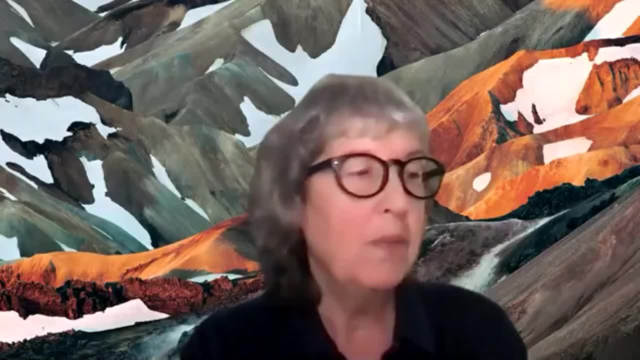 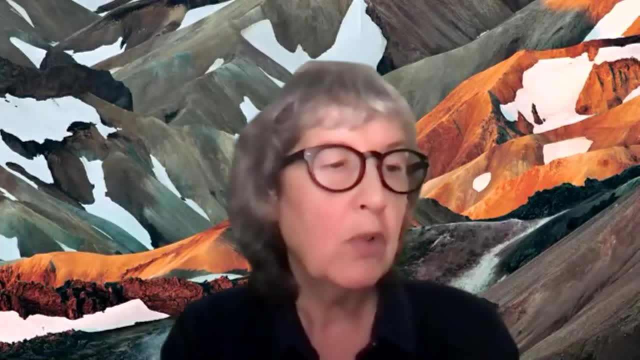 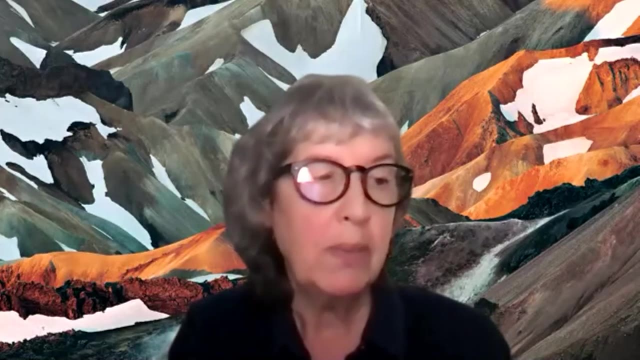 the following topics. First of all, why did you choose to contribute to the FAO report? What are your takeaways from the chapter of the report or activity you contributed to? How do you see the information from the chapter you worked on, contributing to soil biodiversity research? 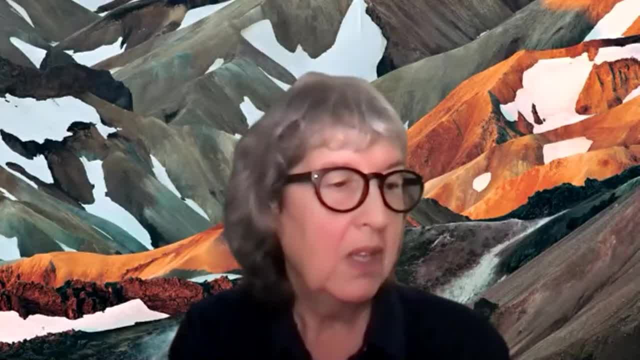 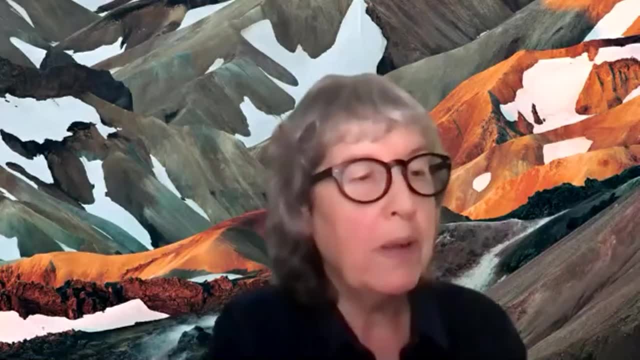 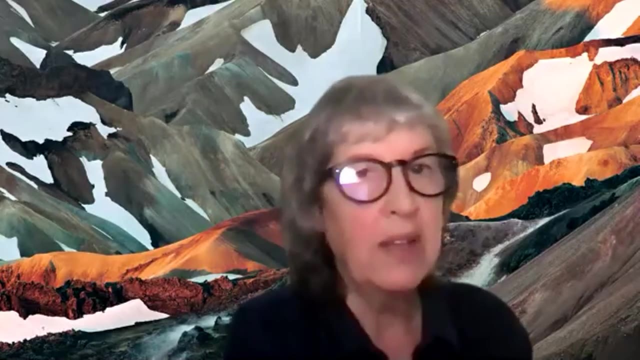 education and or policy. So Diana set the ground rules. After the panelists have finished their opening remarks, we're going to open up things to you For discussion and you're going to put your questions in the Q&A box, in the Zoom and again. 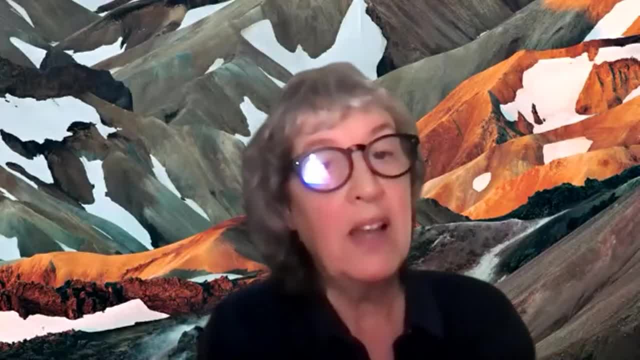 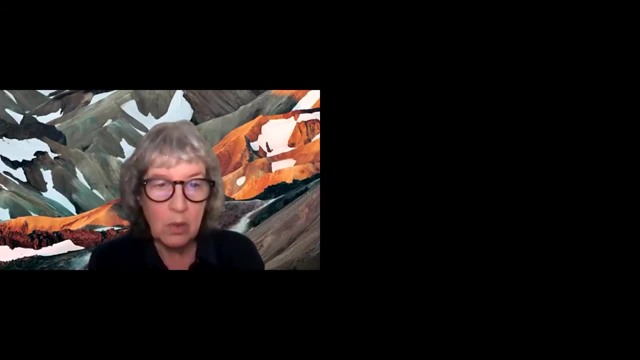 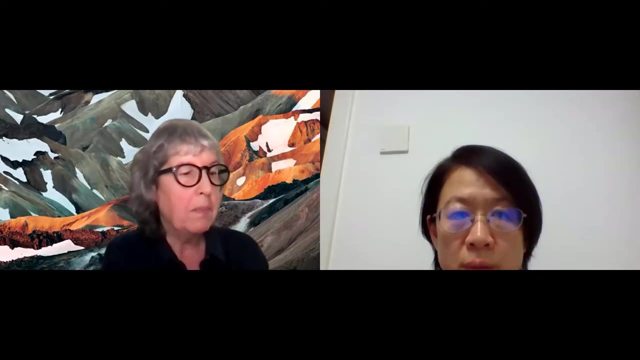 apologize if there's going to be a lot of questions. we may not be able to get to all of them. So before I started, though before we start this, I wanted to say a few words about biodiversity and this groundbreaking FAO report: So soils. 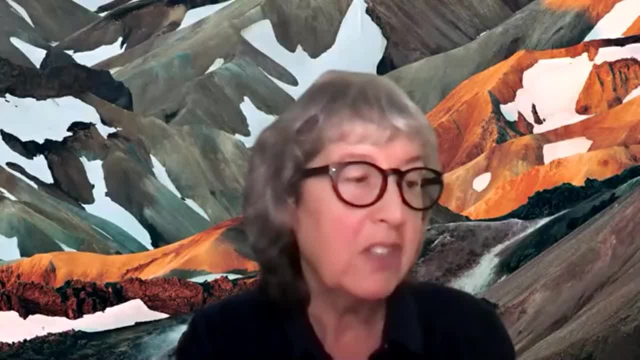 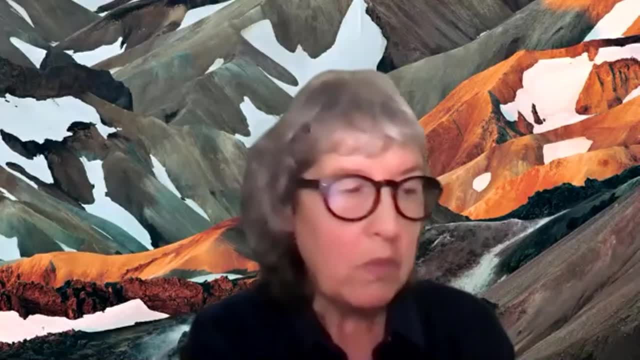 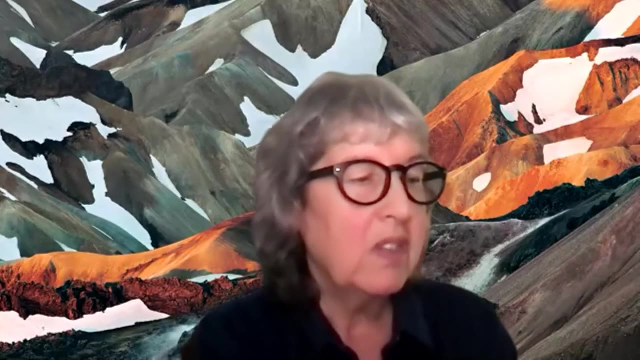 tucked away under our planet's diverse and magnificent terrestrial ecosystems are obscure and hidden, despite the fact that soils are bursting with life, hosting over a quarter of all species on earth and some of the most biodiverse ecosystems. Society values and counts on many of the ecosystem services provided by soil. 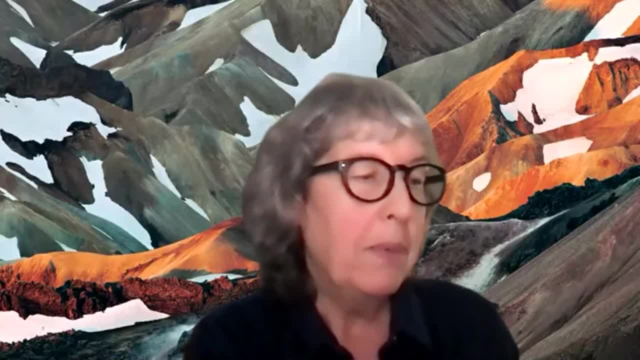 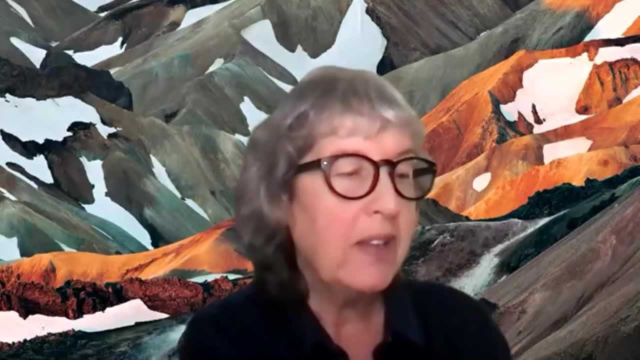 food, climate regulation, disease suppression- much more. but many aren't aware that these services actually come from the soil, So I'm going to give you a little bit more detail on that. Soil is a biodiversity. We take these services for granted, which is a problem. 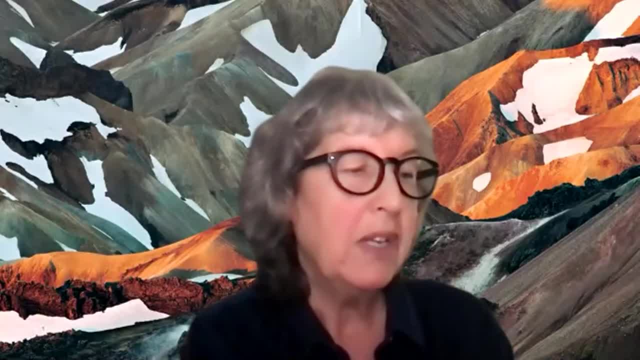 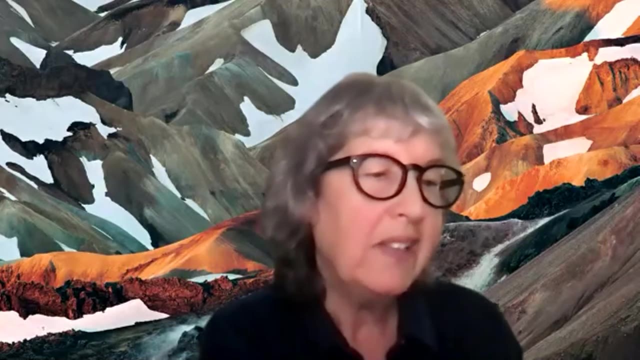 If we don't understand that living beings and their communities underpin these essential services, we won't know how to protect them and ensure their sustainability. The early conservationist Aldo Leopold got it over 70 years ago. He wrote: our task as humans is not to save the environment, nor to preserve things as they are, but to engage. 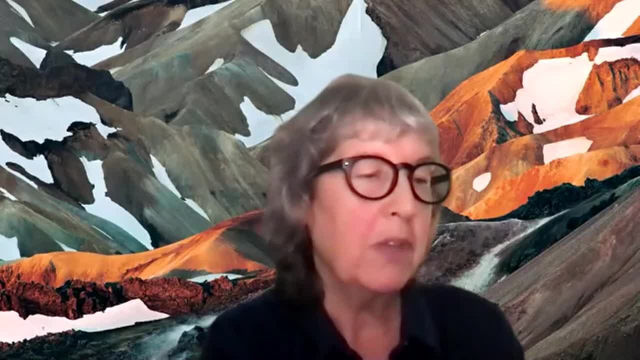 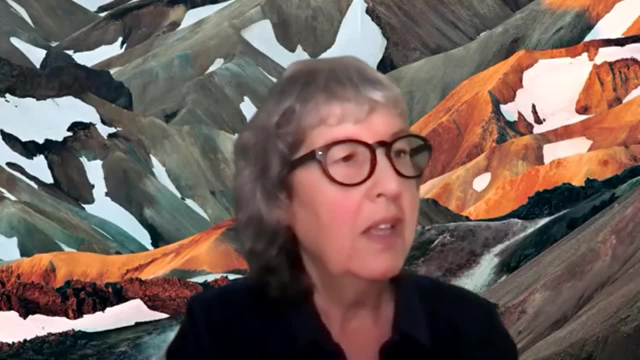 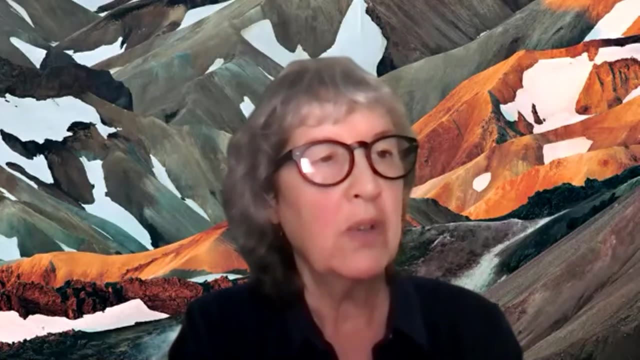 the environment in ways that revitalizes the biotic community. This soil biodiversity report provides a lot of ideas on how to do this. Also, over the past decade, there's been a growing recognition that earth's biodiversity is crucial for human survival and also in its own rights. 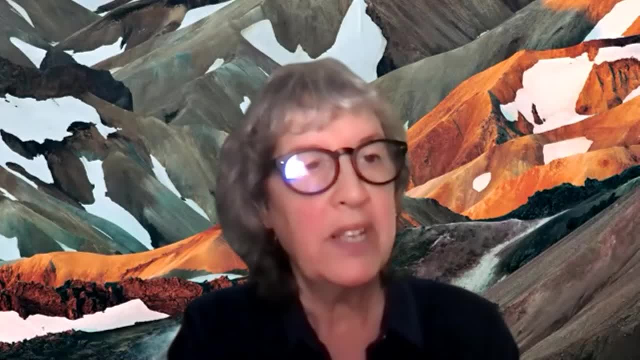 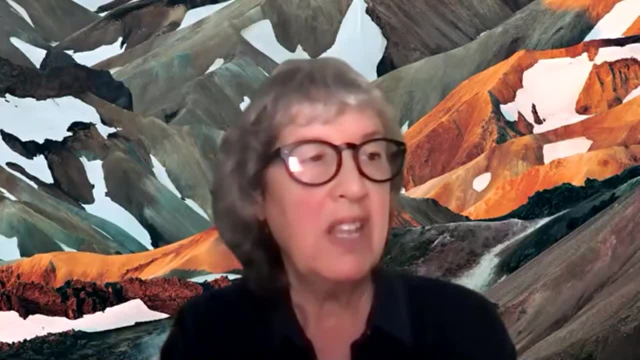 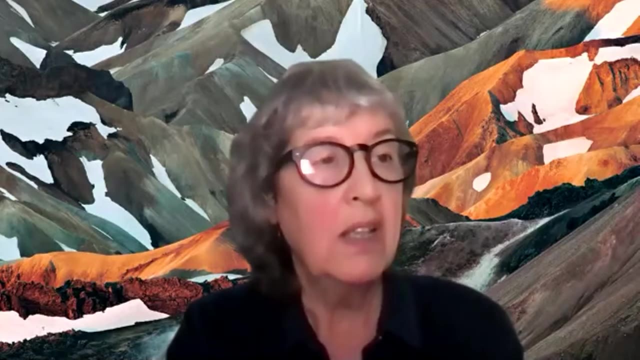 However, global biodiversity assessments and measures for its protection more often than not do not include soil biodiversity. So biodiversity has unique challenges, needs specific protections and requires policy recommendations that may not be considered in existing assessments of biodiversity. This report contains many suggestions and ways forward to address this gap. 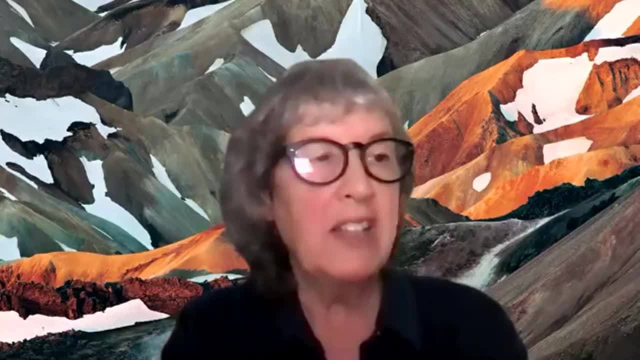 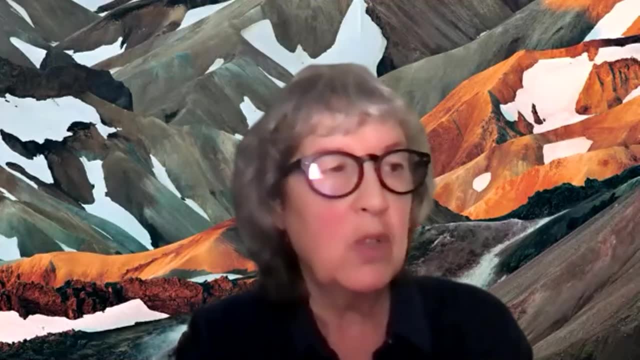 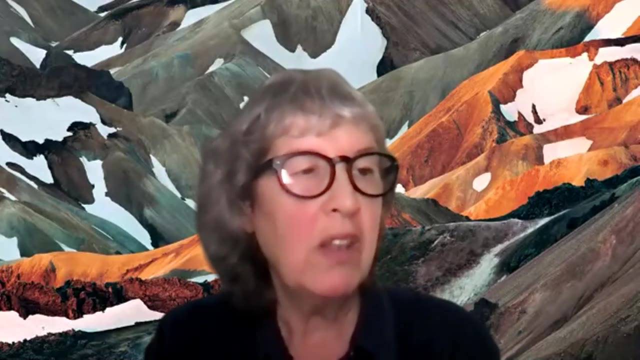 Third, countless children are attracted to marine biology and its charismatic megaphonic. It almost seems like a rite of passage. They are not similarly tugged towards soil biology. Why is that? The report's unabashed celebration of life, of soil life, provides many reasons why children and others of us should be. 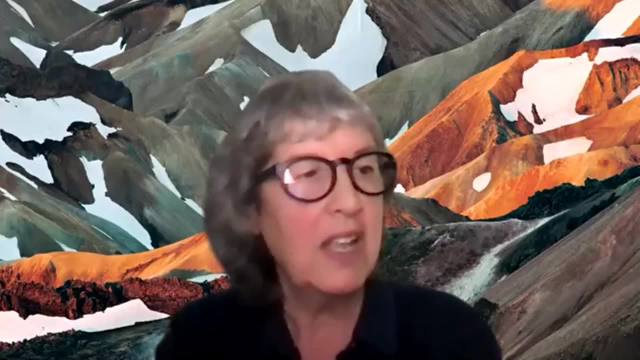 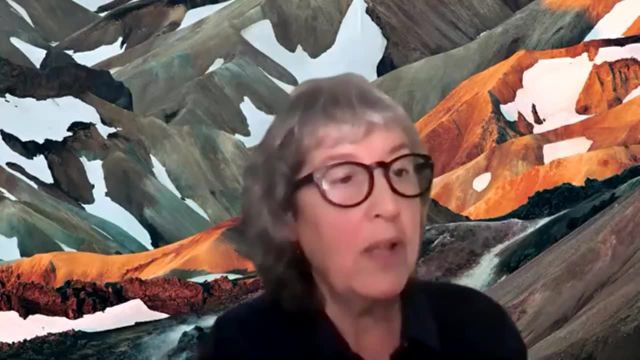 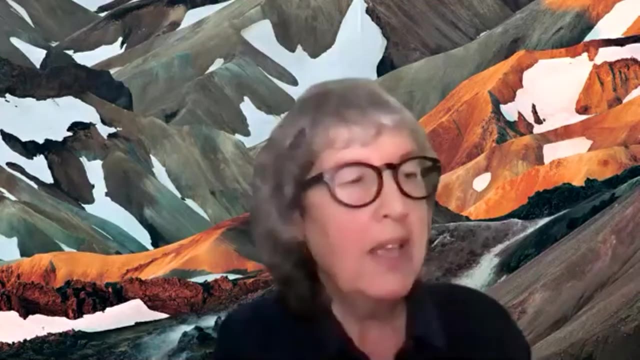 attracted and ideas on how to bring this about through education, outreach and other means. And, finally, increasing knowledge and literacy and passion, in particular, around soil biodiversity is essential to draw on the diverse community of stakeholders required to discover and implement biological solutions for the daunting challenges we face. 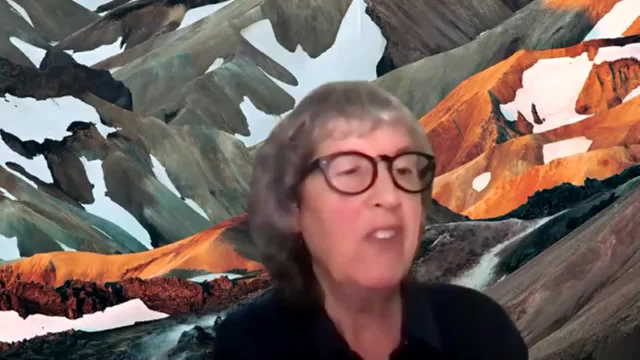 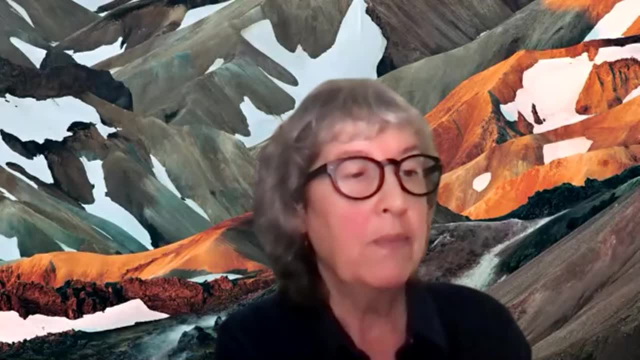 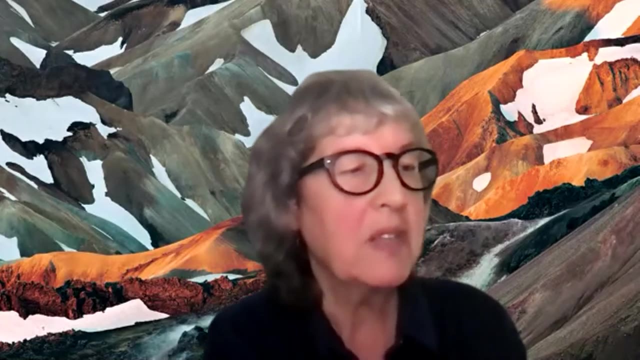 Climate change, agriculture, ecosystem restoration, environmental pollution and human health. Again, this soil biodiversity report is the place to get started. It represents a diversity of regions and nations and provides a wealth of principles, examples, actions and solutions to bring soil biodiversity into the light. 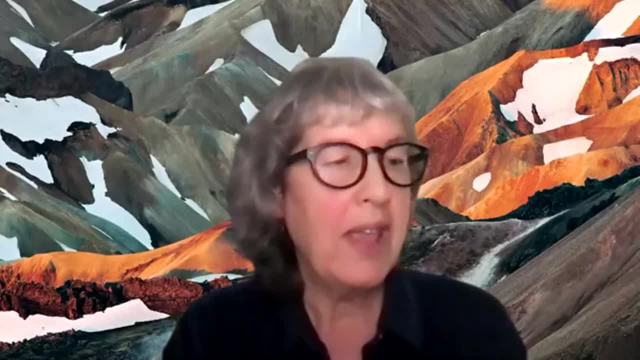 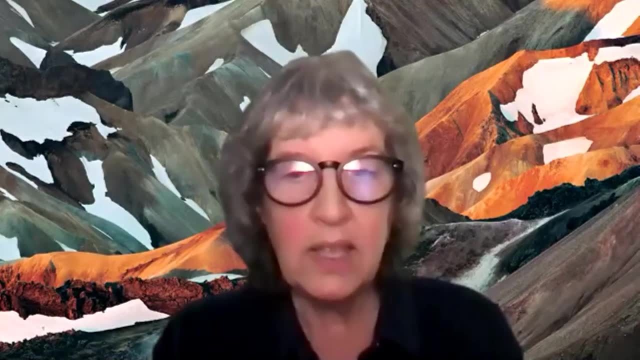 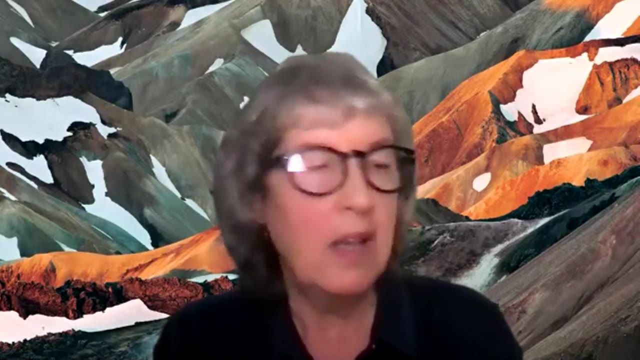 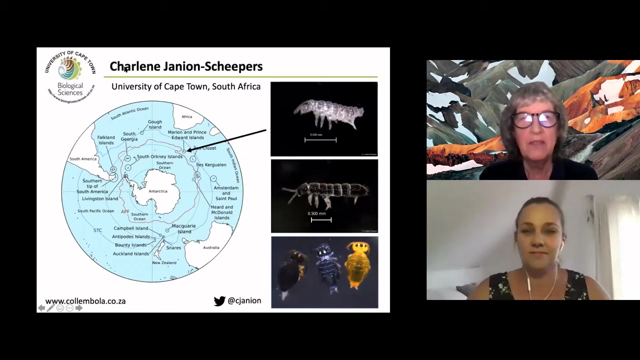 So, on that note, I'm going to now hand things over to our panelists And we are going to start with. we're going to start with Charlene and take it, please. Thank you for that, Kate. I'll just check. can you hear me and see my screen? 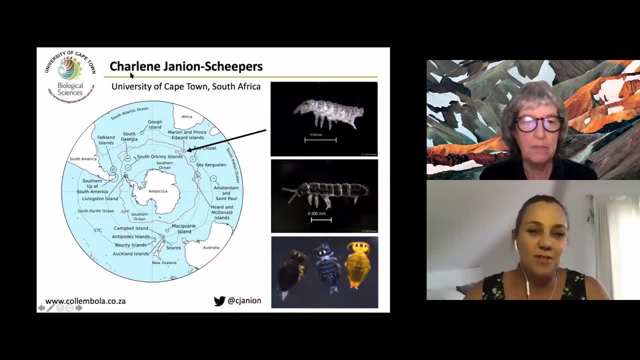 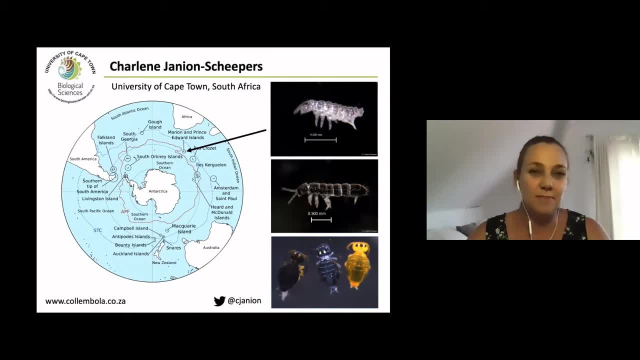 Yep Great. First of all, thank you so much for the opportunity. It's a real honor to be part of the discussion. Thank you, Thank you for the opportunity to be part of this webinar today. So, as Kate mentioned, the first question we were asked to talk about. 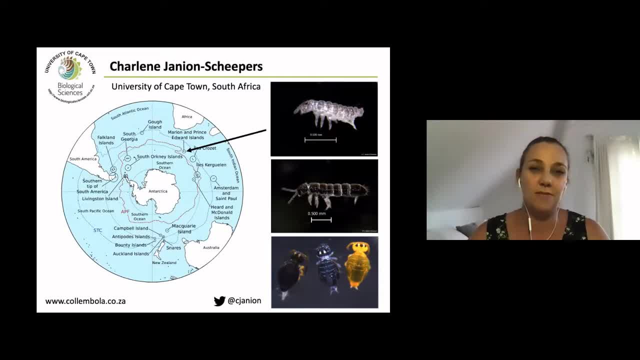 is why we chose to contribute to the FAO report. as a researcher- And for me this was an amazing opportunity to increase the awareness of soil biodiversity and inspire new research, And I realized my whole career was actually inspired by a report published in 2005 called the Millennium Ecosystem Assessment. This report focused on the impacts of global change. 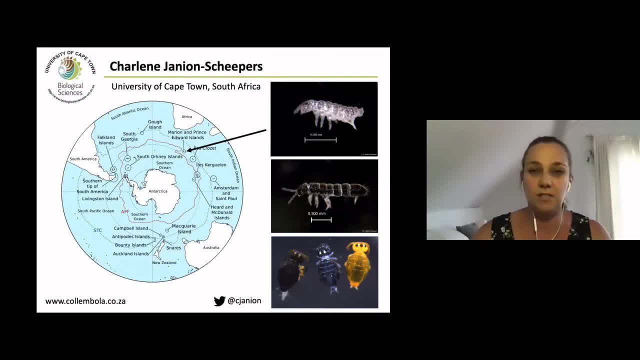 drivers on our planet And it really shaped my research interest on the synergistic effects of invasive species and climate change. My research started on sub-Antarctic Marion Island, which is shown here on the map. Sorry, Shown here on the map. 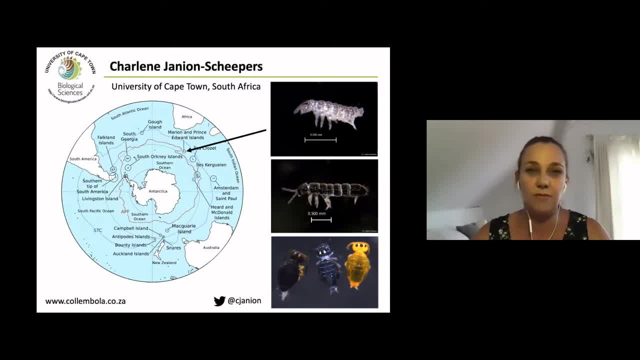 And on this island I worked with my mentor, Stephen Chown, and we focused on the wonderful critters called springtails or columbula, And we compared the traits between indigenous and invasive species. We found here that invasive columbula have much. 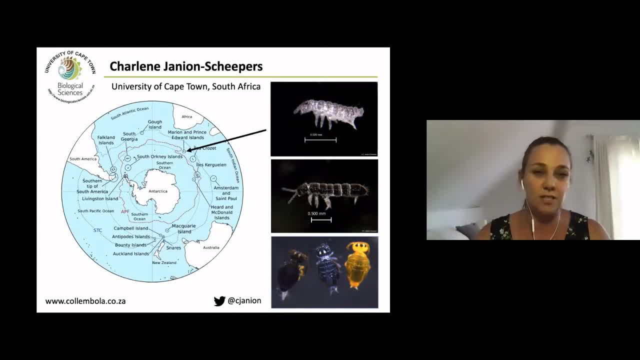 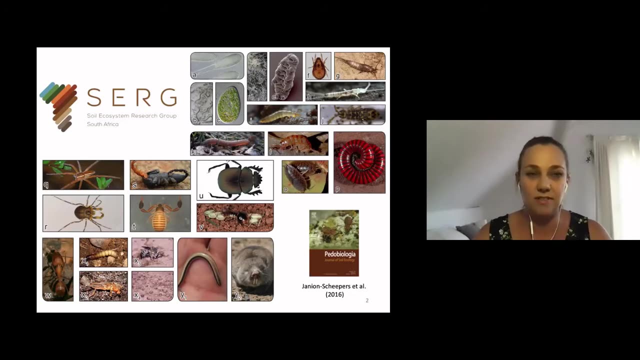 broader thermal tolerances, They perform better than indigenous species. so under climate change conditions, so under warmer and drier conditions. And I then switched my attention to mainland South Africa, where we are very lucky to have many charismatic animals, both marine, as Kate mentioned, and terrestrial animals. But our 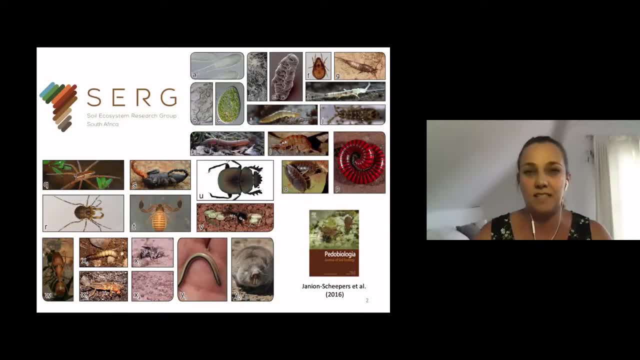 research on soil biology has not been as extensive, and this is partly because of lack of taxonomic expertise. So I really became fascinated with columbula, diversity and taxonomy at the tip of Africa, here in the Capitturistic region, And this was inspired by knowledge. 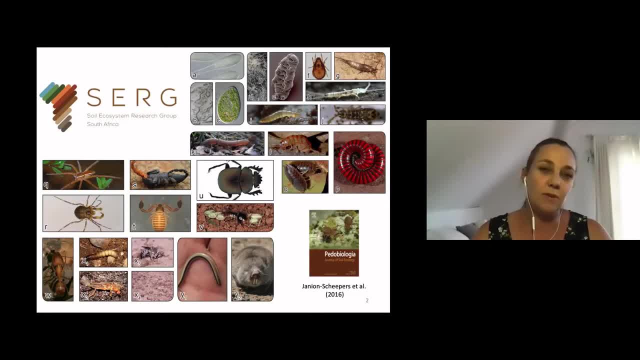 exchange projects with European colleagues. Then we were also inspired by several collaborative projects, such as the Global GSP I and others, And we formed the Soil Ecosystem Research Group in 2012,, which enabled soil biota experts in South Africa to put our heads together and address this huge knowledge gap in our region. 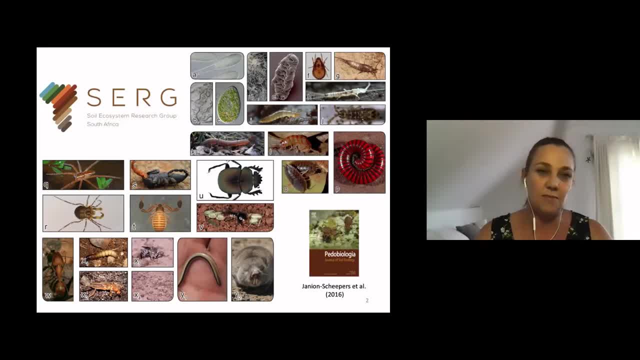 And we found that we have an extraordinary mega diverse below ground diversity with high endemism. So through that process I also became more interested in agro ecosystems and in using Calembola as bioindicators. So this was a very long background just to show you how my research actually led me to be able to contribute to this report. 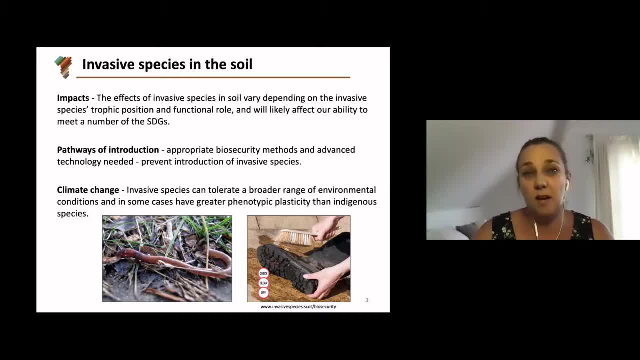 And the second question we were asked is to just give you a summary or takeaway of the chapters we were involved with. The section I co-wrote with Erin Cameron concerned invasive soil species. So, in summary, we found that the effects of invasive species in the soil really vary depending on the species trophic position. 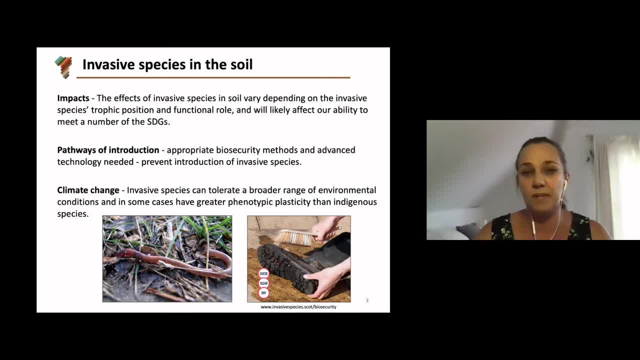 And the functional role, and it will likely affect our ability to meet a number of sustainable development goals. The impact of largest soil fauna, such as earthworms and ants, have been reasonably well investigated in certain parts of the world, But overall, the information on the impacts of most of the taxonomic groups in the soil are lacking. 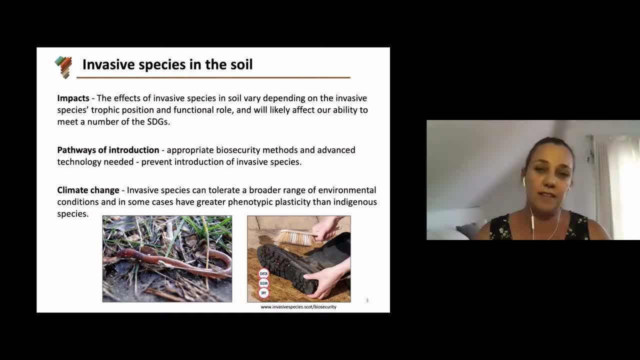 Appropriate biosecurity methods are really needed to prevent the introduction of more invasive species, And also the accurate identification is very important, So we need more taxonomists, of course, While DNA barcoding is a useful tool that can be used for the early detection of invasive species. 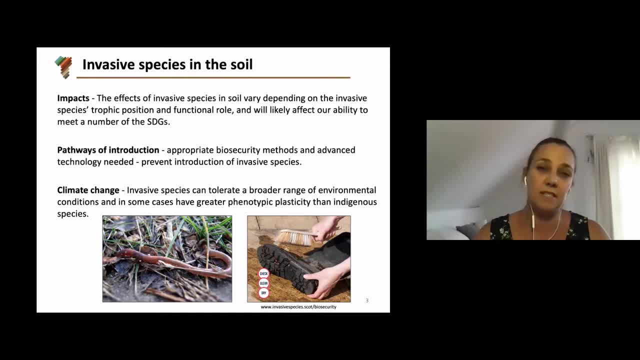 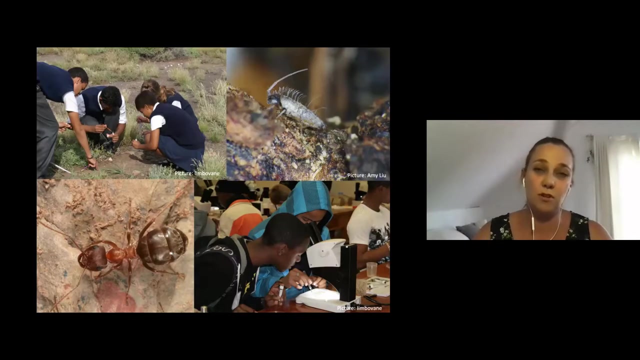 Now, from our physiological research, we found that invasive species can tolerate a broader range of environmental conditions than indigenous species. So the understanding of the physiology of species can really help us to understand their responses to global change. And the third and last question we were asked to talk about was how can our contribution also contribute to further research and education? 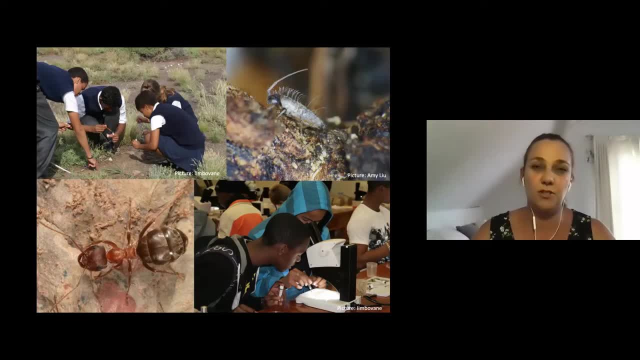 And I really hope that our section we contributed to will increase awareness about the impacts of soil invasive species and also the importance of stricter biosecurity protocols to prevent further introductions. I also hope it will highlight the importance of baseline physiological data to understand The response of species to global change drivers such as climate change. 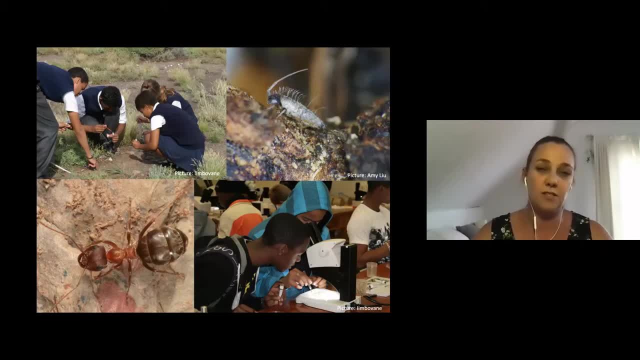 Now other panelists will talk about outreach projects. I just wanted to highlight a project in South Africa where we will definitely use this report as an educational tool. This is a project called Imbuvani and they're a high school project that uses ants to educate high school learners about biodiversity and invasive species. 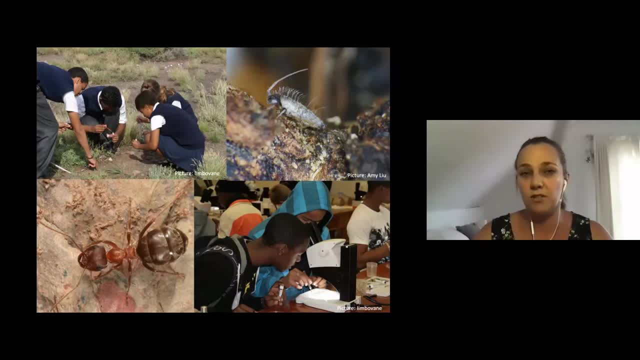 We also in our region have an increased research Interest and for conservation agriculture. So I really see this report as a great guide for landowners and farmers, as it highlights the research gaps and the threats, but, more importantly, it also provides solutions. So thank you very much. 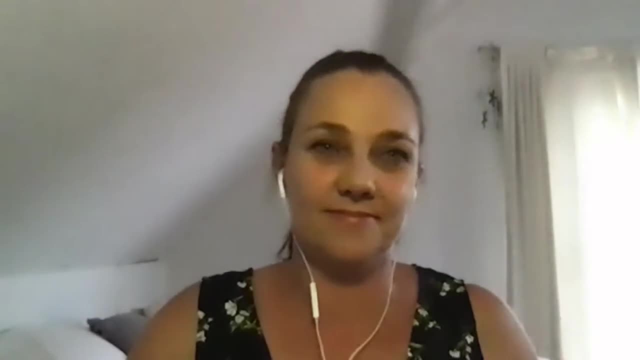 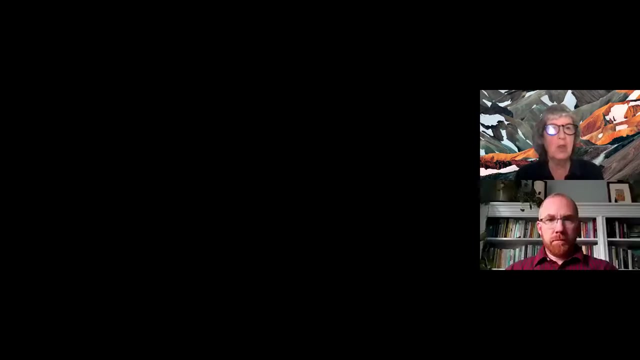 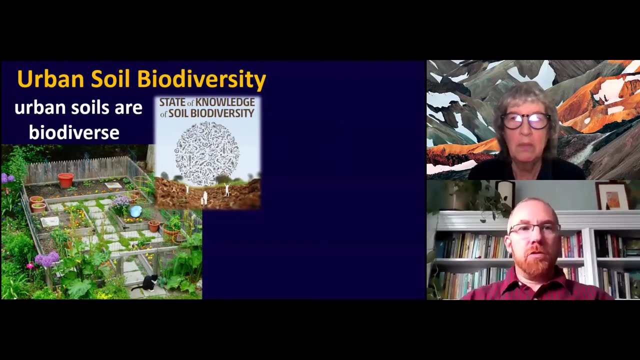 Thank you. So let's move on to our next panelist, who over to Dr Lauren Byrne, if you would Go ahead and present. Thank you very much. Yes, Hello everyone. So I actually contributed to the urbanization section in the report. 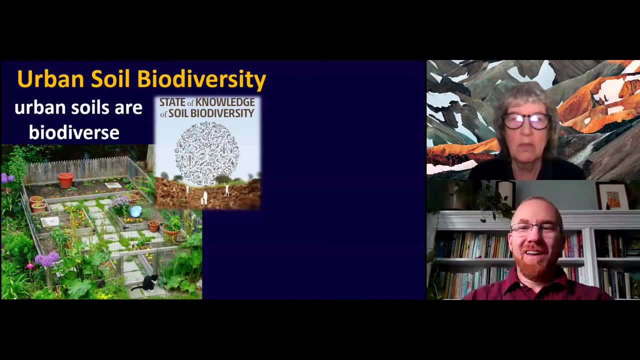 So urban soil biodiversity is my main research interests, And just a key takeaway from that is that urban soils are very biodiverse. Historically, there has not been a lot of attention given to the study of urban soils, But we know that there's a lot of things living in them. 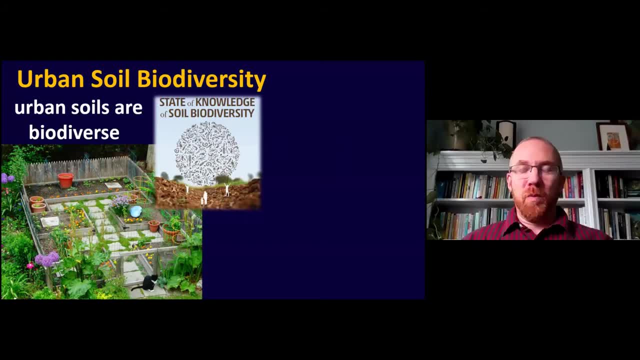 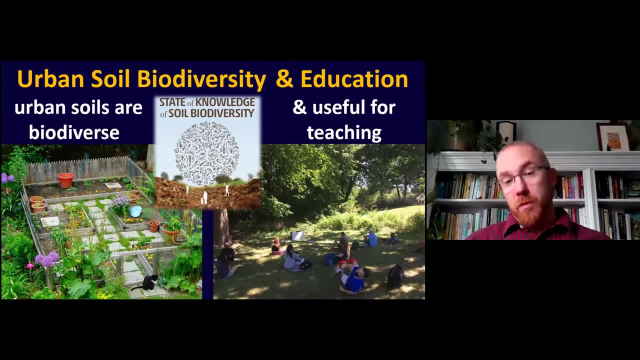 And that's very exciting, So I wanted to highlight That as part of this report. But, as Kate said during the introduction, I'm primarily an educator, So here I want to spend the rest of my time thinking about education and specifically how we can use urban soils as useful foci for teaching. 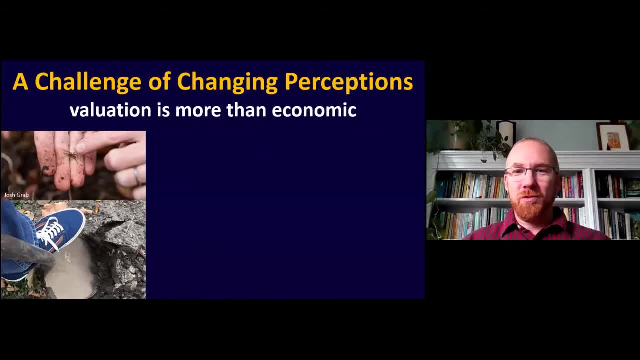 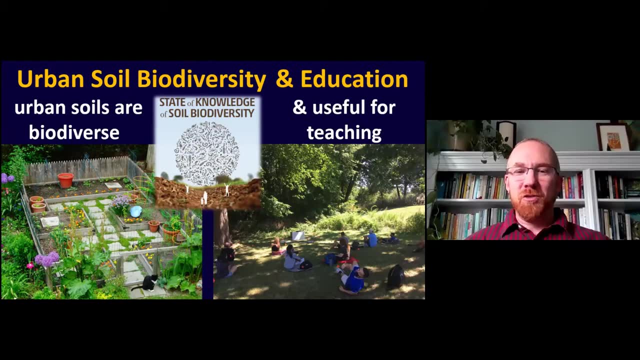 And here on the screen I'm showing my outdoor classroom that I used during the pandemic last fall when I taught soil ecology, And it's just a really great way to engage students by sitting out on the soils on campus looking at these soil biodiversity. 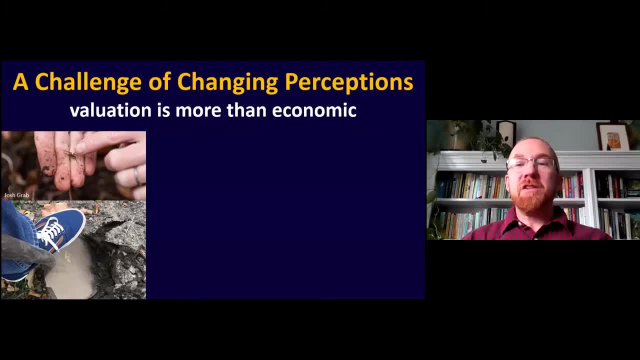 Wonderful things. That is a major challenge I think that we face. that comes out of this report is changing people's perceptions, and the report puts a lot of emphasis on ecosystem services as an economic valuation. But we need to think broader than that is one of my key messages today. 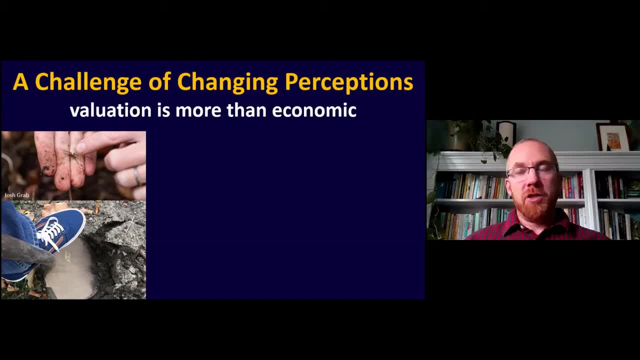 The valuation is much more than just economic And the changing perceptions I'm referring to are getting people to recognize the value of soils, that they're not just dirt. Things are getting soiled, have a negative connotation, bugs and germs, and we can dig in the soils and kind of just move them as we will. 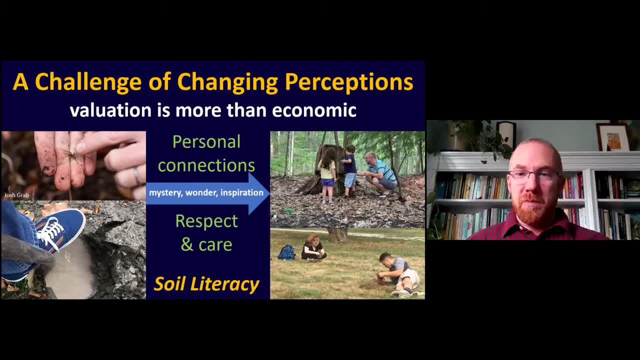 Rather, we need to make personal connections between people and soils, help inspire children through the senses of mystery and wonder of soil biodiversity So that they come to respect and care for it, And this might be considered a form of soil literacy. And I think this is a big challenge that we have as educators: to have people value soil. 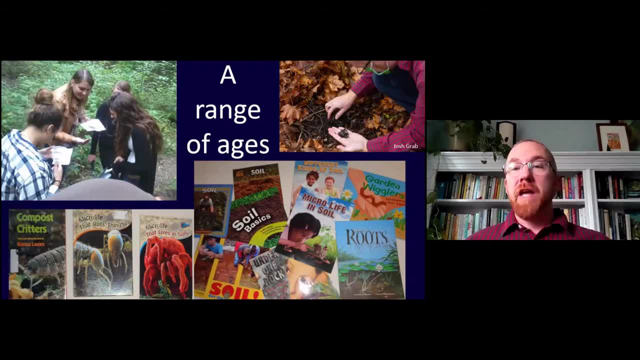 And it's not just children. I want to emphasize that we're thinking about a range of ages here, of course, higher education, college students, but also adults. I had an opportunity to walk with some senior citizens in my Local nature center and introduce them to soil biodiversity. 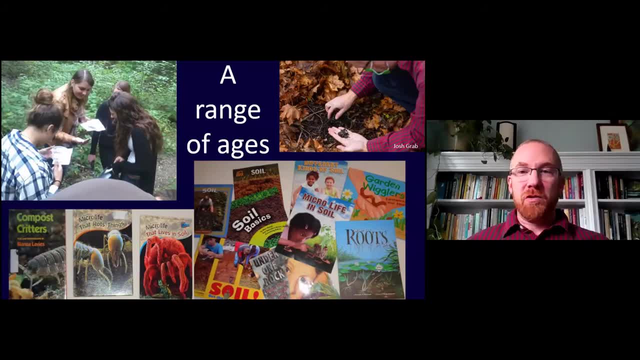 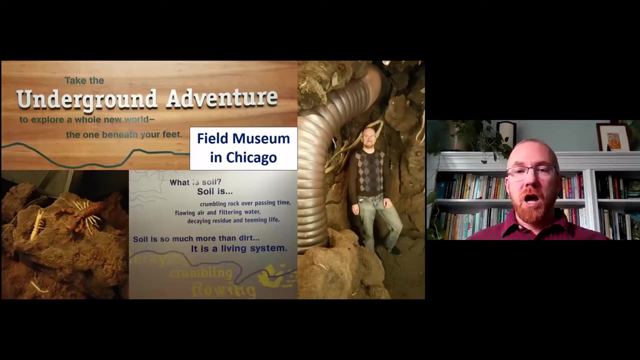 And here on the screen I'm also emphasizing, of course. there's lots of resources available to help introduce people, especially children, to soil biodiversity. The UN report itself can be used as an education tool. One really great resource is the Field Museum in Chicago. 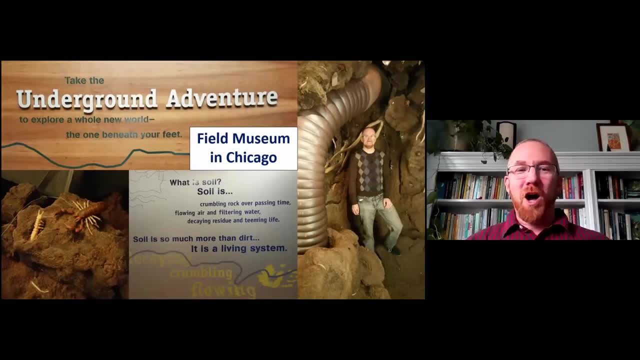 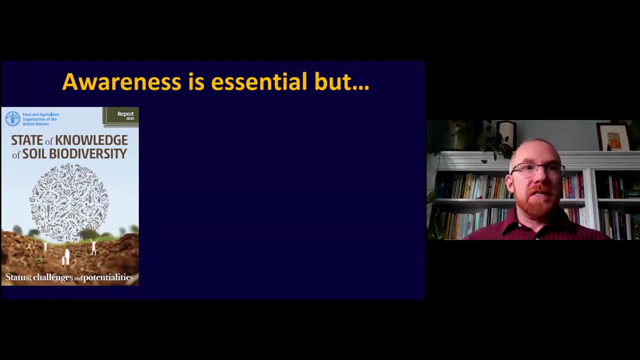 Introducing people to life underground by actually walking through. And you? The idea is that you shrink down to the size of soil organisms and learn about them. really fantastic If you're ever in that area to visit These resources. books, displays, the state of knowledge report are essential for promoting awareness, a word that's used a lot in the report, but I argue that it's not enough. 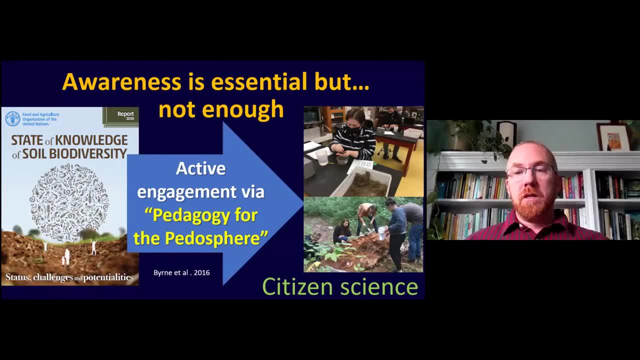 We really need to go beyond awareness through active engagement, working with students and people of all ages Via what I was some co authors have called pedagogy for the petosphere. This involves citizen science, as Charlene alluded to, and really hands on active 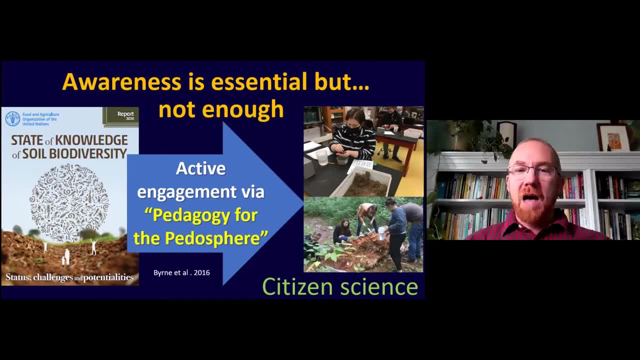 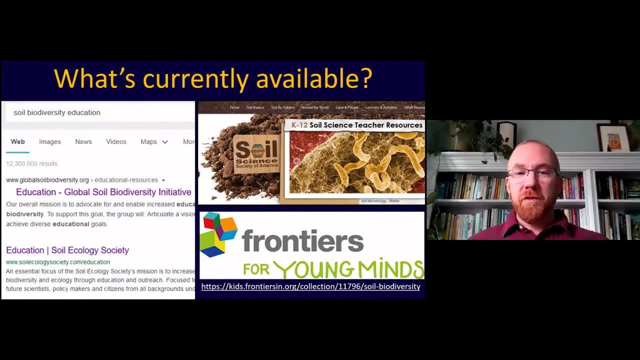 Showing people organisms in the soil, in the lab and in the field. How can we do this? There are lots of resources available online, Of course. if you're interested in a soil biodiversity education, search in Google brings up the top two results Are the global soil biodiversity initiative and the International Soil Ecological Society, both of which have education pages. 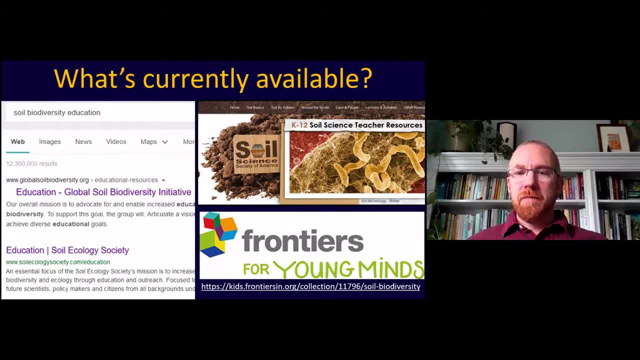 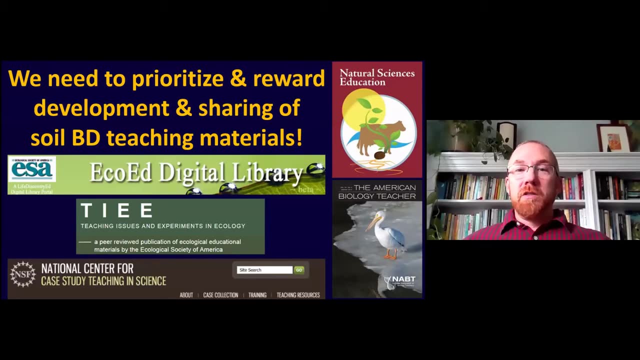 The Soil Science Society of America has a page with lots of resources And there's a really neat collection on frontiers for young minds. The link is there That has a lots of really cool articles. We also need to prioritize and reward development and sharing of soil, biodiversity, teaching and materials. 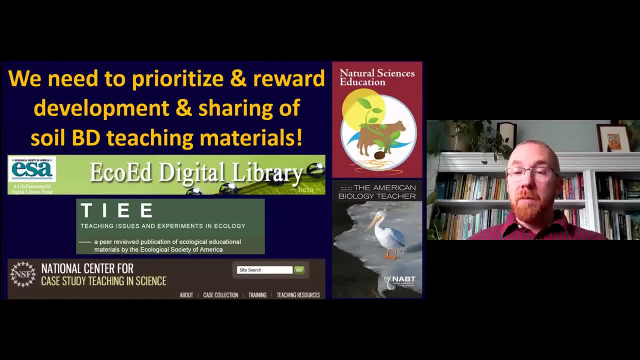 Within our scientific communities. There are lots of places to publish peer reviewed articles about teaching Actual lessons resources. How can we better create a community that does this and that will ultimately help be helpful for ensuring that teachers have resources available to be able to do this? 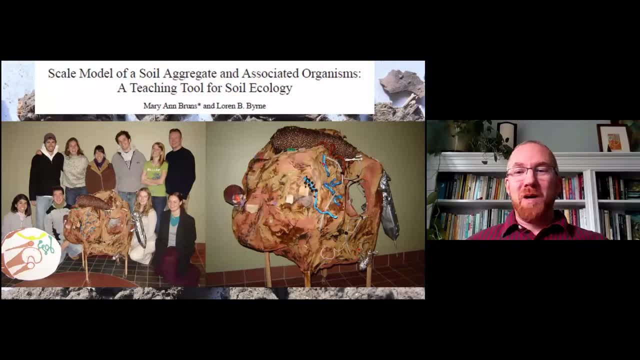 For example, I, with my PhD advisor, Marianne Bruns, published an article In which we Described how to build a soil aggregate model with organisms on it as a teaching tool. larger than life size, of course. aggregate that can really get people engaged in thinking about what is going on in the soil. 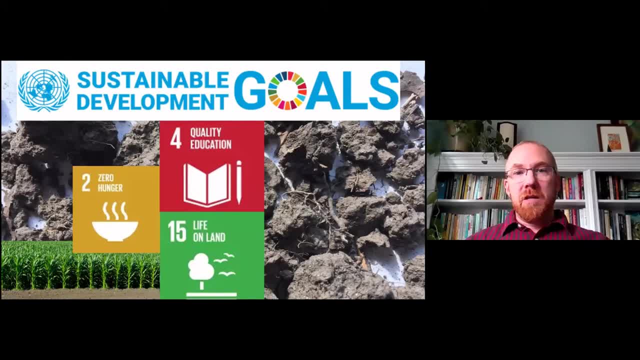 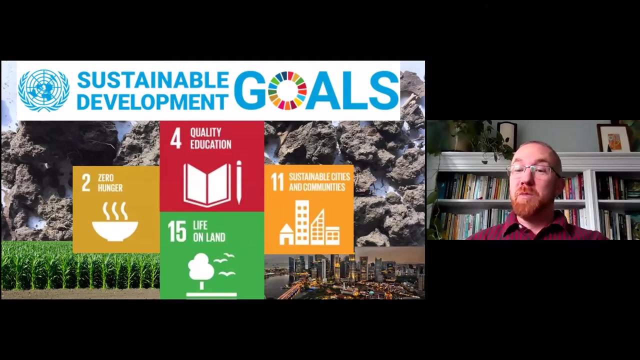 And to conclude, I'll bring it to the sustainable development goals, which highlights quality, education and in terms of soil, biodiversity, that's connected to life on land and probably Most people, and somewhat in the report emphasize food production, promoting zero hunger through sustainable agriculture. But my conclusion is that we really need to include sustainable cities and communities, which is also a sustainable development goal. 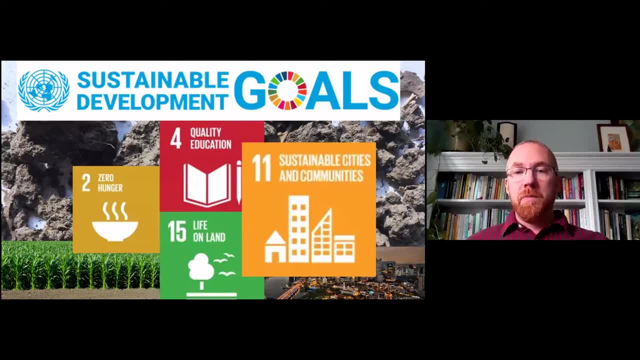 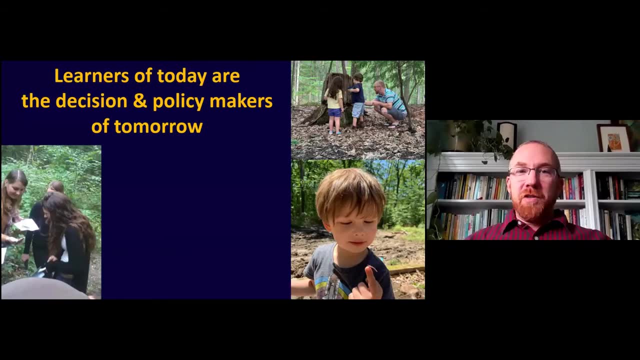 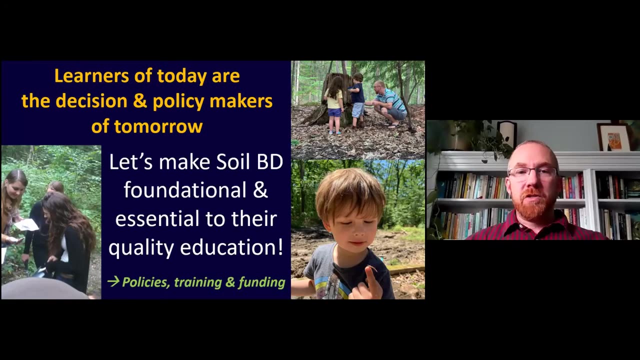 And probably for education. We're going to be able to reach a lot more people if we think about urban soils as a place for quality education. The learners of today are the decision and policymakers of tomorrow, So we really need to forefront and emphasize the need for increased soil biodiversity. 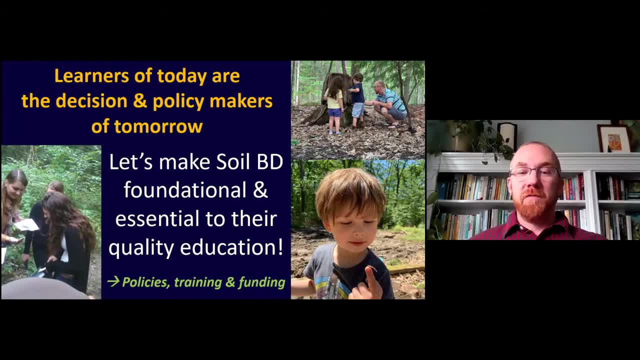 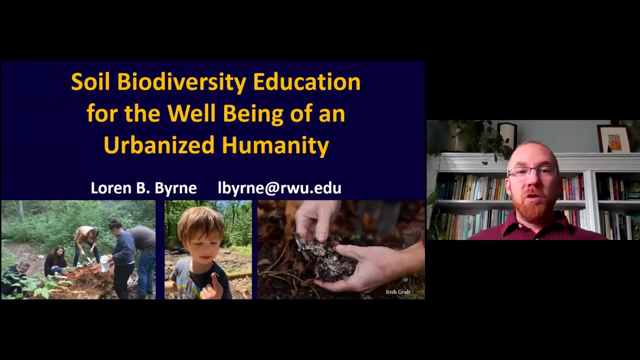 Let's make it foundational and essential to the quality education of People all around the world through policies, training of teachers And of course, we need some funding to be able to do all this really well. So my last point is my title. I put at the end, just as a final message: soil, biodiversity education for the well being of an urbanized humanity. 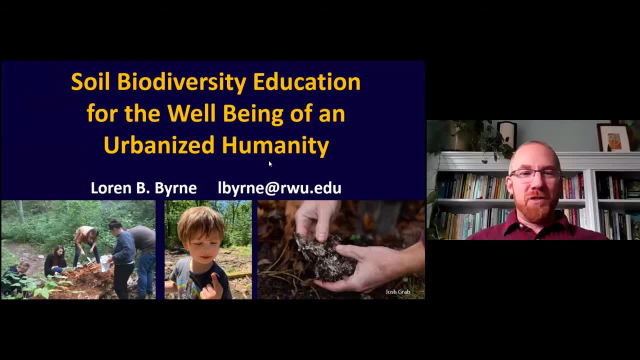 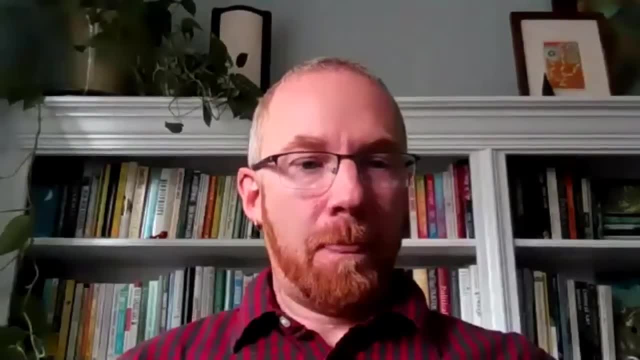 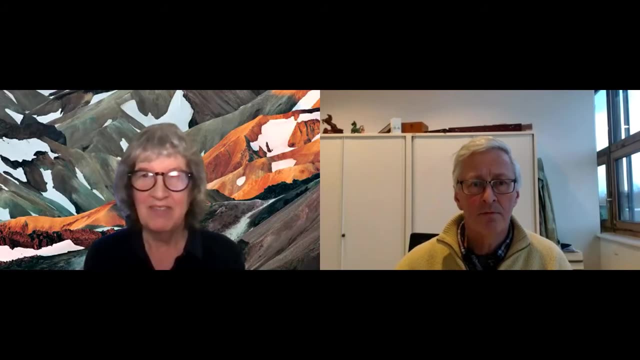 And I'd be happy to hear from anybody. There's my email address to share any of those resources specifically: Thanks, Thank you very much, Lauren. Okay, thank you. So when? what do you have to say? Well, thank you, Kate, And it's pretty that to link, she seems, seems to be blocked, but 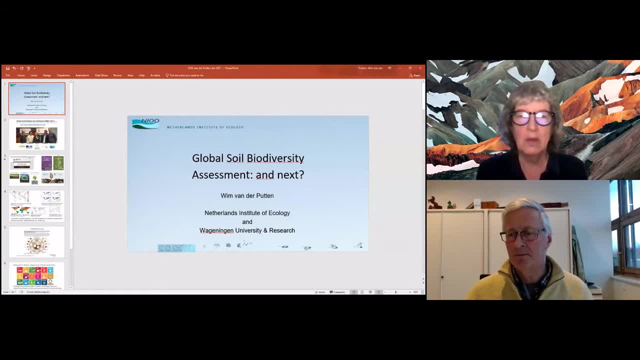 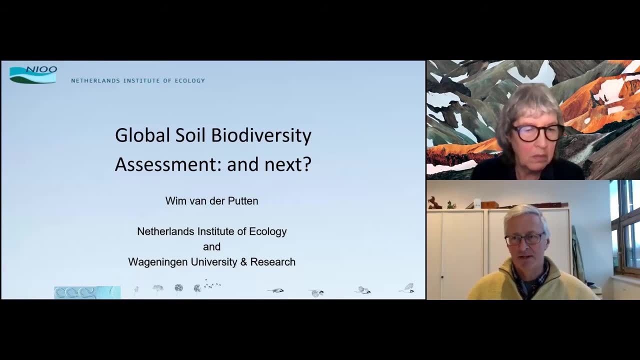 Monica's working on that. Okay, So Well. actually, the idea was that I was the last Question to give an introduction and I wanted to step back and step forward a little bit. Actually, I've been involved with dueling in chapter five, but I also was involved in sort of the overall editing of the report. 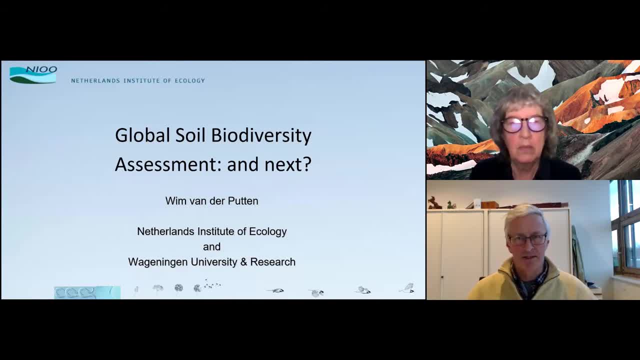 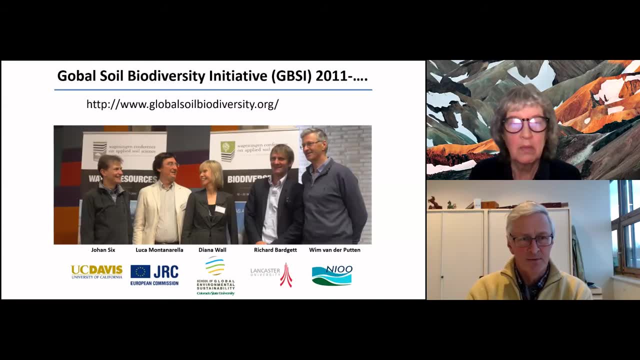 But actually my involvement started already much earlier, in 2011.. So I want to go back to that year. And then, during a meeting in Wageningen, during the first Wageningen Soil Conference, this group of people was coming together in my room, which was just opposite the road of the conference building. 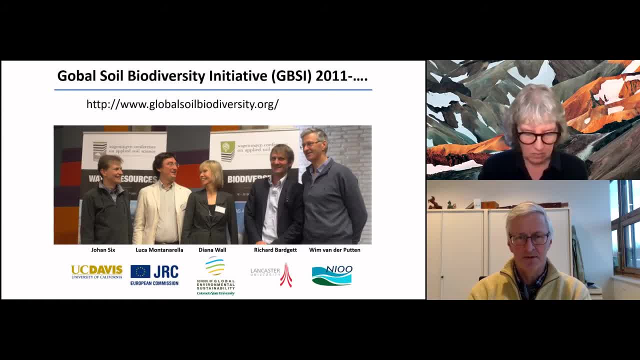 And we were sitting together and thought we should do something. It was a lot of non-soil biodiversity in the conference And while there was a lot of progress being made on soil biodiversity and soil ecology And we said we have to do something to bring this under the attention of a wider audience. 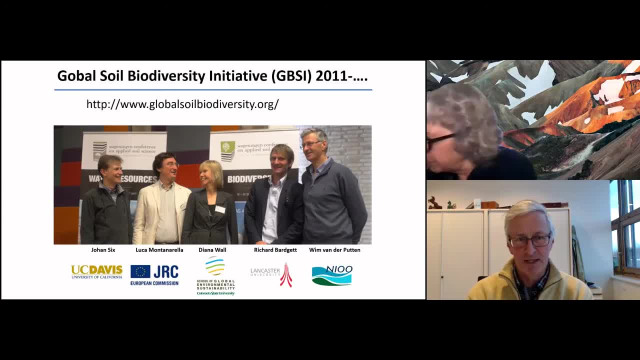 So, with a bang of the fist of Diana on my round table here in my room, the GSBI was established, and then we said, okay, what are we going to do? So the first thing that was done is to set up a website. 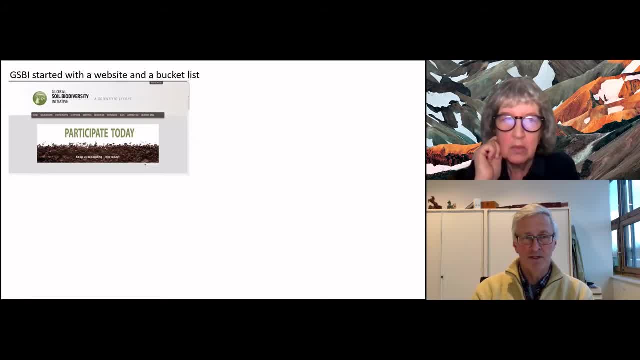 And if you have a website and a good message, you're quite powerful these days. So Diana was invited by the CBD to speak, and by many other at many other occasions And in 2012, we were asked: what is on your list? 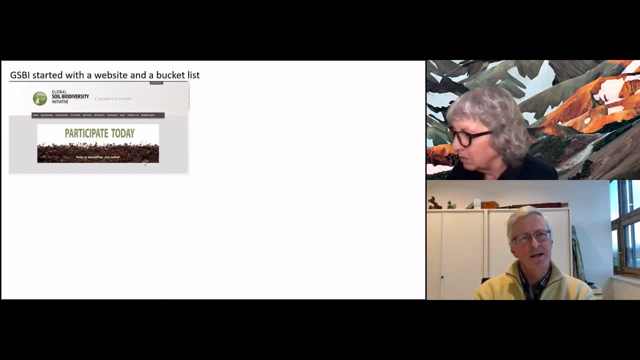 So actually now we're looking back at it. I think we then formulated a bucket list, and not that we were thinking of dying afterwards, but actually we just formulated a list of things that we wanted to do, And it's amazing that now, within 10 years later, that we are able to say we just did the whole list. 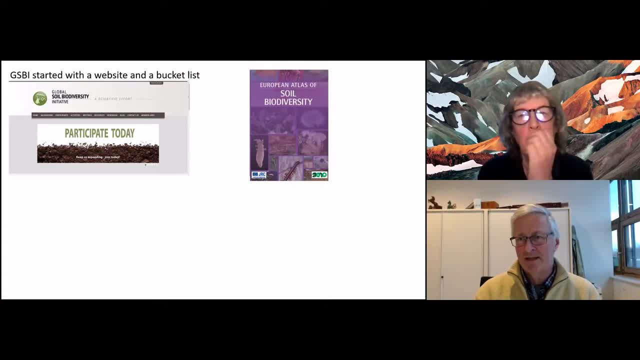 So we thought about doing atlases on soil biodiversity. So a European atlas was produced and a global soil biodiversity atlas was produced. And we couldn't do this alone, of course, So we were receiving a lot of help from the Joint Research Center. 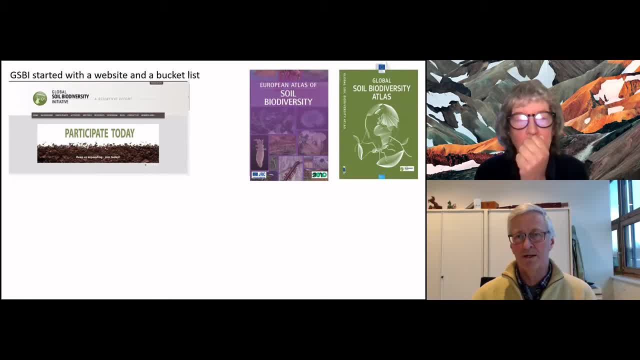 That was very experienced in making atlases of all kinds of issues related to soils And the GSBI brought together all the experts worldwide and that together helped us to produce these atlases. Then we said we have to reach out to our peers. 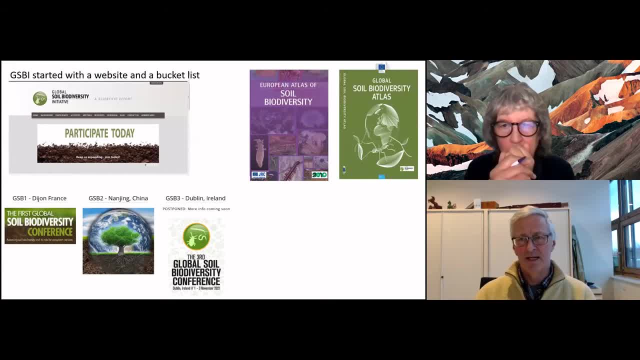 So we need conferences. So that's what happened. So there was a Global Soil Biodiversity Conference, The first one in Dijon in France, organized by Philippe de Monceau. The next one was in Nanjing in China. That was a huge conference. 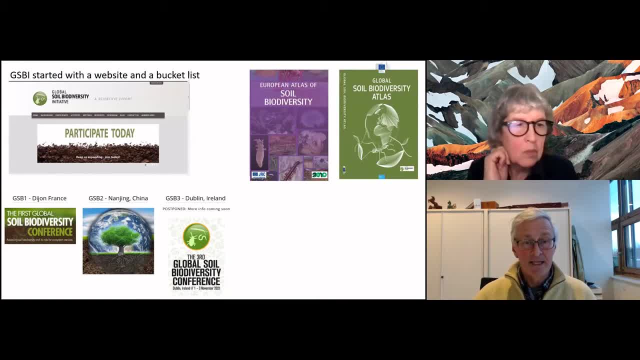 Many, many Chinese people were there, And the next one is going to be organized in Dublin as soon as COVID allows. And then we said: okay, we also should start producing a Global Soil Biodiversity Assessment And luckily the United Nations picked this up and asked the FAO. 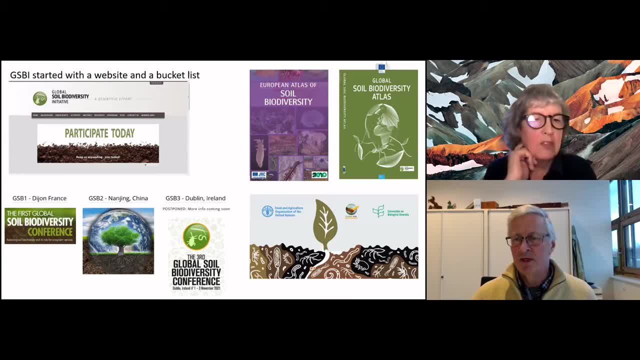 the Food and Agriculture Organization of the United Nations to start producing this Global Soil Biodiversity Assessment, And the Global Soil Partnership, the IDPS- all the organizations that Diana mentioned in her introduction. they all contributed to producing this great first Global Soil Biodiversity Assessment. 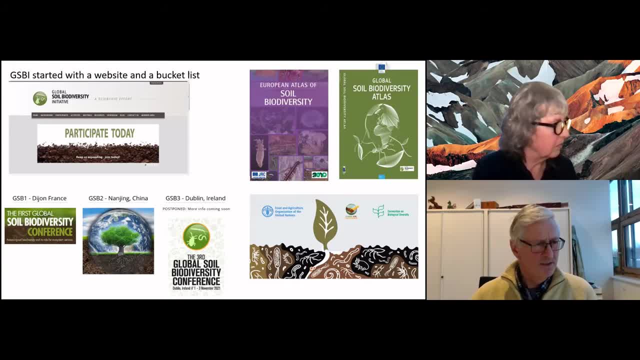 that was released December 4, 2020.. So actually, if I look back, we just did the whole bucket list. So is it time to die or to go on? Certainly it's not time to die. There's still too much to do. 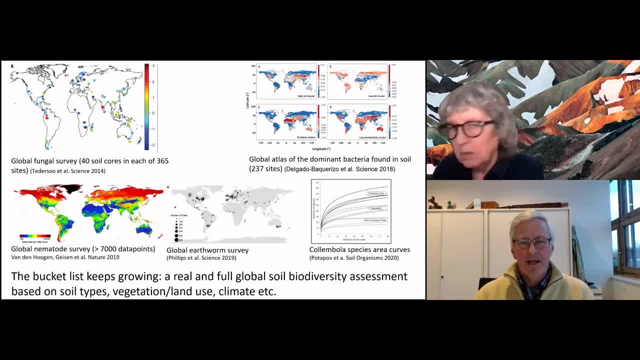 So the bucket list keeps growing And actually over the past years we have seen many very interesting papers on assessing various aspects of soil biodiversity worldwide. So we have a nice study pulled by Leo Tedesau on Global Fungal Survey. There's a nice study by Manuel de Gado and colleagues. 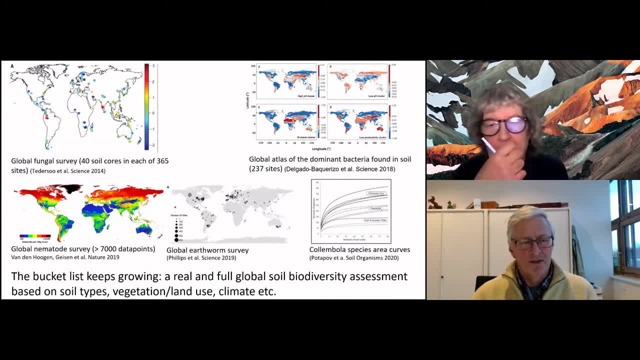 on dominant bacteria: worldwide. Interesting paper by Johan van der Hoogh and Stefan Geissen. on nematodes, There's a study pulled by Helen Phillips, which is the Global Earthworm Survey, And then there is a study on Glamland species by Podapov and colleagues. 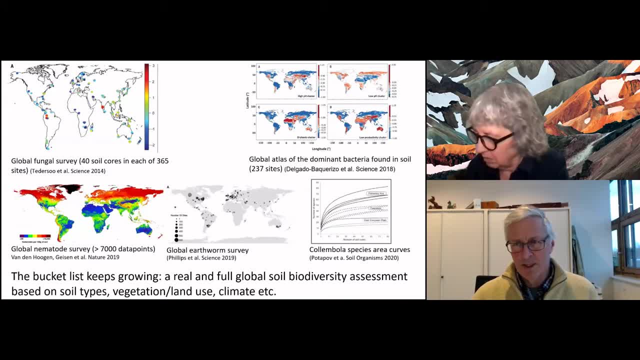 And there are other studies as well. So what's the intriguing thing Of these studies? I'll mention two. One: if you look at the top left panel, you see Africa, and then you see two, four, five sampling points, maybe six sampling points in Africa. 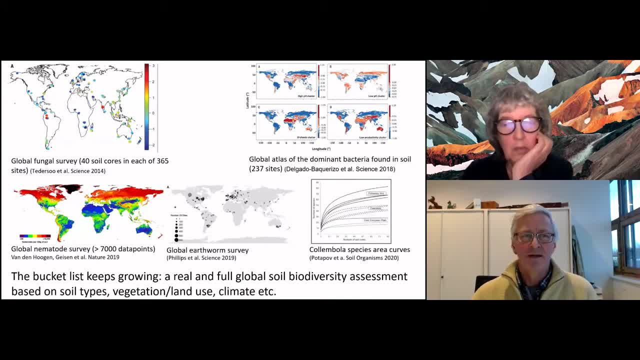 Six sampling points in a whole continent that just varies from desert to tropical rainforest, So this is not enough to cover a whole continent. The other thing that is striking is that there is a lot of research going on. If you look at all these different studies. 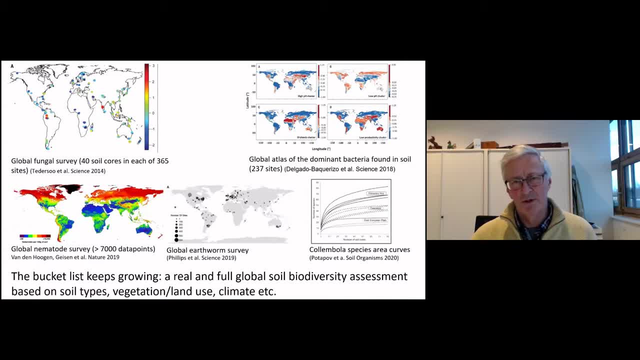 is that each study focuses on one species group or one taxonomic group, So fungi, bacteria, nematodes, earthworms. So I think a real challenge for us in the years to come is to look at soil biodiversity in conjunction. So we should go out and take a spade or a core or whatever and then collect soil samples. 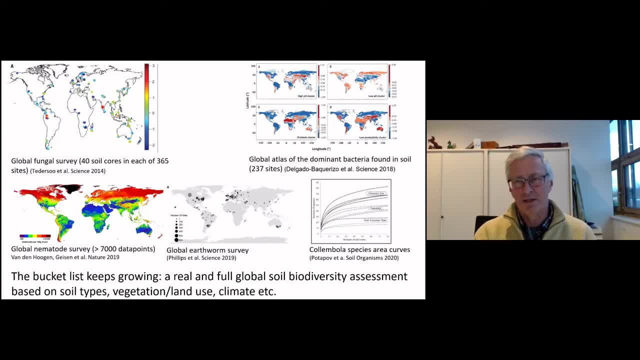 but just take out everything that is there, So not only the bacteria or only the fungi or only the nematodes, but everything. And then look at how these organisms are interacting with each other and how that interaction depends on land use, on climate conditions, on vegetation type, and so on, and so on. 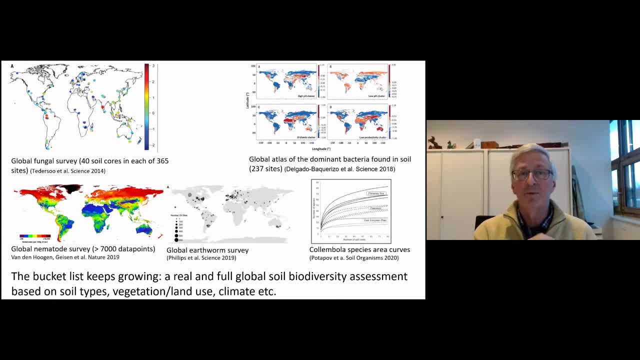 And then look at the functional consequences of these community compositions And, ultimately, what we need to do is to reach out to people who manage the land, who own the land, and then show what the use of the land is doing and how that is affecting soil biodiversity, but also its functioning. 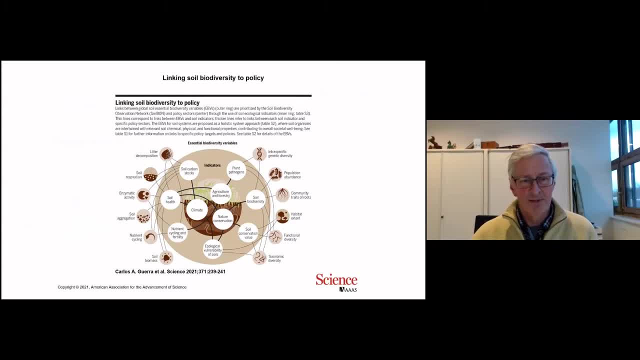 And then we have to reach out to policy And there's a very nice paper that appeared in Science a week ago, pulled by Carlos Guerra, And that makes a plea to link soil biodiversity to policy. And that's really important because many policymakers are very unaware. 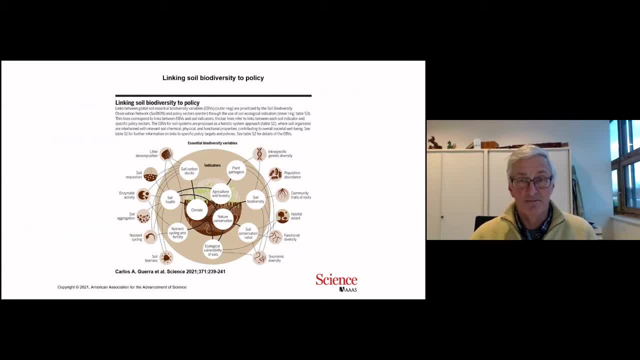 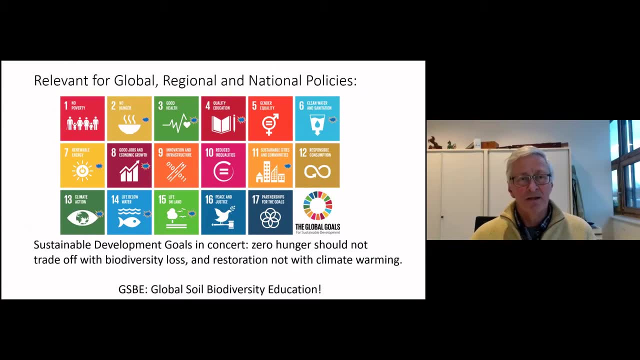 of what's going on in the soil underneath their feet. So this is a very important next step to be made. And then Lauren already mentioned the Sustainable Development Goals. I've put in blue dots where I think that the Sustainable Development Goals are affected by soils and soil biodiversity. 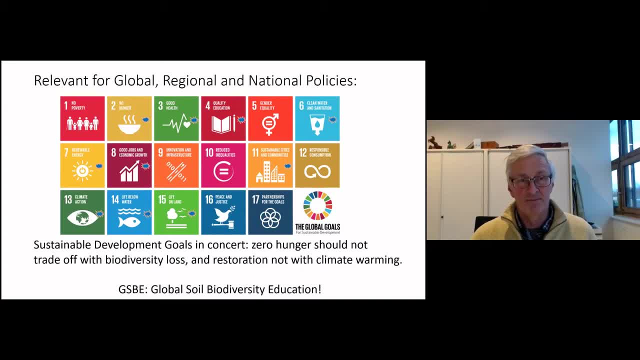 No hunger. It all comes down to soil biodiversity. But one striking thing in the Sustainable Development Goals is that people tend to focus on each goal individually. So I don't know hunger or climate action, And the thing that we are experiencing more and more is that one. 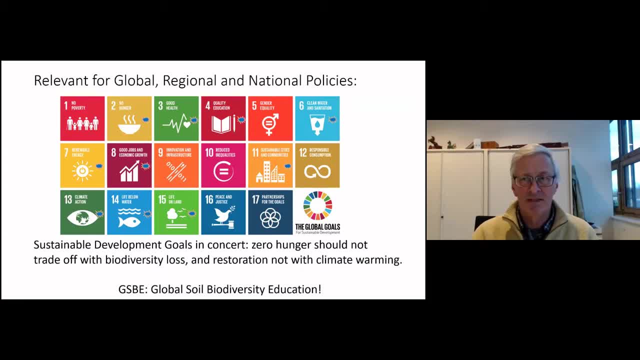 solving one goal can go at the expense of another goal. To give an example, if we solve the hunger issue worldwide, then, for example, making soils highly productive, then that high productivity can go at the expense of soil biodiversity. This is what has been established for a number of sites worldwide. 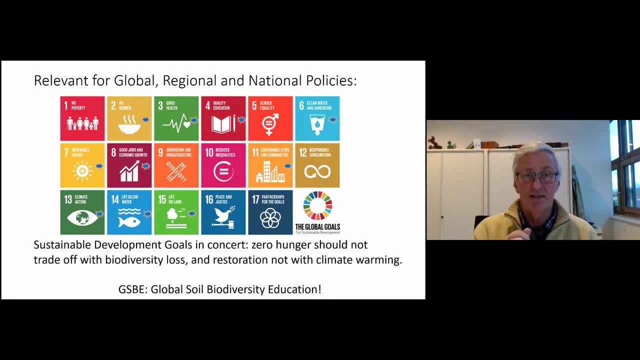 And if it goes at the expense of soil biodiversity, it goes at the expense of soil multifunctionality. So this is actually a paradox, because the paradox is that we can have highly productive soils in terms of food production, but that are producing very little. 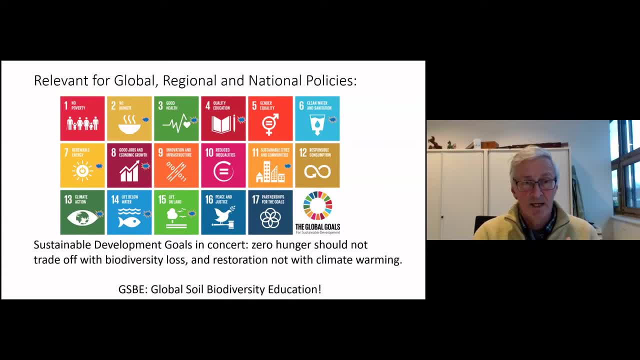 or very few other ecosystem services on which we also depend. So we should look at win-wins instead of trade-offs, And I think this is a crucial and a very important goal for the years to come And also in support of Lauren. 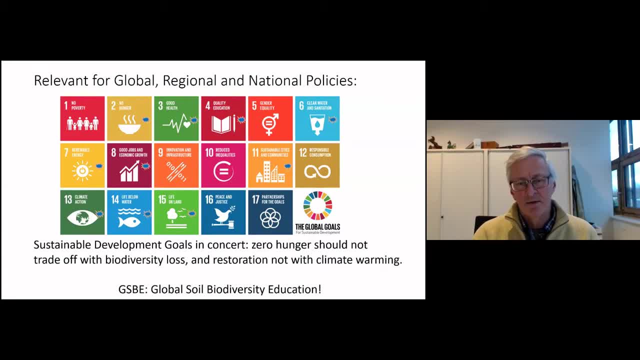 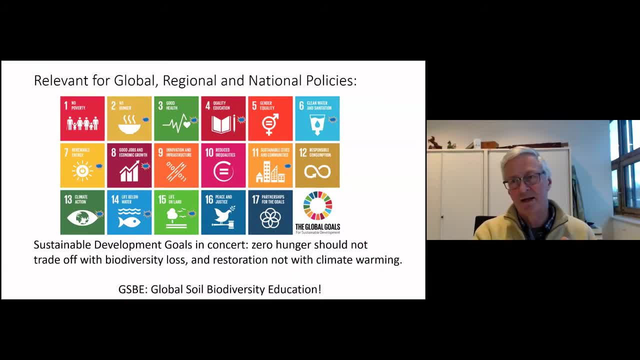 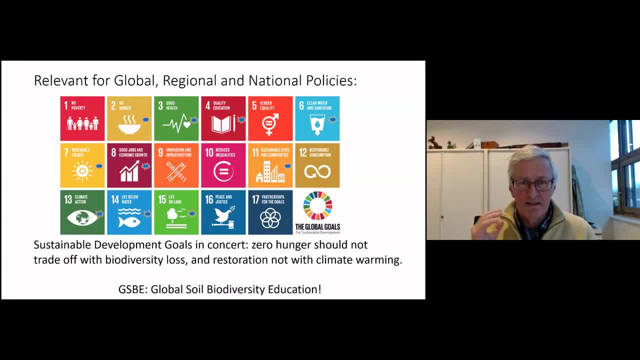 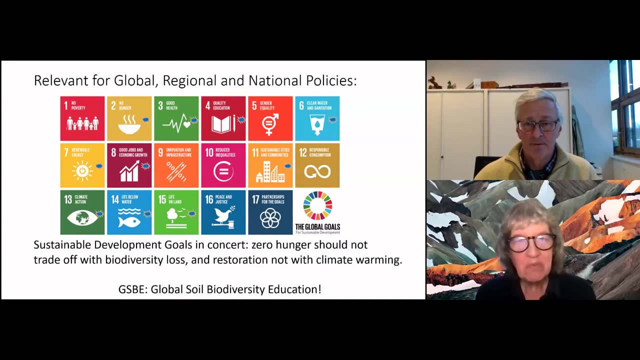 So my point that I would like to make is: let's keep on going, Let's make a new bucket list And let's go for soil, biodiversity and make it work. So, Kate, this is my contribution. Okay, Thank you very much, Wim. 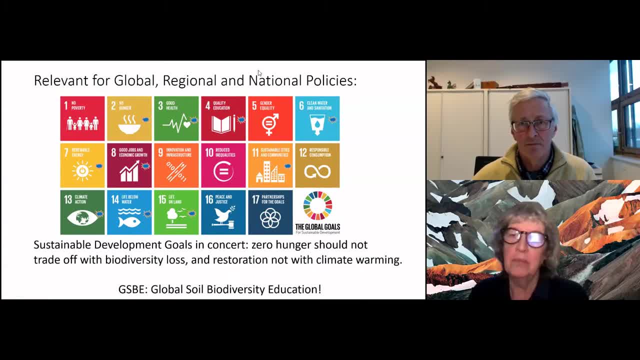 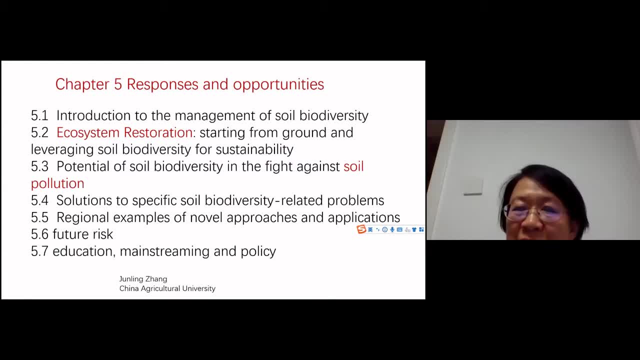 And so we're fortunate to have Dr Junling Zhang back. Okay, Hello, Thanks, Kate. Hello everyone. Sorry, just jump off. So this is Junling here from Beijing. I'm glad to be here in this webinar to share with you all for Chapter 5.. 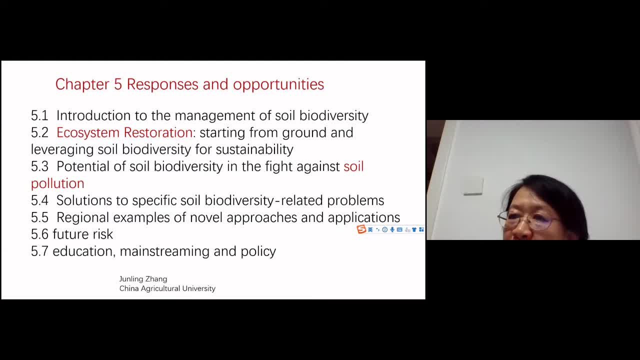 First of all, many thanks for other contributors or collaborators for your hard work, And now it's really in good shape. Chapter 5 is Response and Opportunities, And here we have several sections: Introduction: Ecosystem Restoration, Potential of Soil Barrier, Devastation in Relation to Soil Pollution. 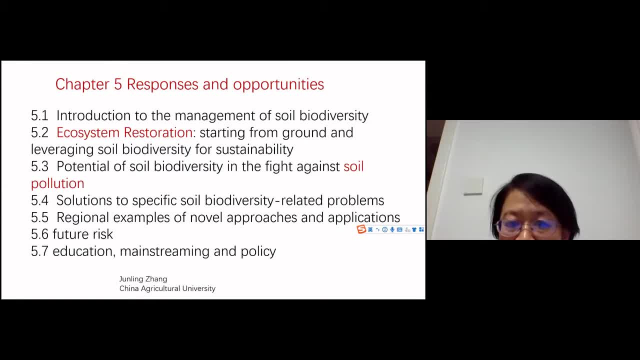 And then it's a solution and the original examples of novel approach in the evidence And future risk education, mainstreaming and policy. So we are asked to talk why we are interested in contributing to this chapter. I think for me this is because there is increasing recognition of the need to enhance soil-based 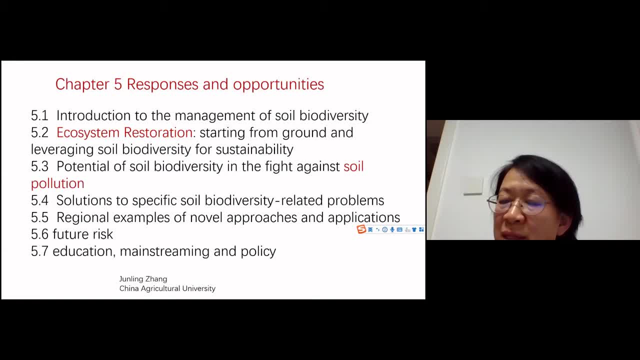 multi ecosystem services other than merely production driven service provision. So I'm here from Agriculture University here in China and the main task here is to maintain food security And nowadays, particularly this year, this coming past year- secure global food security and promoting healthy foods brings unprecedented challenges for the limited cultural land. 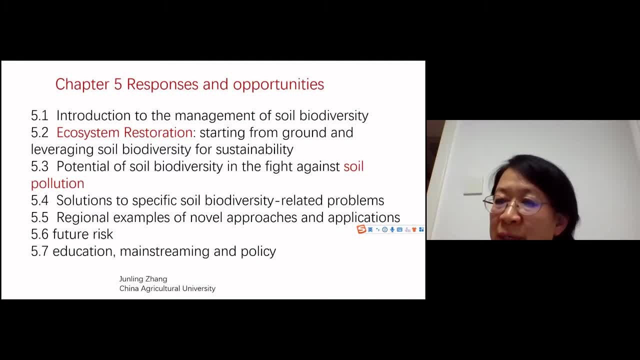 So this is particularly more evident in China, because here agricultural systems feed 20% of the world population. So agriculture in China has achieved enormous successes. However, conventional agriculture come along with the deleterious effect of environments such as soil acidification, So it is erosion, et cetera. 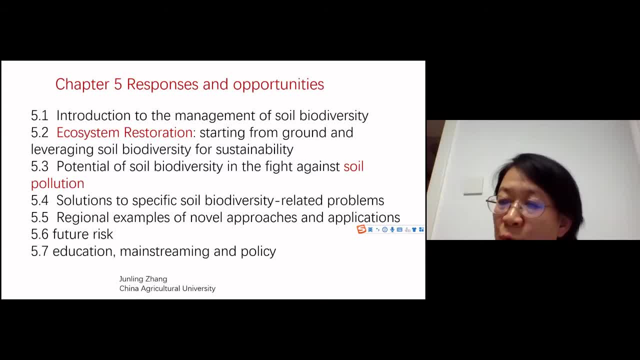 Therefore, there is an urgent need for transformation of present-day intensive agriculture, following a path that is being called, in China, agriculture, green Development, That is, AGD. So AGD was proposed as a national strategy of sustainable development, pursuing green development. 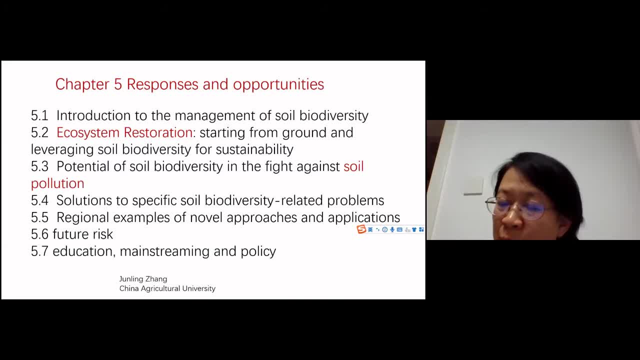 intending to contribute to the achievement of the world's sustainable developer goals. The core of AGD is to reduce excessive use of external inputs and promoting the internal regulatory and regenerative process of soil. This is a key component for this process. For this, I want to give two examples. 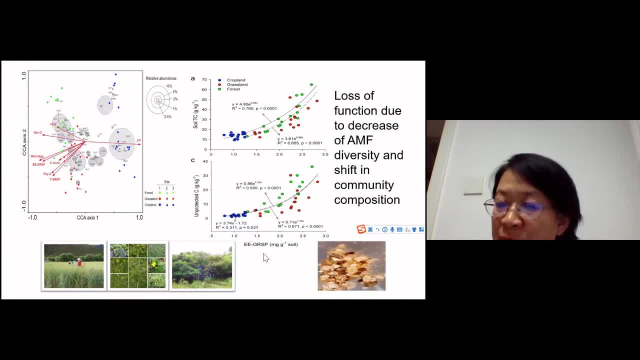 So here I would like to have. this example is from Tibet, a plateau where agricultural practices are still underdeveloped, developed. So we compare the the biodiversity among agricultural soil, cropland, grassland and forests. So here is soil carbon and is unprotected carbon. 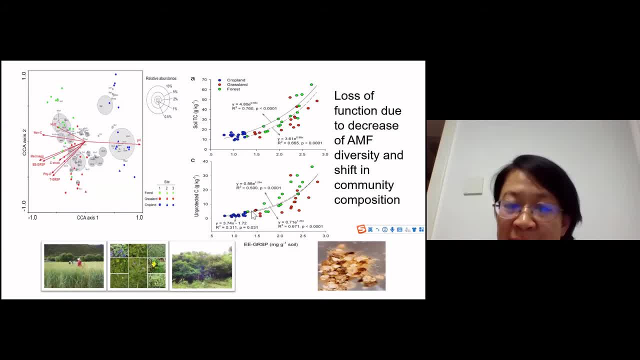 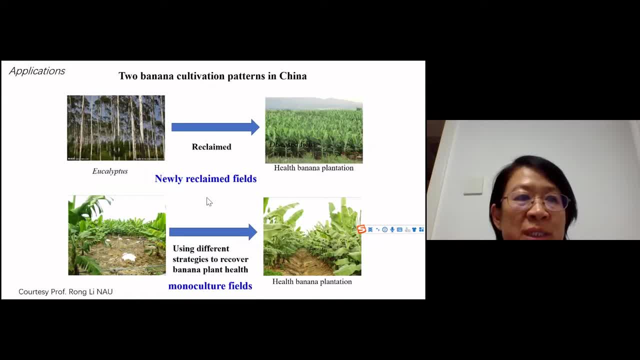 And the other example I want to share with you is the application part. So this is the experiment conducted by Professor Li Rong, who is from South China Nanjing Agricultural University, where they have been working in Hainan for many years. What they did is that they manipulate soil. 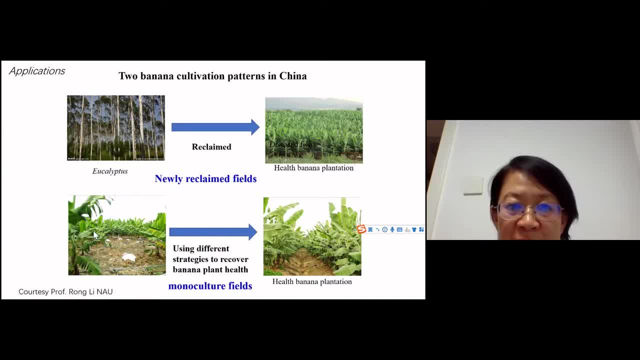 microbiome in banana fields. This is a newly reclaimed field and this is monocultured fields. So in these two kind of situations, different strategies are used, but the core is to inoculate effective biochemicals. So how can we use bio fertilizers to produce healthy banana plantations? 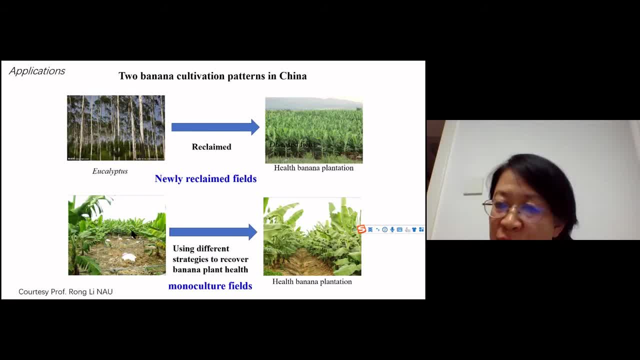 Therefore, from those examples, the take-home message is that there are great opportunities to enhance and maintain the biodiversity of soils for sustainable development in those unhealthy or diseased soils Management that increase soil biodiversity and take account of the composition, traits and function of soil. 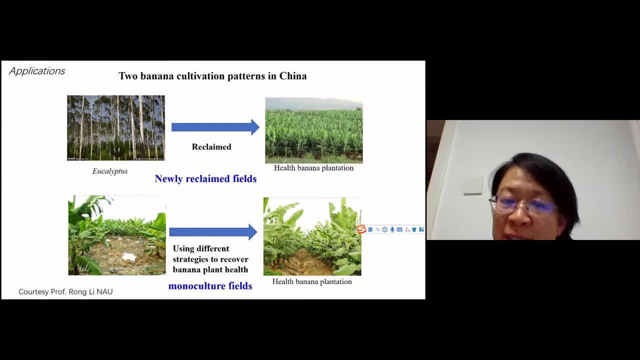 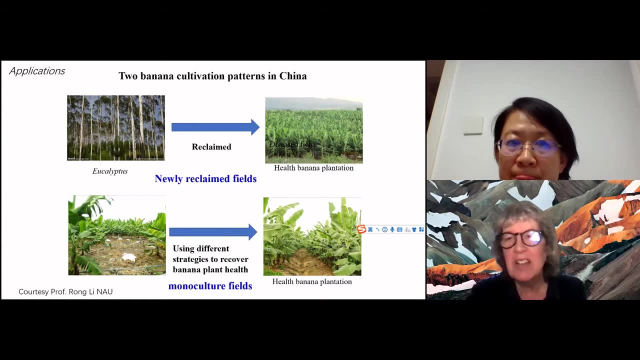 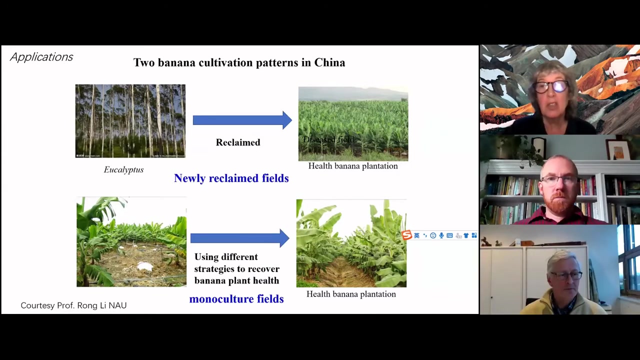 So this is an example of how we can use bio fertilizers to create healthy organic organisms, as well as ecological internet interactions, essential for creating, maintaining healthy soils for sustainable development. Yeah, that's it, Thanks, Great. thank you very much. So now can I ask all the panelists to turn on their cameras. 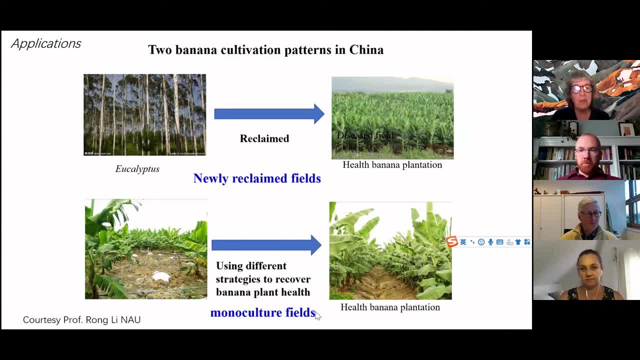 and we're going to start the Q&A section. So we have a number of questions pouring in. Thank you, audience, You're really proactive and some great questions here. And just to remind you, put the questions into the Q&A box and we will try. 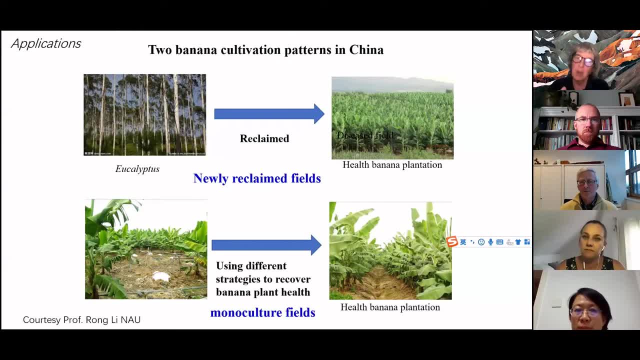 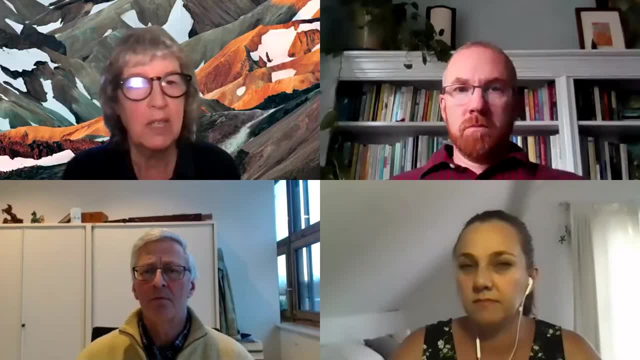 to answer as many questions as possible, but I'm just warning you that there may be more questions and there's time to answer them, but we'll do our very best. Apologize if we don't get to yours. So first of all, there's a question for Lauren. 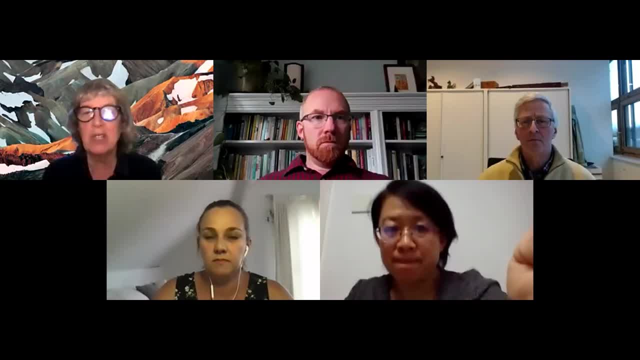 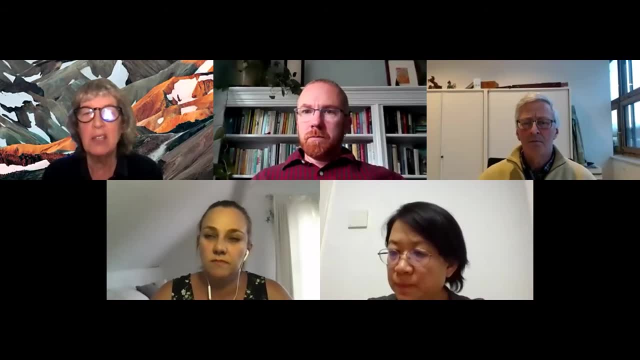 The idea of increasing literacy around soils and biodiversity is critical to increase a willingness to protect and preserve soil organisms. How do you see this having a spillover effect to politicians and conservation managers that often make these decisions or may be blind to the consequences of their actions on soils? How do we develop? 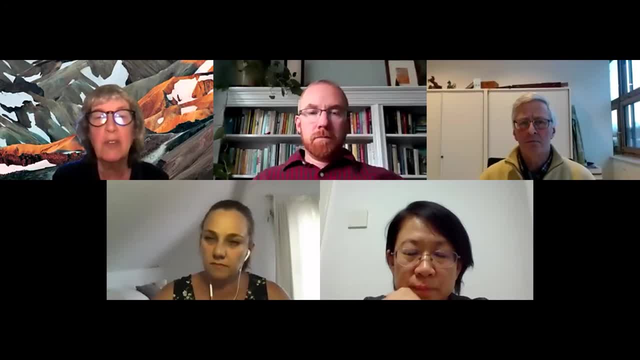 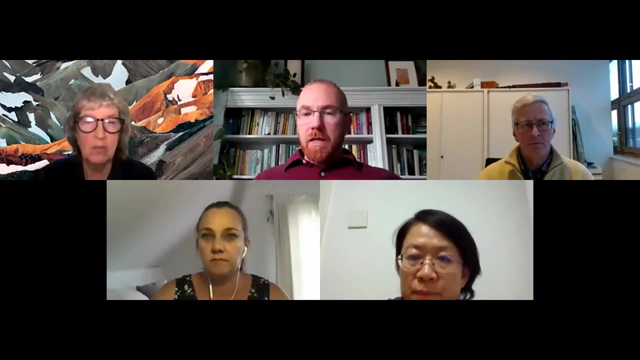 a strategy to accelerate this, And this is a question from Carlos Guerra. Yes, thank you, Carlos. Yeah, it's a very multi-dimensional issue. One of the key points I think I'll re-emphasize from my last slide was that we have to keep in mind that the students of today, the, the children, 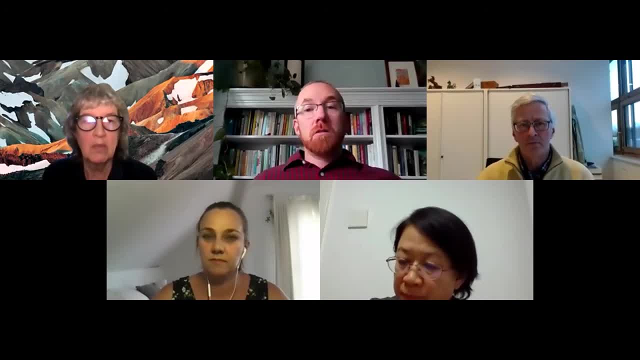 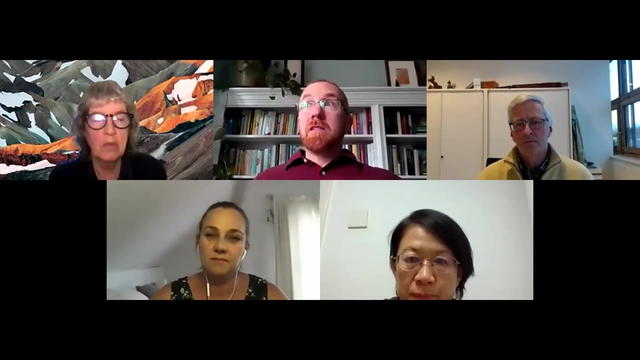 are going to be the future policy makers. So certainly that's a long-term strategy that is needed to promote soil literacy in children of today so that they carry that forward with them in their future careers. Assumedly, someday, Assumedly, some will become policy decision makers, But that's probably too long-term right. 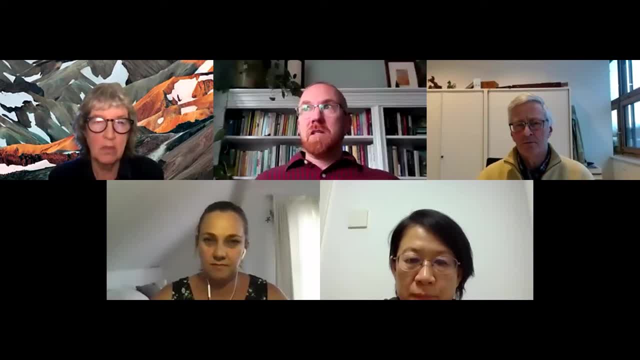 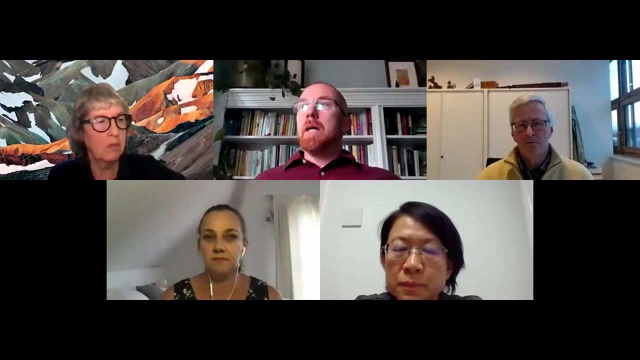 We need some short-term solutions because the problems we're facing with soil management and sustainability are today, So we need to engage directly with policy makers of today. of course I have limited personal experience doing that, but you know it's a natural extension of what we do in. 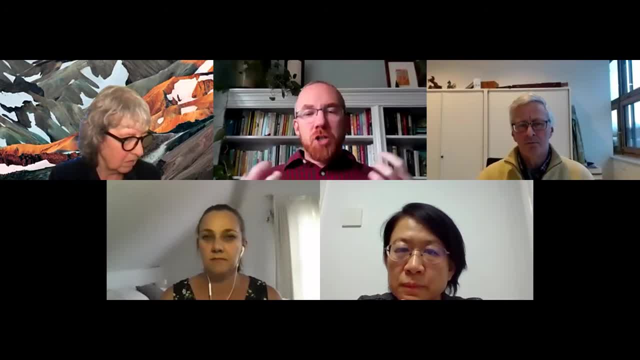 the classroom. I think It's something I'll be doing in the future as well. I'm not going to do much. How can we show them with concrete- or I shouldn't say concrete- with physical soils right and physical organisms in front of them? Can we take columbulin cultures, earthworm? 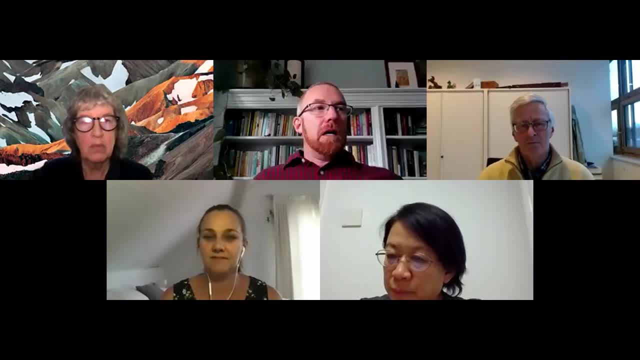 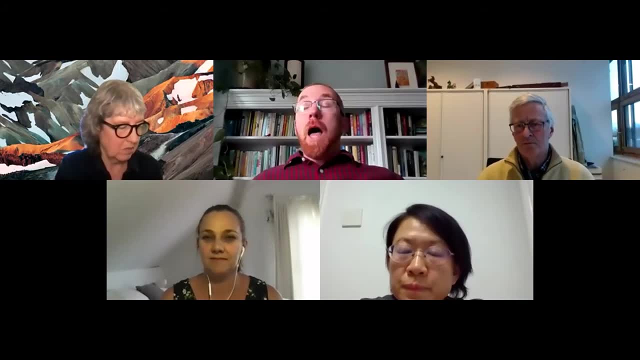 cultures into their offices. That, hopefully, will open their minds to the possibilities. I think a top-down strategy that's really important is using reports like from the UN to say: look, this is a global issue. And then, from the bottom up, we as individual community. 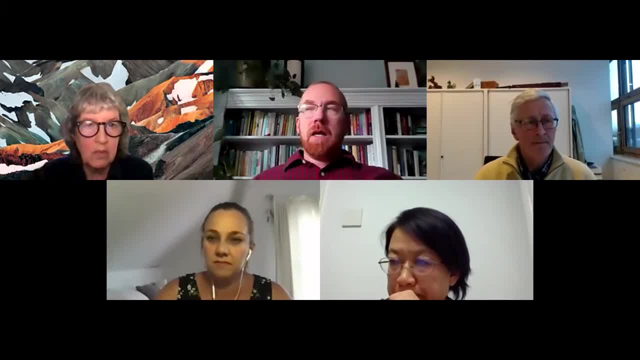 members have to bring it to their attention and say, look, this is the global report And as you're one of your constituents, I'm a scientist and go in front of them. Just a quick little anecdote that I was thinking. when I saw your question. Jane Lubchenco is a famous marine ecologist in the United States, probably globally among marine ecologists- And Kate's comments to begin about why people love marines. so much is apparent when we think about what Jane Lubchenco did with the United States. 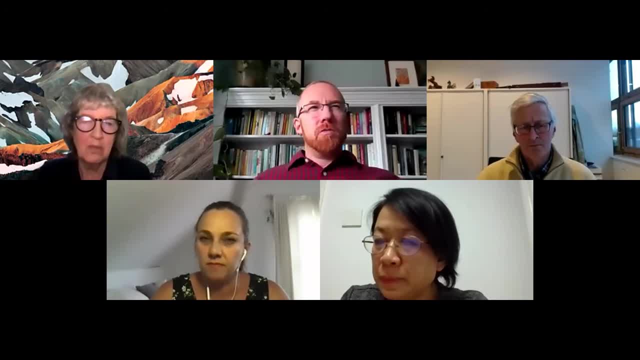 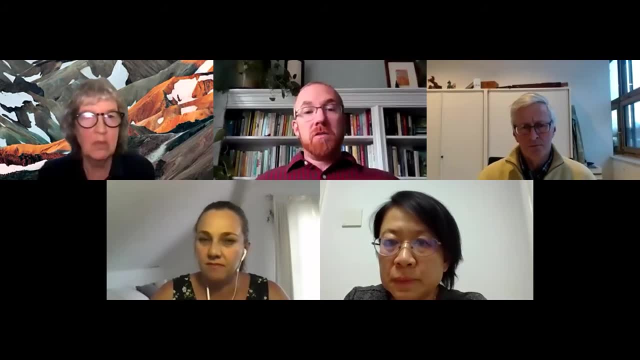 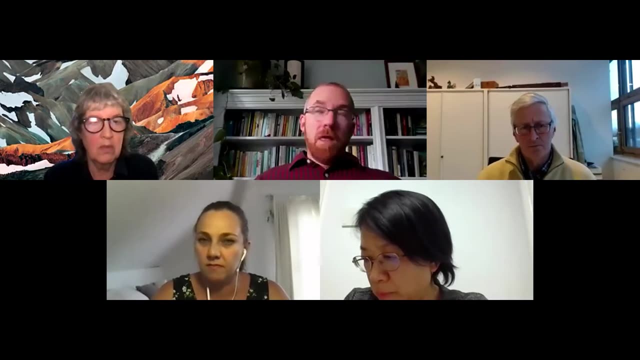 government. She served in a role, I think she was the chief of the NOAA, But anyway, the key is that she was able to have an audience with Congress leaders in Washington and she had a demonstration for them with ocean acidification And very simply had some beakers. 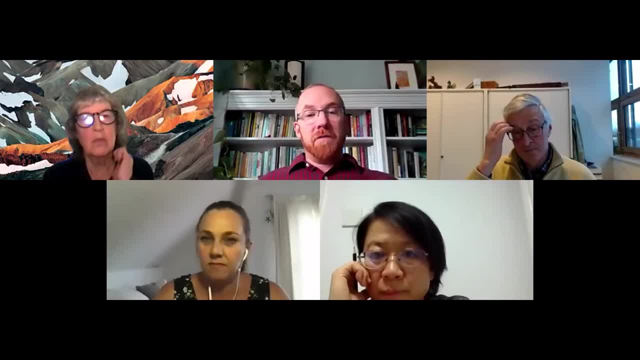 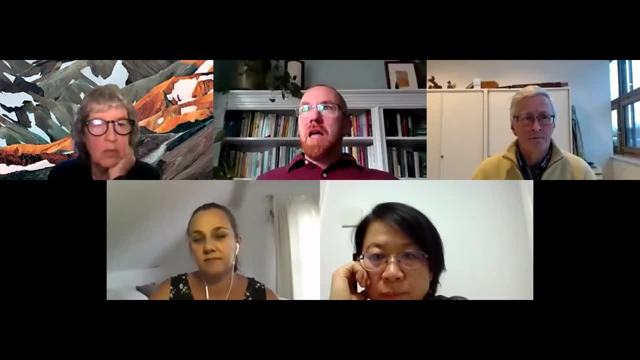 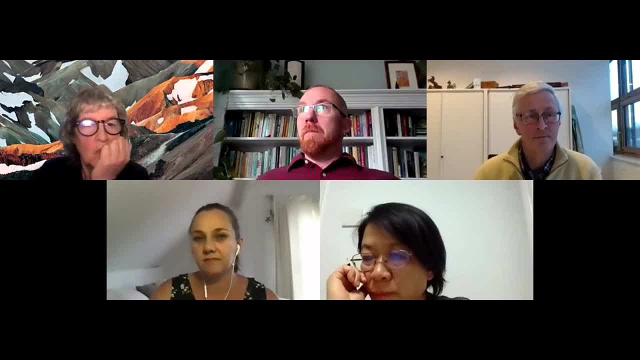 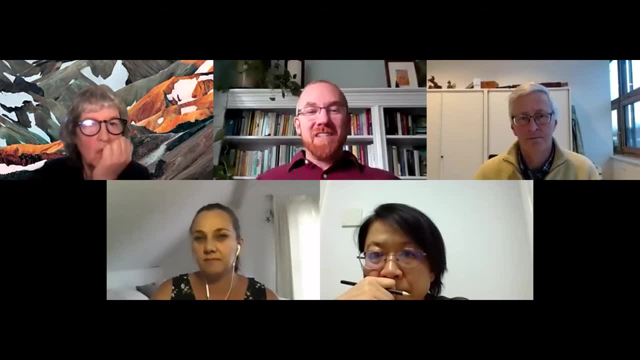 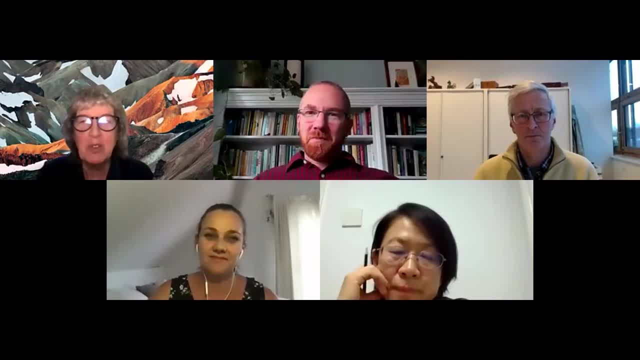 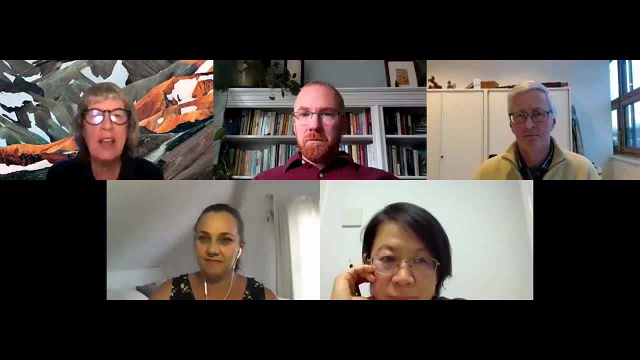 my head response: Yeah, great, Thank you very much. We have a lot of questions. I'm going to keep going here. There's a couple of questions that are regarding how to get engaged with these activities. Zolfikar Sagi asks as a soil scientist or ecologist. 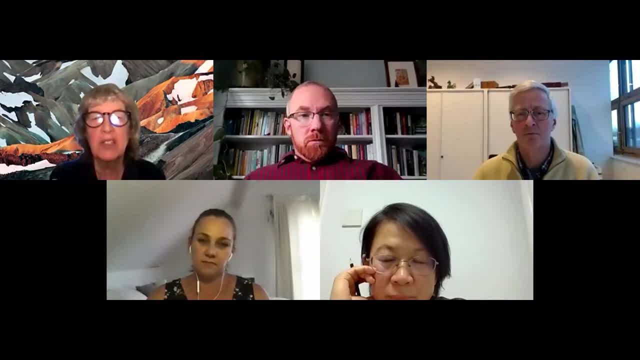 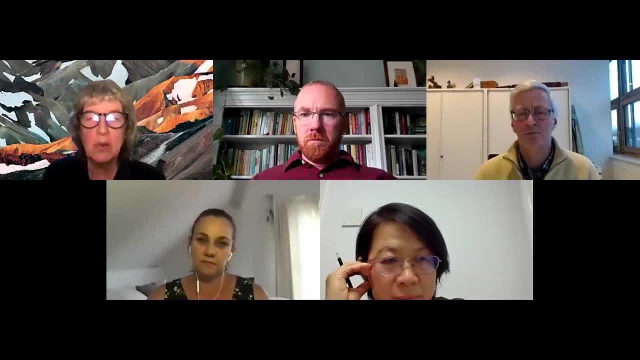 in various countries. how can we contribute in any global initiative like the GSBI with our limited resources and data with us? And then there's a question similar from Eric Towe: What sources of funding are there for students from Africa who are interested in soil biodiversity studies and education? 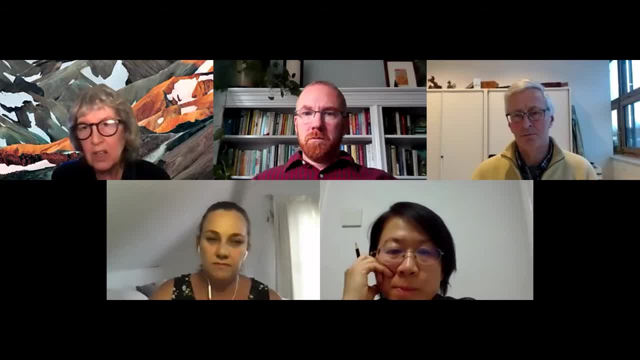 And I think we could start there. Sure, Okay, All right, start with Charlene. maybe you have some thoughts about this and then maybe we'll follow it up with someone else and, if any like, if anyone wants to contribute, please let me know. yeah, from from my. 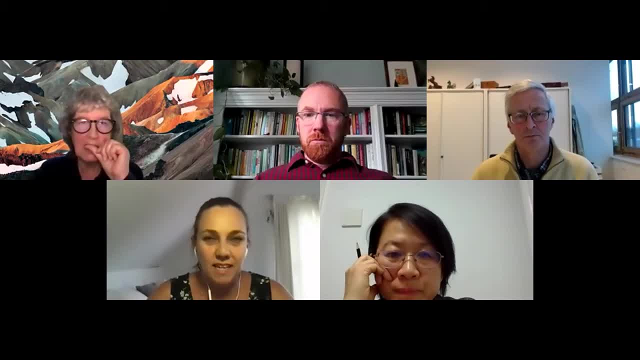 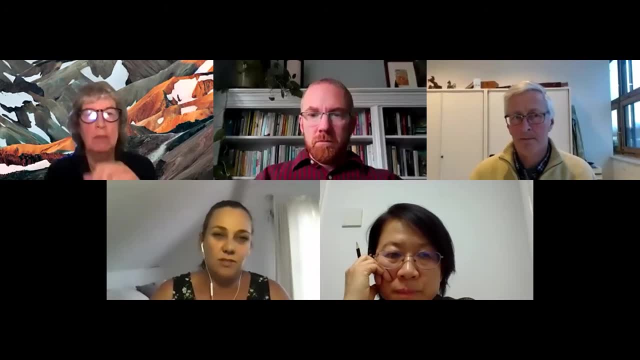 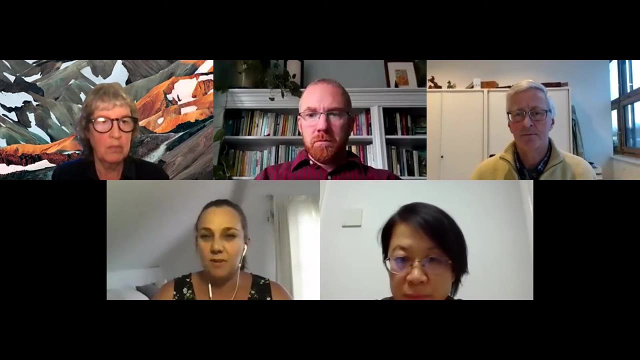 experience. I became interested and grew as a researcher by just being very collaborative and you don't necessarily have to visit countries, but definitely the knowledge that has been built in Europe for generations of soil fauna. you really want to learn from the the best of the best, and I had the opportunity to work with taxonomists from France and Russia. so I would say 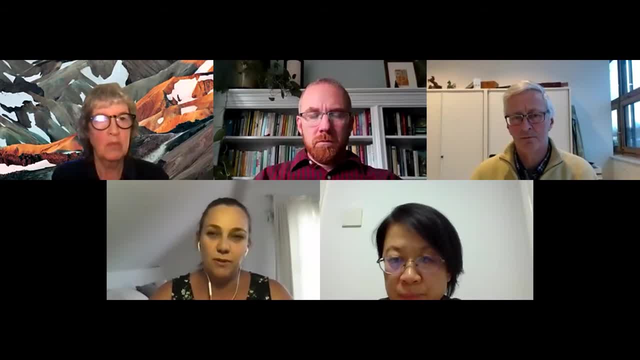 collaboration is the key contact people you know and in terms of the, the question about funding for for students for from Africa, certainly in South Africa I know we have many collaborations with African countries. I encourage you to look at the NRF, the National Research Funding website of South Africa there. 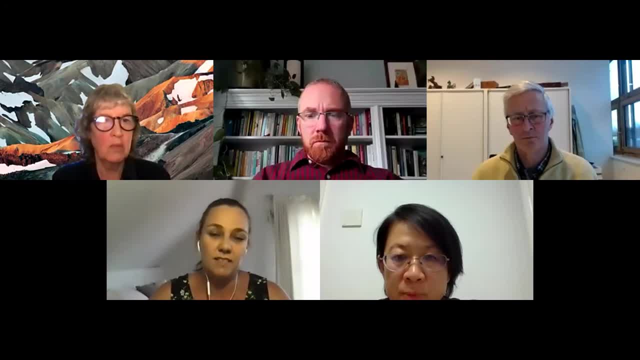 are a lot of opportunities with different universities to collaborate. there are also many European countries having bilateral grants with South Africa and I think that's a very important point and, as I think, Vim, you pointed out, that there's a huge gap in African soil biodiversity knowledge, and I think African countries have a lot of opportunities to collaborate with. 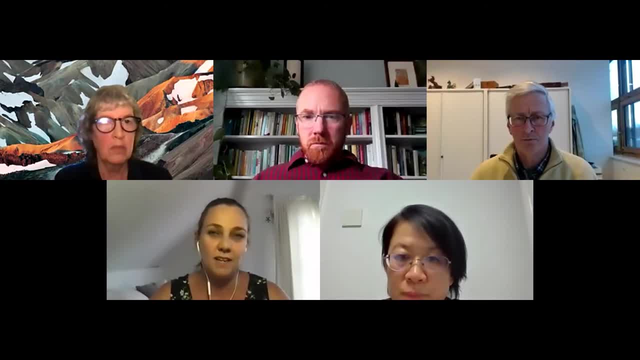 different countries, if you just want to enjoy it, I think. how did you explain that? the language? and in Africa I mean maybe be specific, what language would that be to compare bulk knowledges? well, these wait on that, but what? Rose Power? and another one that I have: U90. 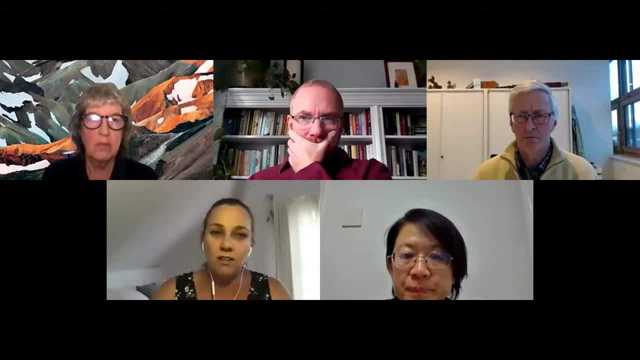 to read: we much to market, more to organic, however, will be really hard hit by climate change. so I think the future and the key is really collaboration. from my experience working on Kalimbola and the past 10 years- it was just me working on Kalimbola- 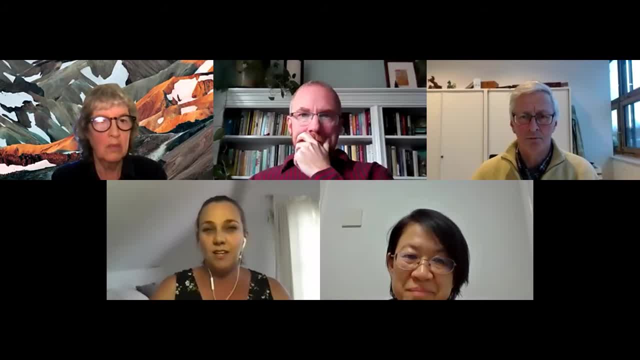 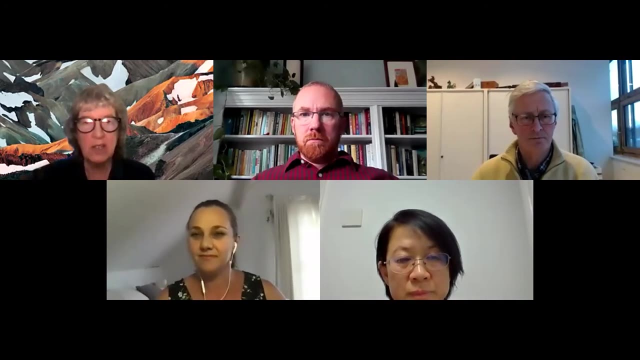 and now we're almost 10 people. so I know it's possible with the right collaborations and a bit of hard work and just yeah. so I think that's my advice. thank you great. thank you very much. we have a policy question that I think I'll target Wim with. what are main factors which? 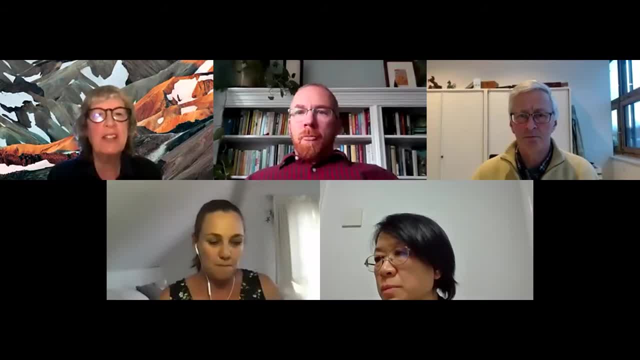 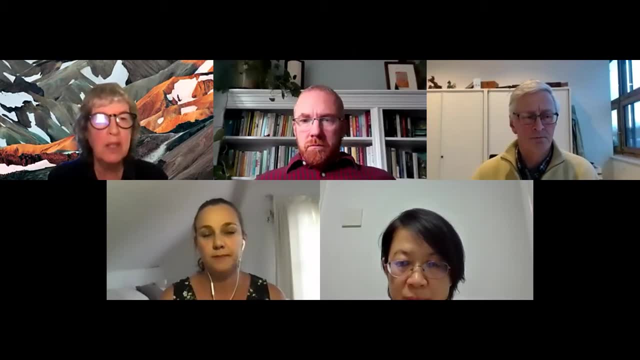 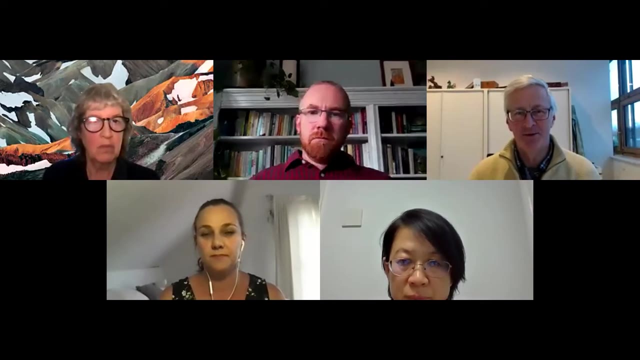 inhibit the implementation of more efficient? what are the main factors that inhibit implementation of more efficient policy measures for soil biodiversity protection? from Catherine Deglemeyer. yeah, well, if I start with the European Union, we don't have a soil like a soil act. so the soil director. 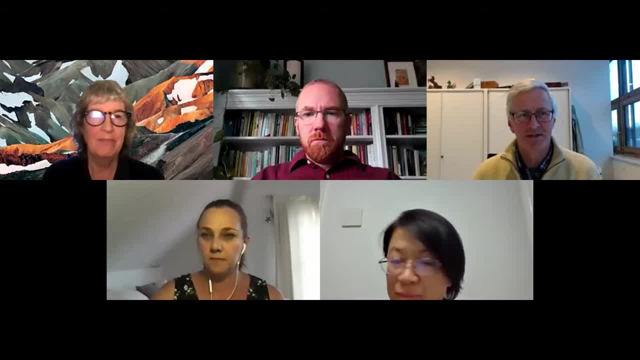 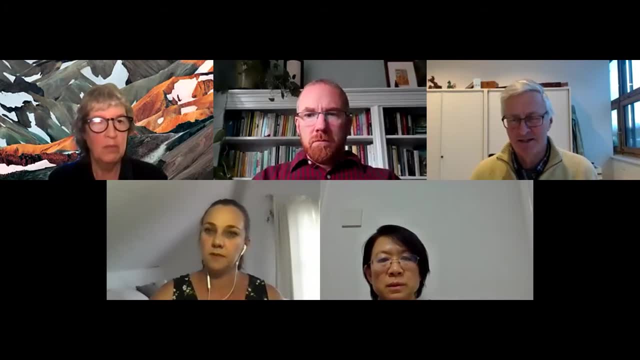 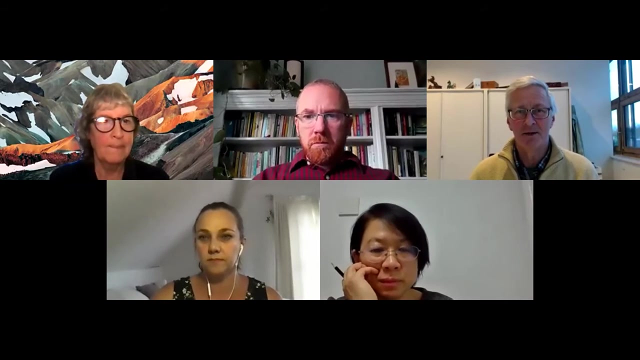 failed because of some countries blocked it and I, to my shame, the Netherlands was one of the countries blocking that, and they all did it for a different reason. so one of the factors that inhibits the implementation of efficient measures is that often there is no policy. so first we should have policy, so for Europe, we try to solve this. 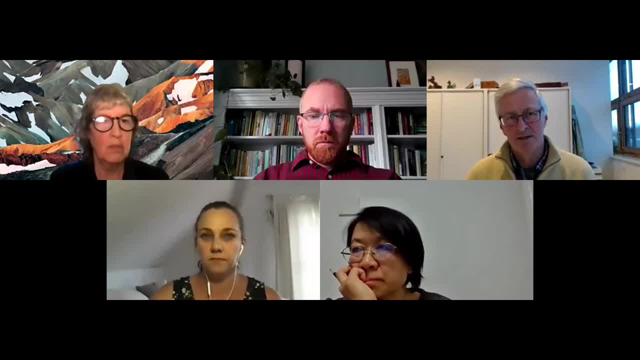 in a study done by the European academies of science, and this is the study can be found on the internet, you can download it. and what we did there is we said: well, actually, soil is important for, for nature conservation, so it is important for food production, so it is important for climate. 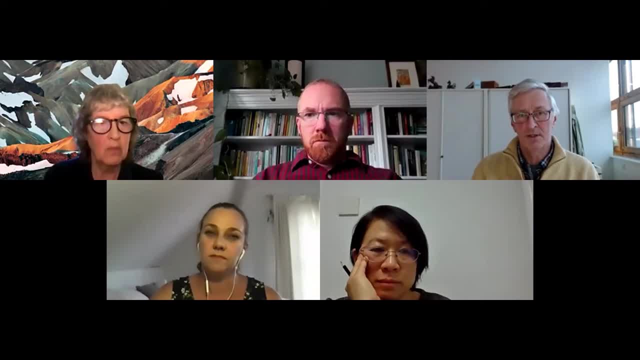 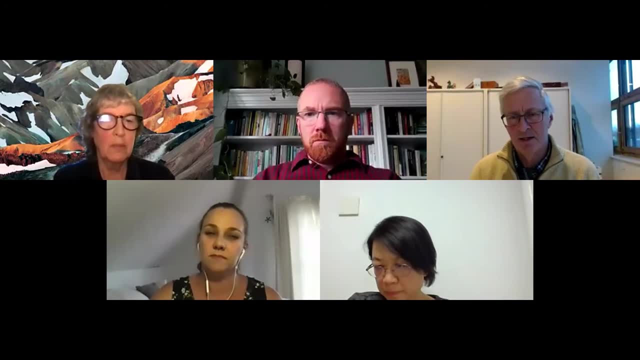 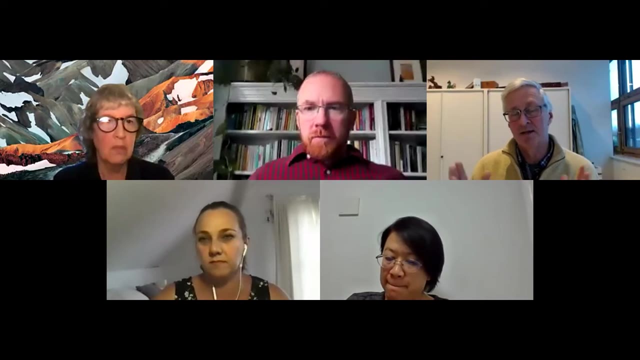 and for human health, and if we don't have a soil directive that can directly protect soil, then we can protect soil through all these other policy areas. so sometimes you have to be creative in order to find the right solution, and so this is only a European example, but you can. 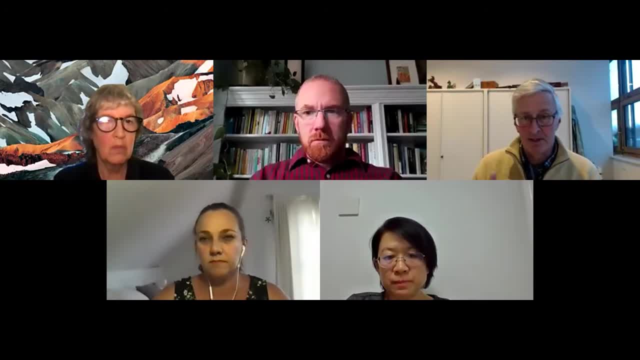 give the examples for different countries in South America, Africa, for China, and so I think the real solution there is being creative. and if you can't just get the, the, the, the, if you can't get the people to motivated to have a soil act, then you can tell them soil. 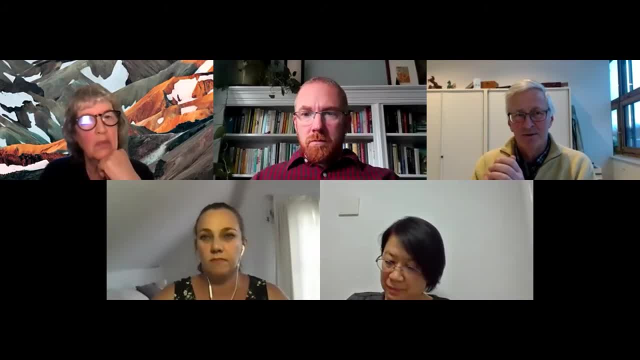 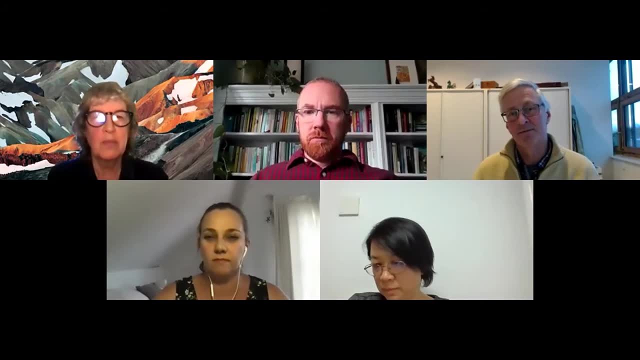 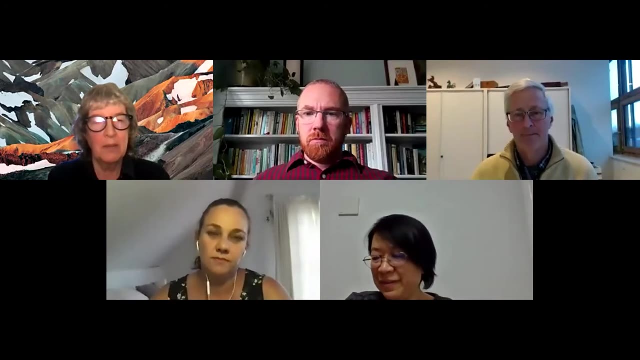 is crucial for the quality of your food, and soil has to be placed in the on health ideas. so that that would be my answer. okay, great Chunling. do you have anything to add to that from the Chinese perspective? yeah, thanks, so yeah, as we mentioned that here in China, soil is. 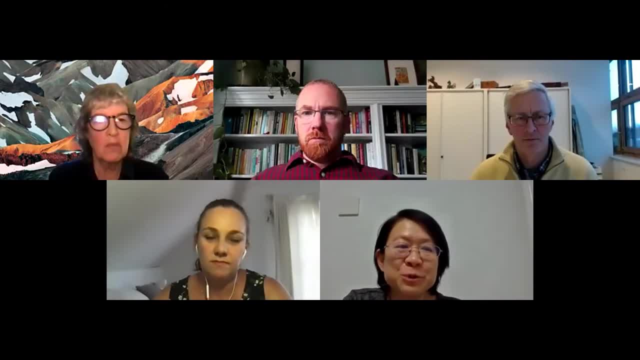 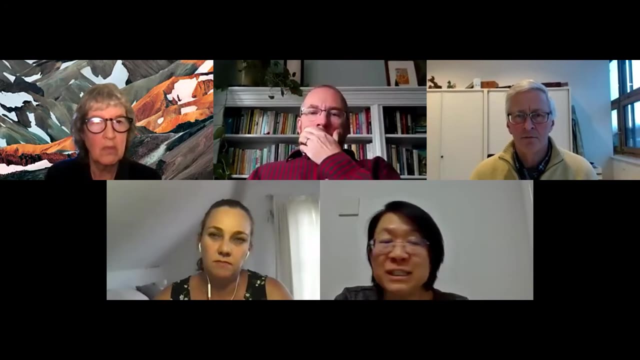 very important because we have a lot of pressure, because, as I mentioned, because the huge population here in China. therefore so um program, there are a lot of programs regarding soil protection or soil conservation, and even though it is the AGD program, um, it's launched 2017. 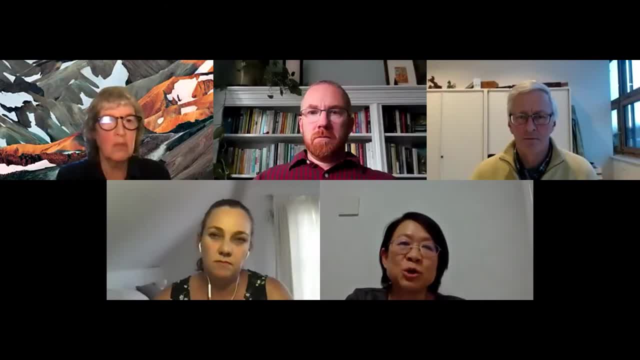 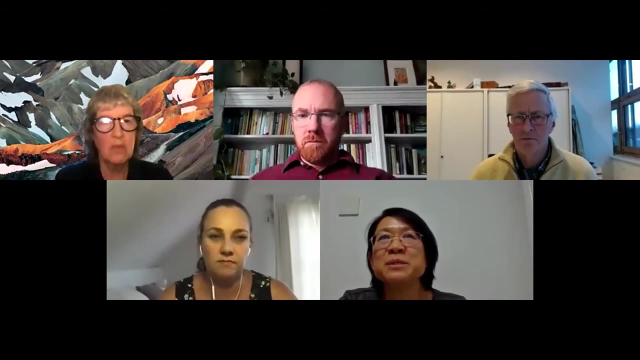 and Ministry of Agriculture, Ministry of, is really pay a lot of attention to for food security. therefore, soil is a place to to have start. so i think that, um, yeah, it's really as mentioned, as mentioned by them, it's really dependent on different countries, but uh, so it's really precious because it's really 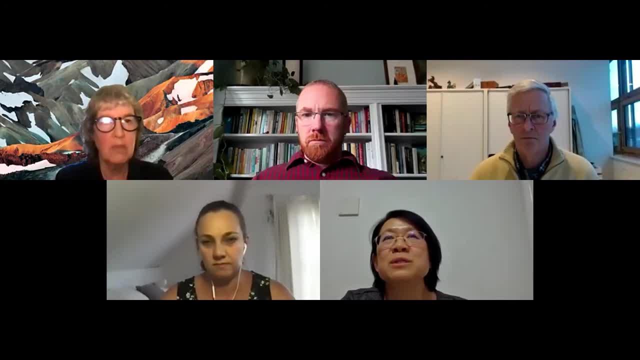 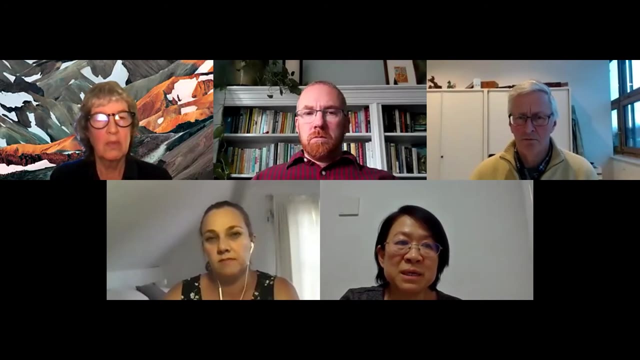 highly connected to the human health and also to the um, to to human health as well. um. i think that in the in the coming uh, in china at least, there are a lot of programs coming out related to soil, so it's a good start for soil scientists and also for other scientists working. 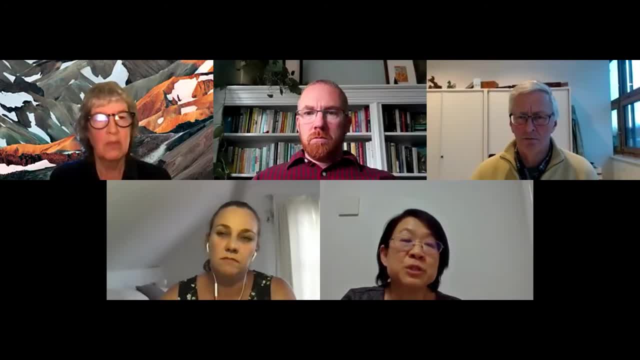 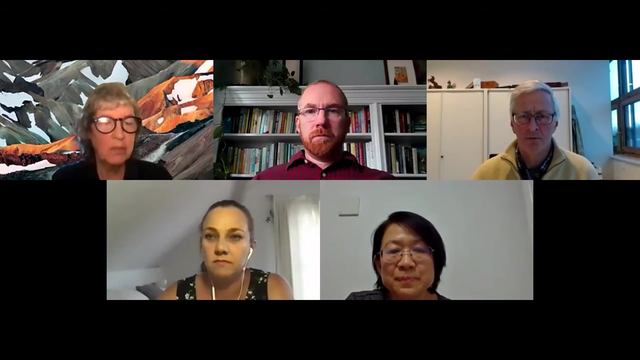 together to really to maintain food security, not only for china, but also globally. so i think that by doing all kinds of collaborations among different regions, different countries, that they're always great opportunity for us to promote soil programs. yeah, okay, great, thank you, um. there um are a couple of questions about urban soils, so i'll start with lauren on that. 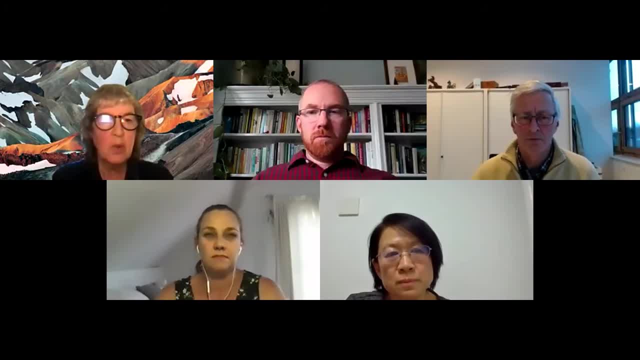 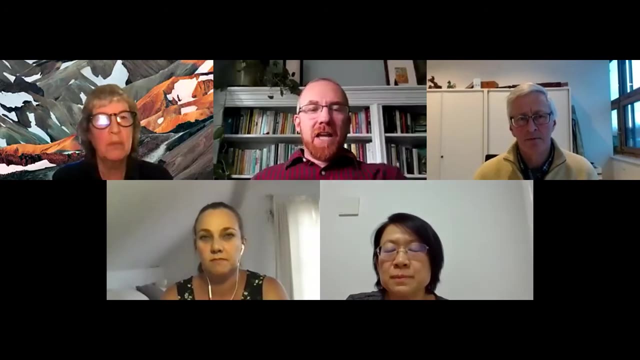 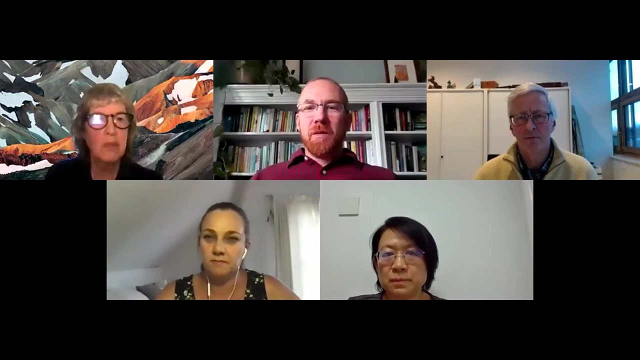 what are the main suggestions to improve the biological quality of of urban soils? and i think there was another question about um. that was um. sorry, yeah, i think just start with that one. yeah, you know, kate, i i typed an answer to his second question, so it probably um. yes, this is odoardo's questions about uh. 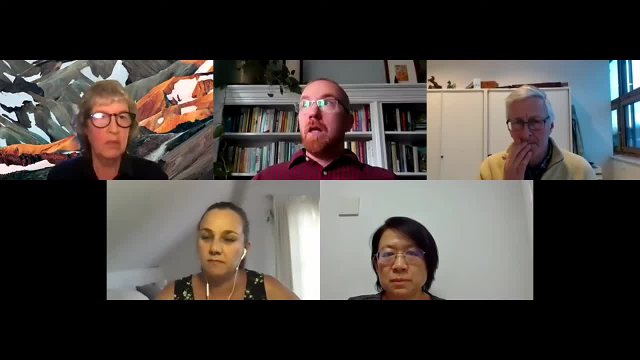 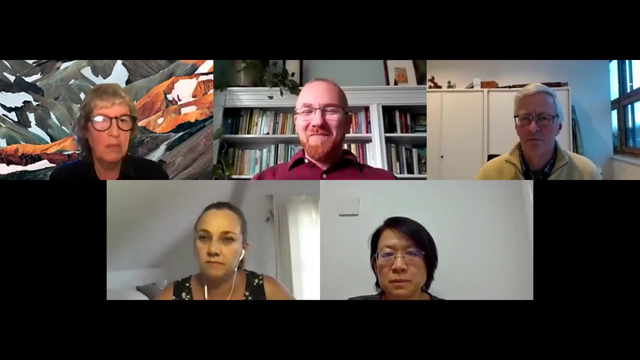 bio: the biological quality of urban soils and grown food in them. um, i just wrote uh well, it just came out uh a chapter about urban soil restoration. so if anybody would like um my personal pdf copy of that, i'm happy to share it if you want to email me. um, urban soils are often. 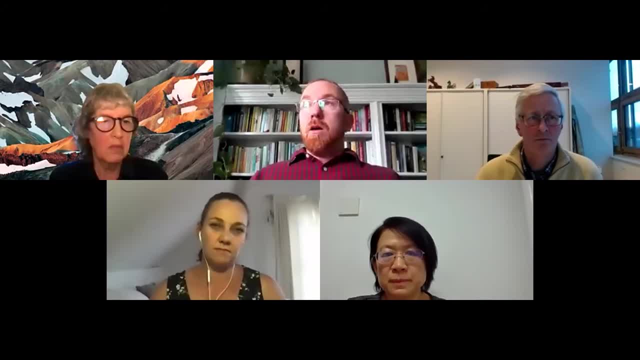 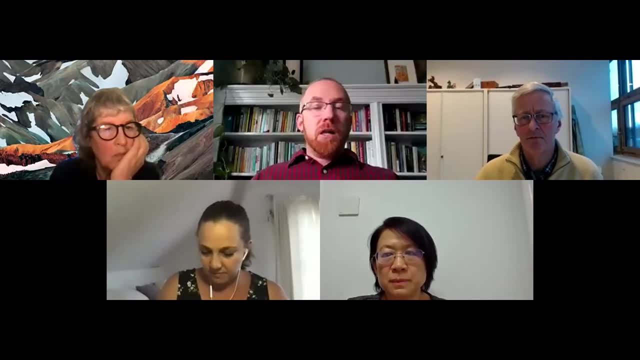 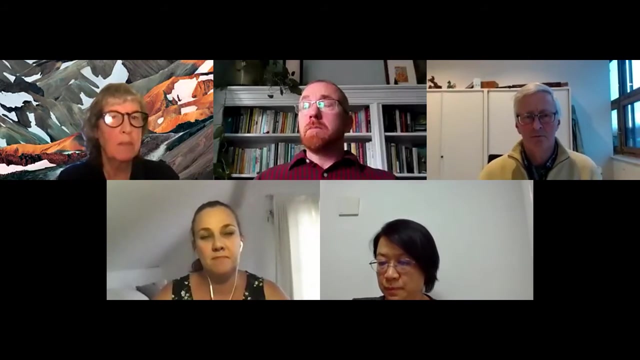 degraded, that's true, but not always uh. so that's a key starting point that sometimes urban soils have very high quality already. so a big challenge for urban soils is site-specific investigation. because of their very complex histories and landscape contexts, we need often very specific information about them as a baseline, um, if they are found to be degraded, uh, through compaction. 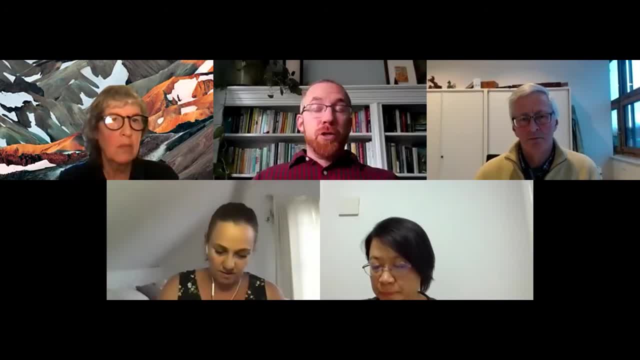 loss of organic matter, uh, erosion, of course. um, there are lots of strategies that can be taken to improve urban biological soil quality and in the review that i prepared for the book, chapter uh, most of the research has been done about adding organic matter to these soils and uh, by and large, that is the key first step, because we know that organic matter in soils provides food for the organisms. it helps the aggregation. it can also bind up some of the pollutants and prevent them from being taken up by crops. that is a key starting strategy. now the more nuanced response is: well, what kind of organic? 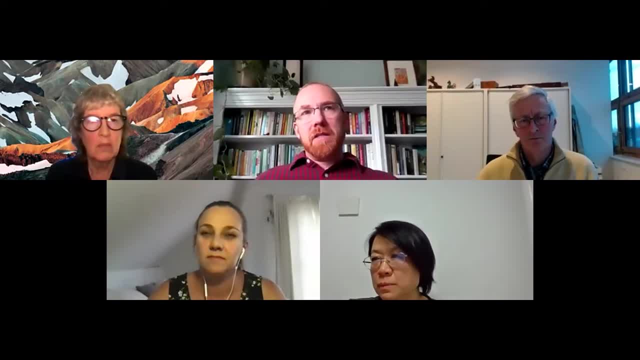 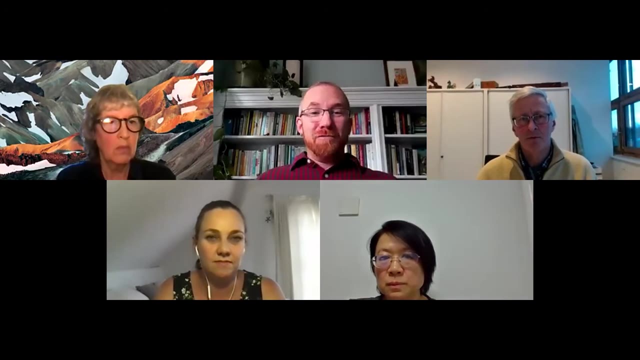 matter. there are lots of possibilities and you have to pay attention to some of the the different types of organic matter that people are using, whether it be just basic compost of different food scraps or manure brought in. there's a lot of interest in using sludge from sewer. 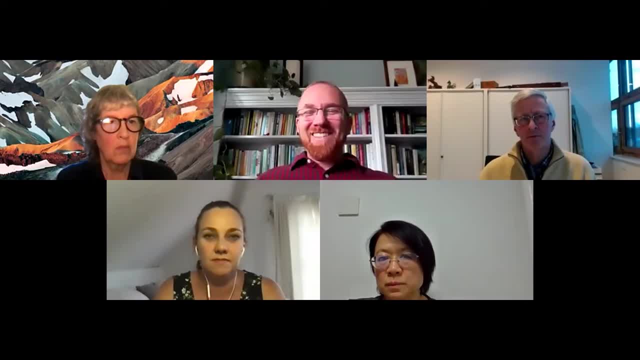 systems are basically human wastes once they're treated. they've been used. lots of possibilities and of course his second question was about specifically about pollutants and we have to be very cautious of that. but we know from lots and lots of places around the world who have been doing urban community garden. 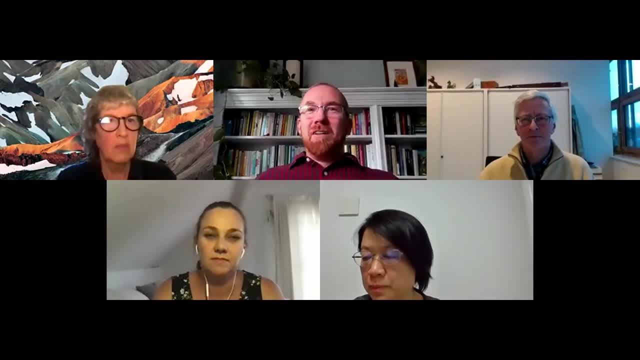 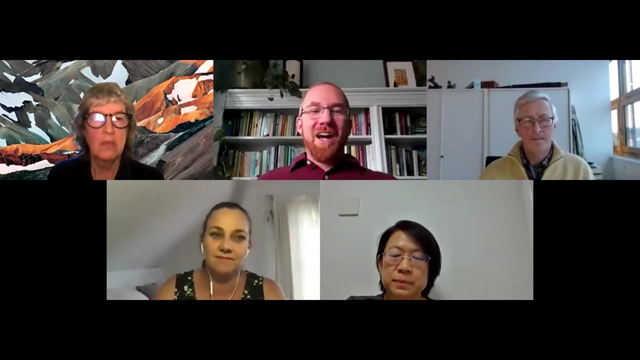 for a long time that it is possible to have local, fresh, healthy foods from urban soils. so, yes, we can put a lot of emphasis on those and that may be some of the other questions- a great way to engage policy makers for further. you know, having gardens right outside the the houses of congress and government, um talking to them about soil in their 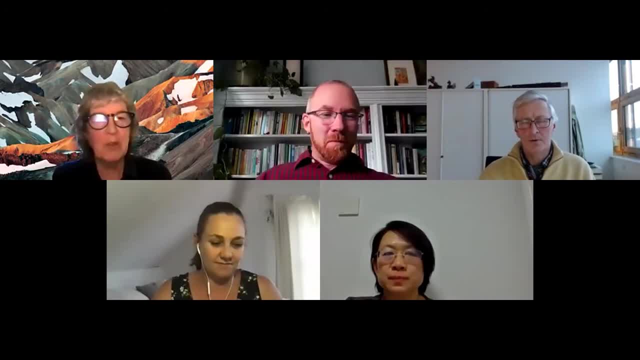 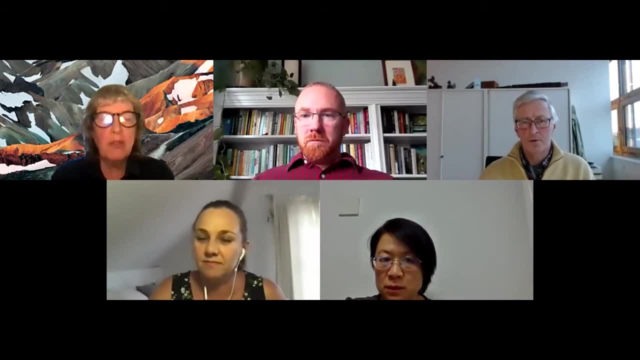 terms of areas of cost. right now it's really up to them to establish what they need to do for their area of cost in their particular communities. so if you can get some good feedback on that can also be helpful in the midst of any other work environments. 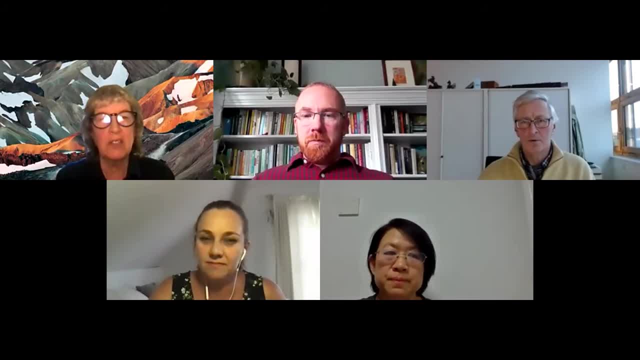 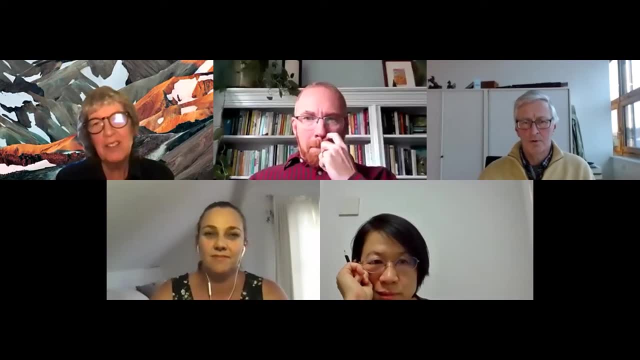 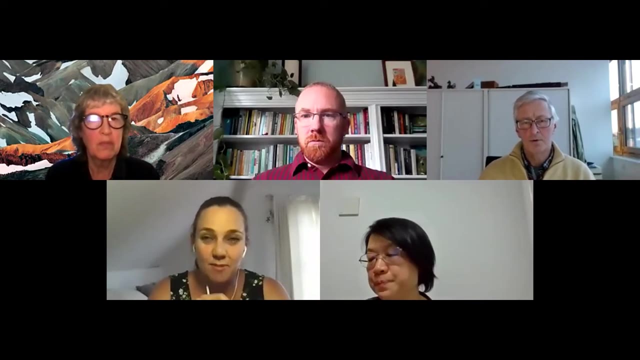 yeah, great, thank you very much. i'm going to direct the next question to charlene. this is from cesar marine. could it, could it be possible in the future to establish conservation areas based on below ground biodiversity hot spots? There has been recently a review by Erin Cameron, who was my co-author on this chapter, about the linkages between below and above ground research or the sort of the mismatches actually. 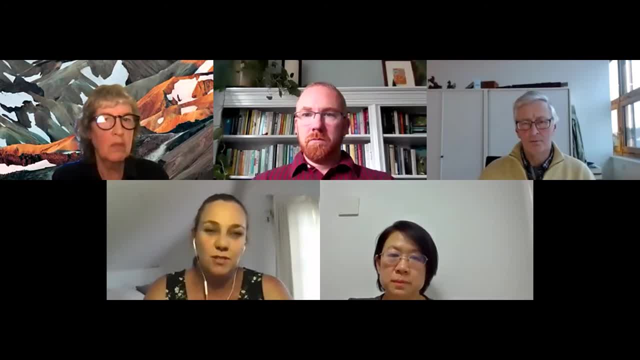 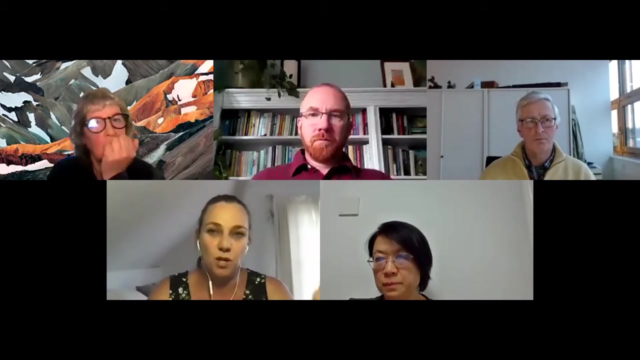 But from the experience here, the first start is to know what you have- And we're very fortunate in South Africa to now really have a good grip on the soil, biodiversity, at least taxonomically, And then to, as part of conferences, to just publish all of this material, have the data available, which will then feed into policy. 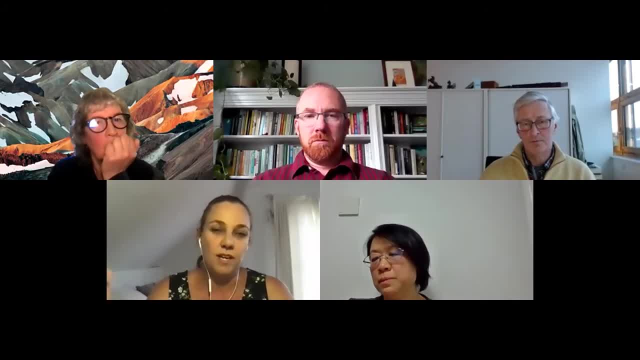 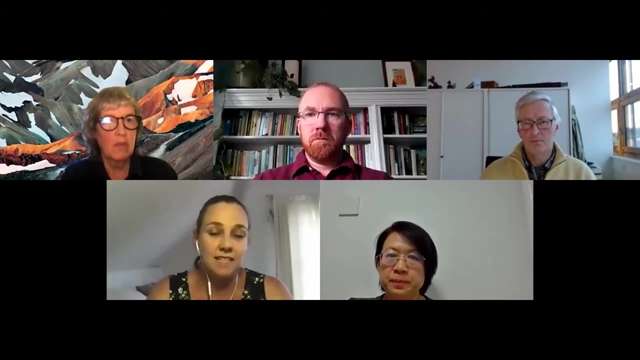 And in our situation we are feeding it into reports, into our national parks, for instance, which are usually the biodiversity hotspots, And that way managers, land managers and conservation agencies, at least here, have real data, have empirical evidence. 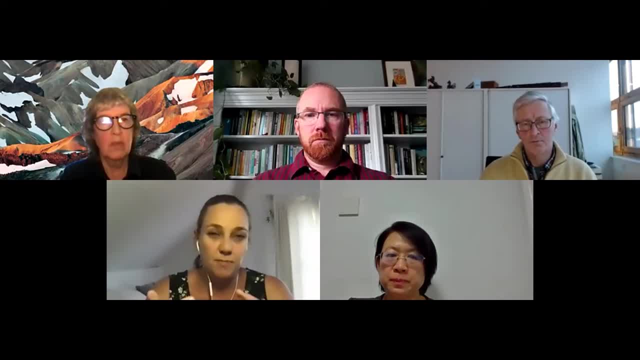 Of the really high biodiversity, even if it's below ground, And furthermore, I think, not only biodiversity data, but also ecological data, such as predator-prey interactions, for example. I'm very interested in how columbula are basically the top prey for spiders, for example. 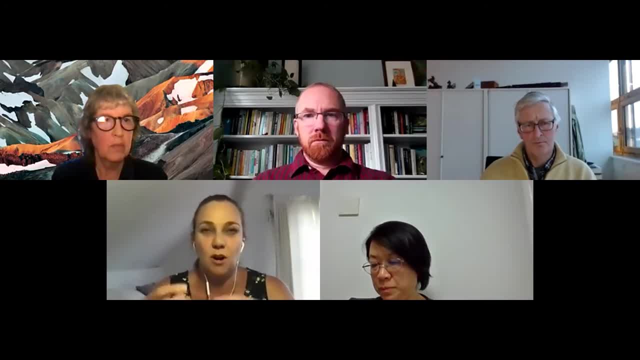 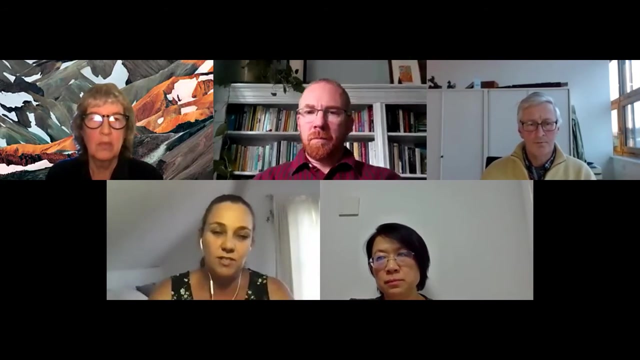 So once you get a bit more handle on these really complex interactions, I think conservation, Conservation agencies will take notice and realize the services that the soil, biodiversity is providing, if that answers your question. So I think the start is really know what's out there and just widely distribute it, not only by research articles, by popular science, like The Conversation. 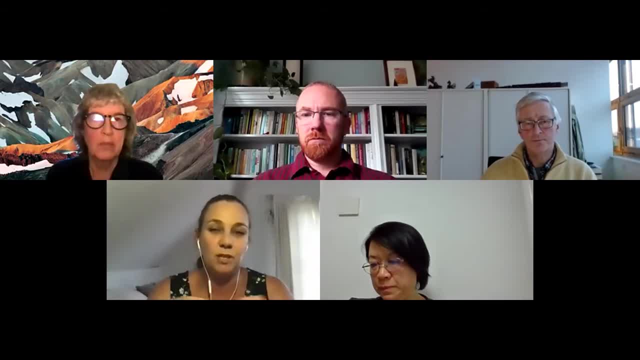 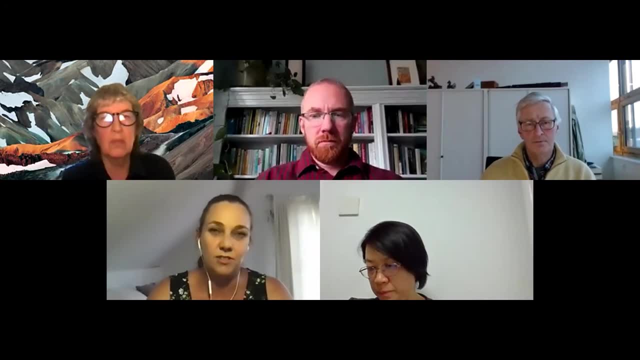 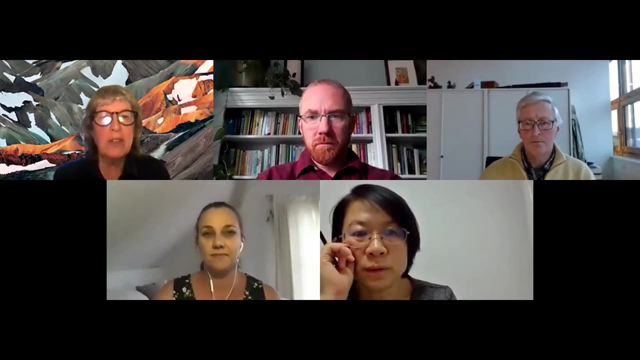 In here we have The Conversation: Africa get it out because people read it, newspapers read it And they That it gets to the right people who make those important decisions. Great, thank you very much. Next question: To what extent do you think that soil biodiversity has already been changed due to land use change- Forests, grassland, arable land- in the past 500 years? wouldn't we expect that we've already lost a large part of, in this case, soil fungi in the past? 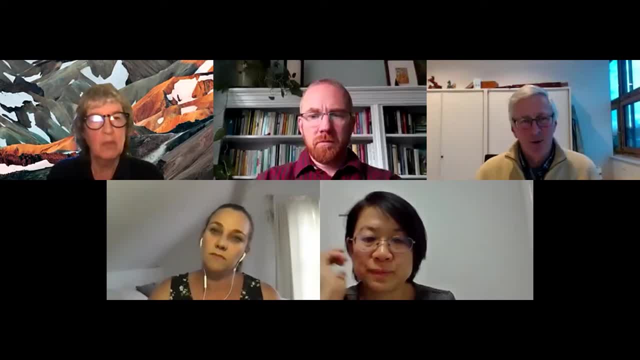 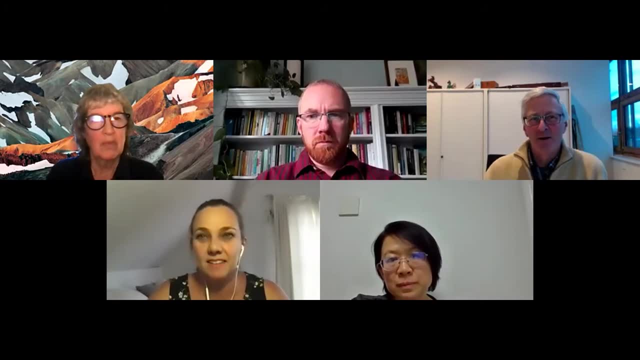 Yeah, I saw the question. It's an intriguing one. I immediately I had to think back to what Jim TJ once told me. He said soil is the dustbin of history, and so whatever enters the soil will stay there for a long time. 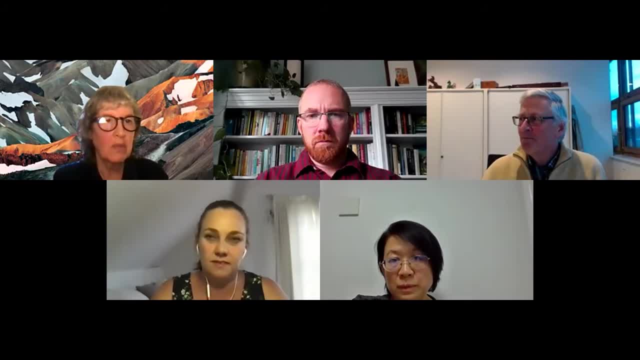 So, thinking about that suggestion, it might be that still a lot of the things that you think that they're gone, that they still might be there somewhere, but we for sure have changed soil biodiversity a lot So over the last 500 years in the various continents. 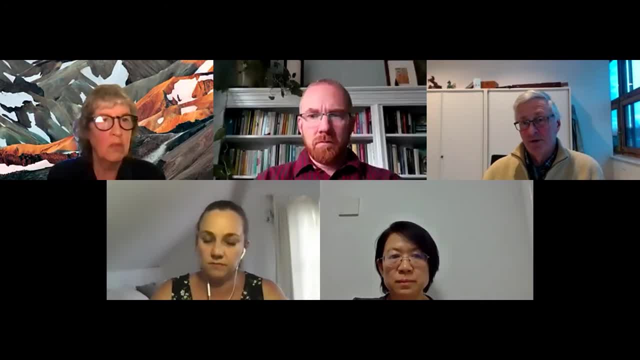 we have had a lot of deforestation And so if you would change the forest to a grassland or an arable field, you're going to change the soil community strongly And I think that in the world that we are living in now, with much higher productivity in most areas, food production, timber production, that we are driving soil systems from more fungal dominated to more material dominated, but even more that we also changed the whole efficiency of the carbon processing through soil. So we are losing a lot of carbon. The carbon is less processed through the soil. and food web And staying into the soil in this world for a long period of time. Also, I think we are changing the soil more towards sort of pathogen and herbivore dominated and going away from mutualistic symbiont dominated. So those are the big changes that we are seeing. 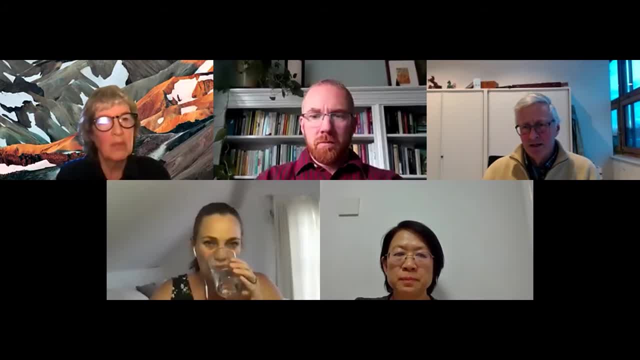 But I think that if you're going to look, you still will have certain sites that are maybe not exactly the same as they were, for example, in the past- I mean, they were there 500 years ago- but they still have characteristics of the types. 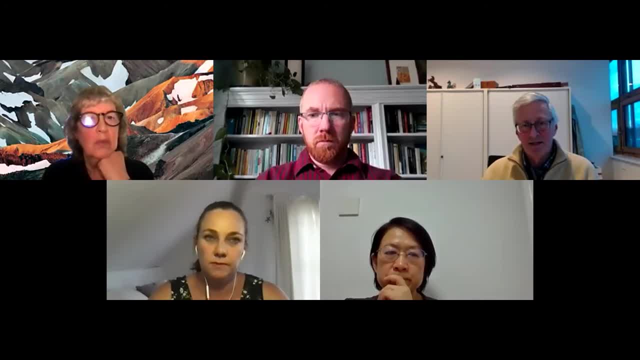 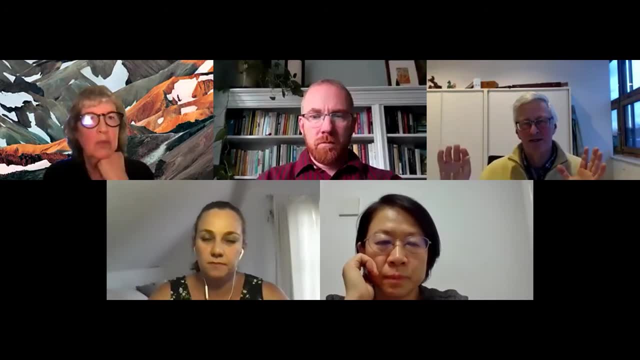 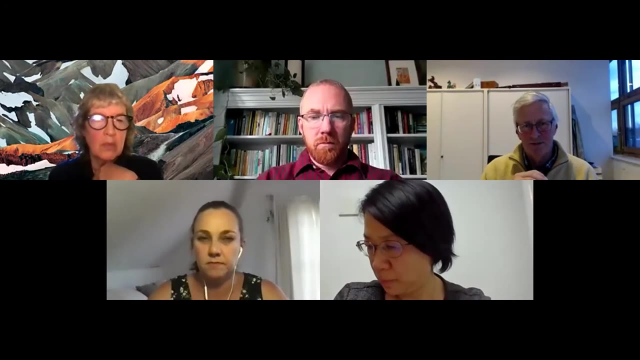 of ecosystems that were there in the past. And it's interesting because above ground you would just in these fragmented areas, you would have lost all the above ground biodiversity that is expected to be there, because these organisms need a much larger space to live. 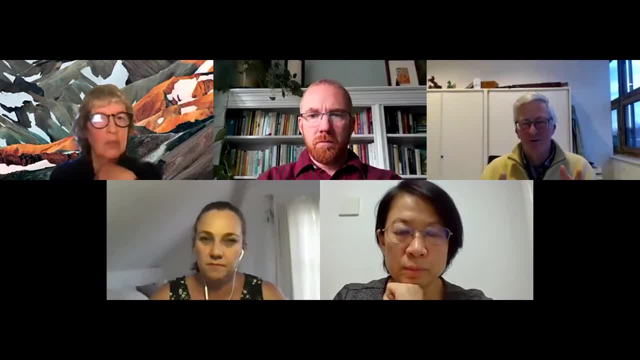 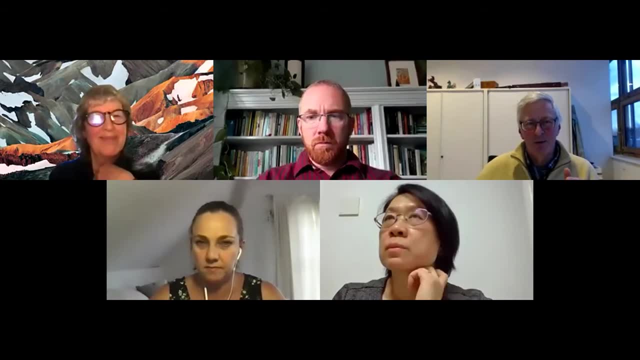 But the interesting thing is, if you're going to sample underneath the tree, you will have the. you will have the soil community of a forest. If you're going a few steps away from the tree, you will have the soil community which is characteristic of a piece of arable land or pasture. 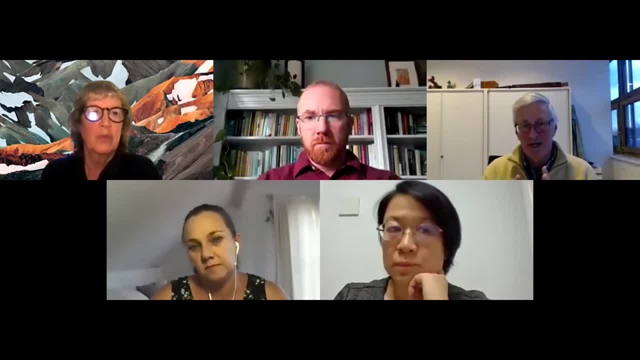 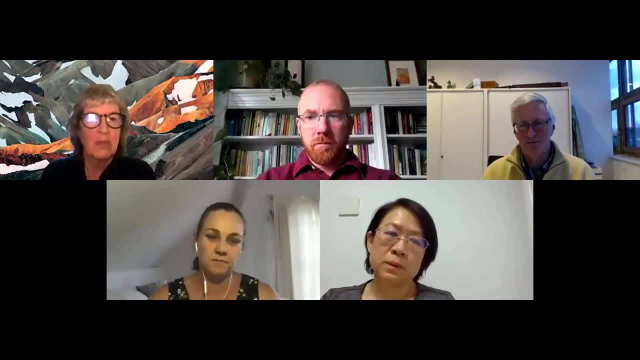 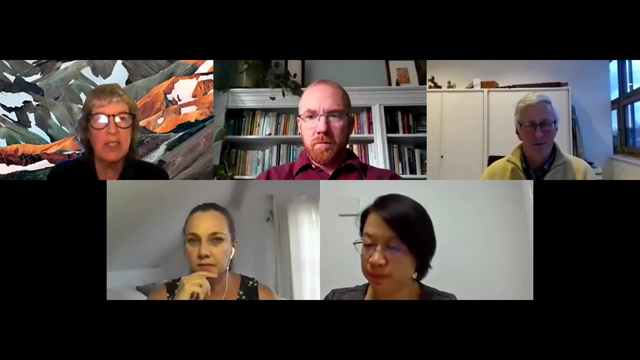 So I think there is still a lot of soil biodiversity there that used to be there at much larger distances in the past- Great. Thank you so much, Zhenli. I'm going to ask you a couple of agricultural questions. Pradeep Dede asks. 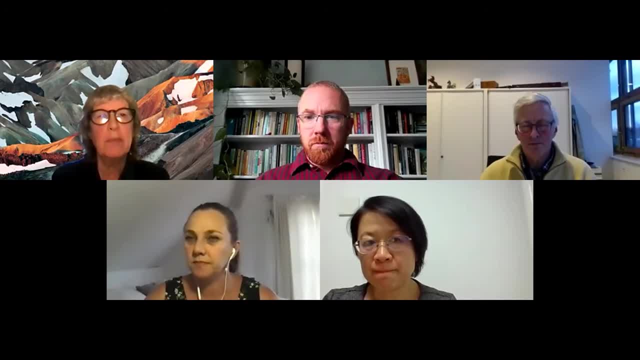 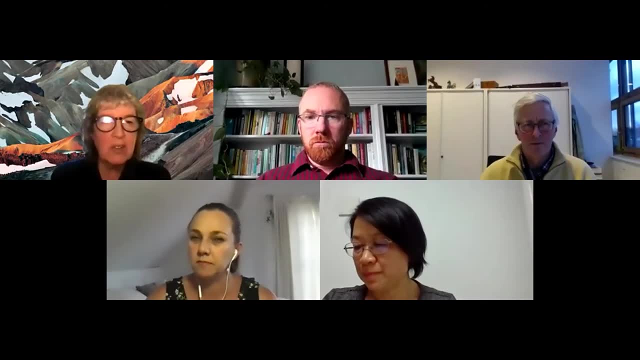 soil biodiversity is key to nutrient cycling: How to balance nutrient mining and recycling to maintain soil health? And I want to add a second question: How, from Kalavakuntla Jeevanrao, how to maintain an optimum good soil biodiversity? 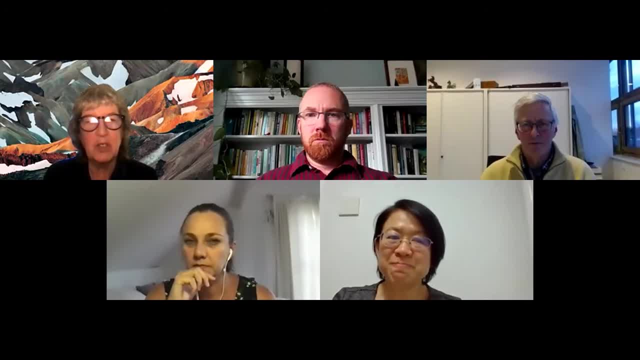 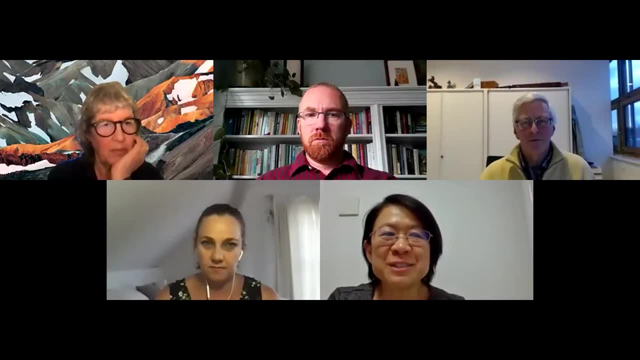 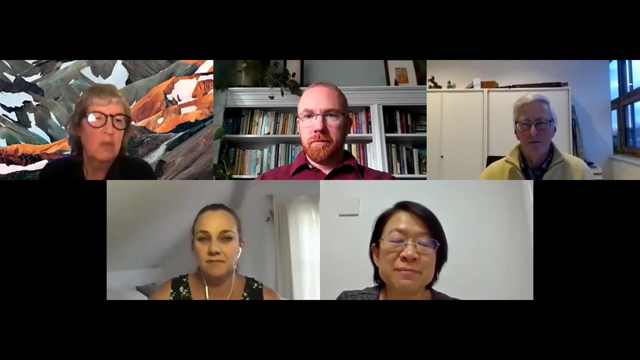 when we use agricultural chemicals. Could you handle those two, the two of those? They're slightly related. Yeah, Yeah, Oh, it's very challenging Question. actually, this is what we are trying to do at the moment. So what do we realize? that is that the beneficial ones? 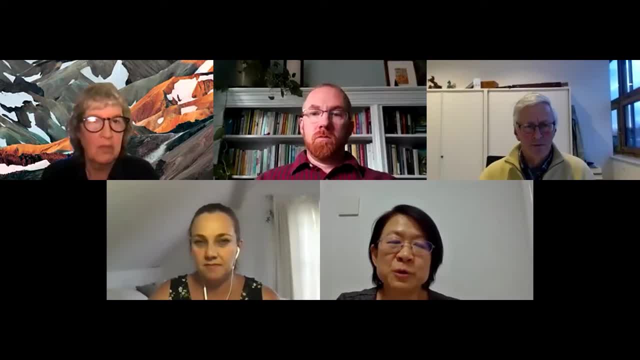 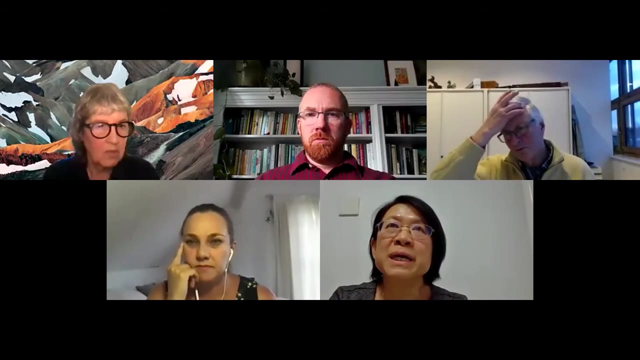 for example, if you give a lot of phosphorus fertilizers into the soil, then you've got a problem with mycorrhizal fungi. So proper amount of application of fertilizers is very important. We carry, we conduct a national wide survey. 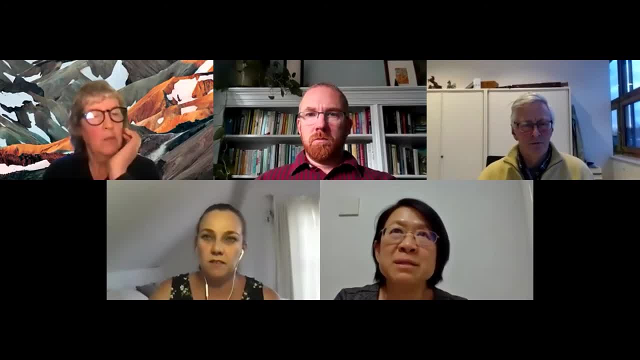 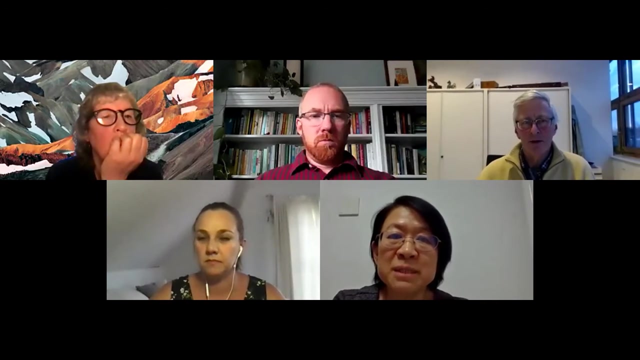 about soil microbial abundance in agricultural soils And there's still huge amounts. I mean amount is still huge, but the composition of soil, microbial composition is changed greatly. So that means the function group is very important. Sometimes people argue whether you know. 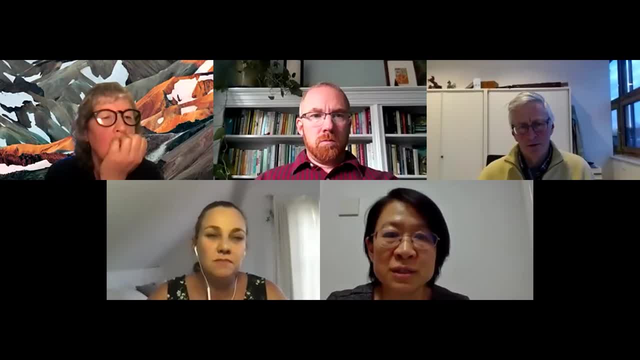 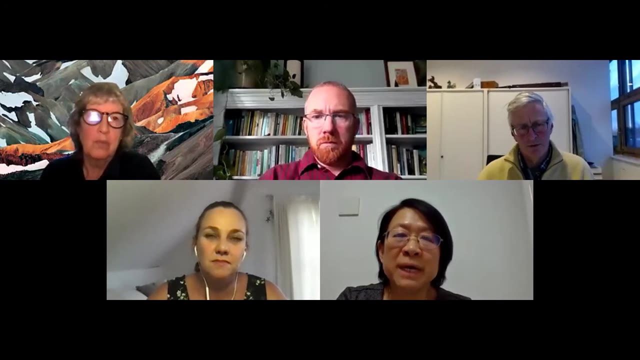 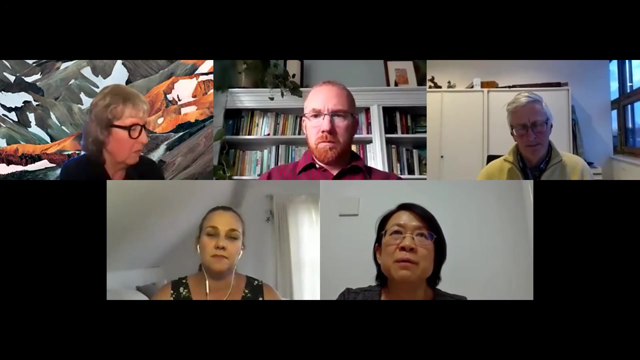 whether the abundance is important or whether composition is important in ecosystems. agriculture, land, function. Probably the function groups are much more important. Therefore, when we manage the agriculture, soils, then you really have to consider the function groups. For example, if you apply phosphorus into soils. 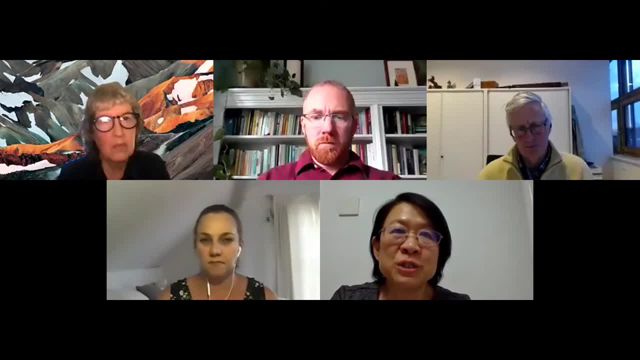 think about mycorrhizal fungi. If you apply nitrogen, you have nitrogen. If you apply nitrogen to the soil, then you have to think about the nitrogen-related soil function groups. So it's- yeah, it's difficult to say one solution for all. 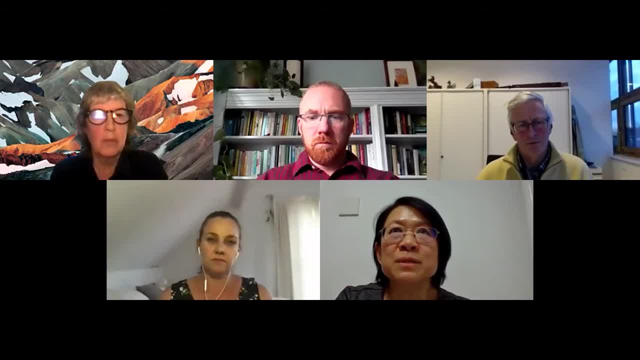 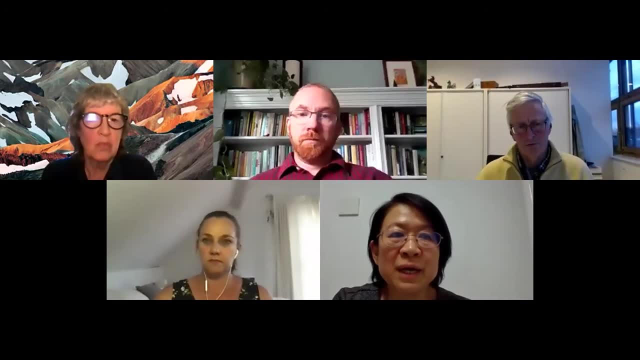 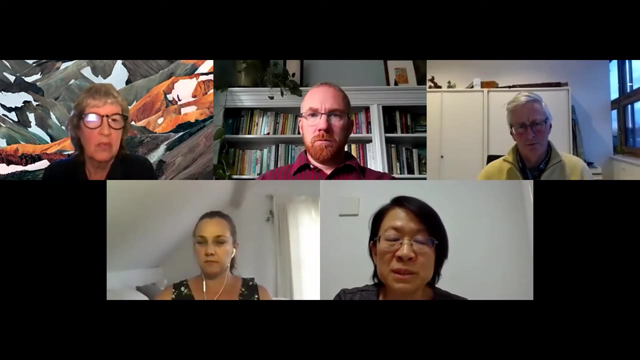 but indeed you have to consider about what kind of material you want to put into your soil And then think about then link that one with the soil, so microbial groups, and then use a proper amount of the nutrients in the soil. Then it's because, for example, 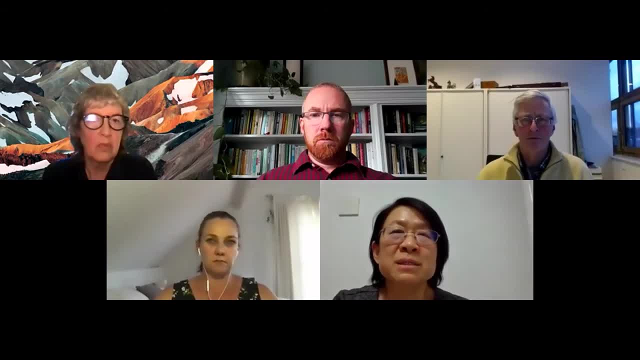 we have a forest-forest reagent experiments by using about well in North China Plain, by using about 30 milligram kilogram. 30 kilogram per hectare, that is a proper amount. A micro is a fungi is maximum amount. 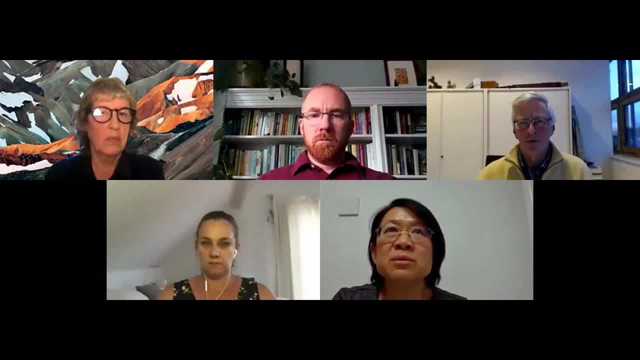 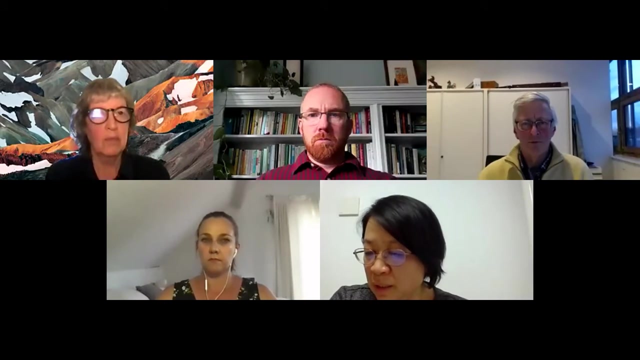 and also without, the yield is the highest. So you have to do kind of like a pilot experiment to find the proper amount for this kind of relationship relationships between soil microbials with the crop yields. Yeah, it's really tough and there is a lot to do. 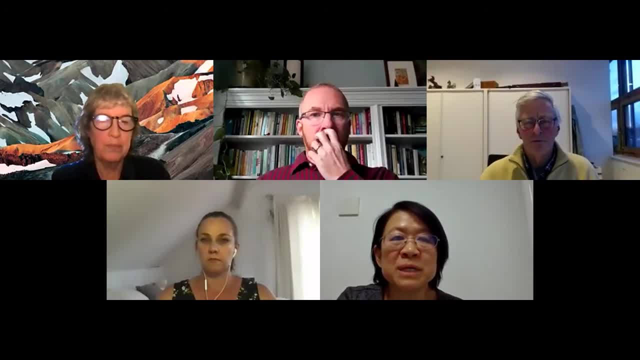 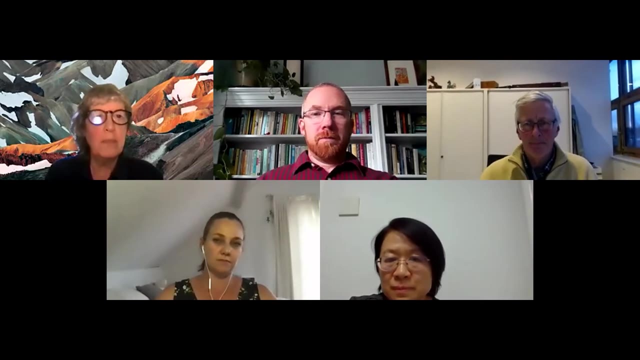 but with the advance of this microbial technology, the new technologies, there are always chance to be to do such kind of experiments. yeah Great, thank you very much. Okay, our next question is for Lauren from Zulfigar Sagib. 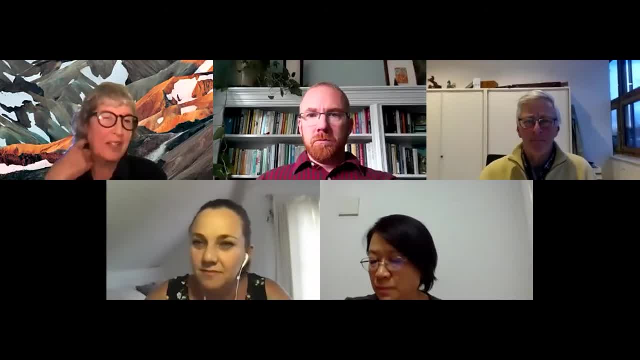 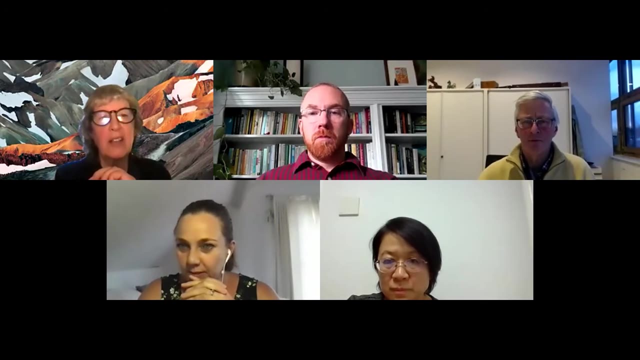 I'm sorry about pronouncing everybody's names incorrectly. What about educating the professionals about soil biodiversity? Many professionals working on various aspects of soil productivity do not bother, don't address soil biodiversity or ecology due to lack of proper expertise. So these would be like working professionals, I think. 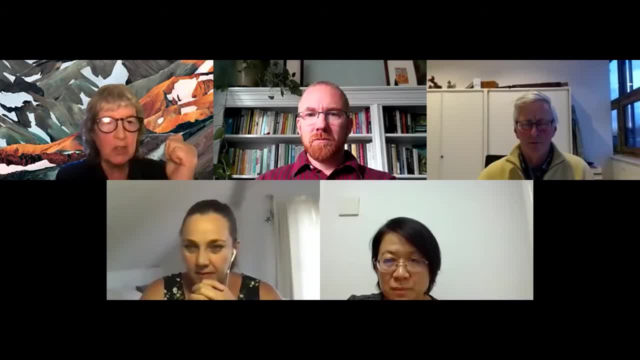 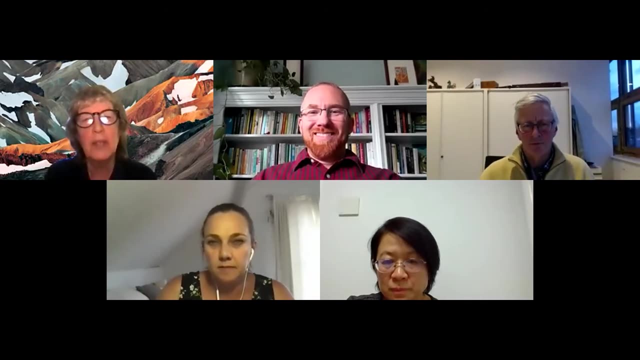 Any easy to do methodologies and standard determinations using recent tools? Could that be helpful to get information on biodiversity, anything in the pipeline like that or any other ideas about this question of training these practitioners, I think? Who may not think about soil? 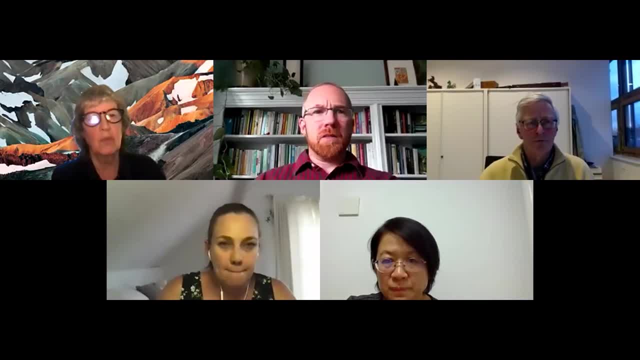 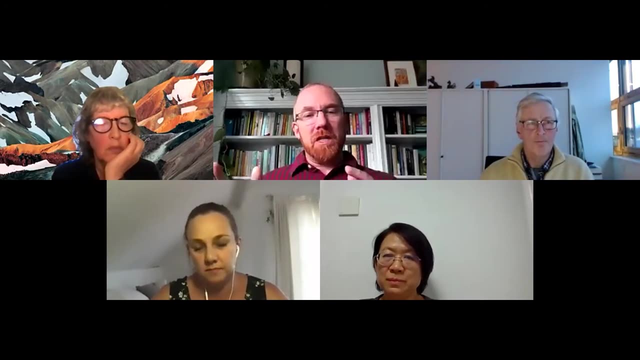 Yes, I'll share a couple comments, but some of the other panelists might be better prepared to answer this because they're more involved in some of these research methodologies. I've always been struck myself at this disconnect between professionals in the soil science world. 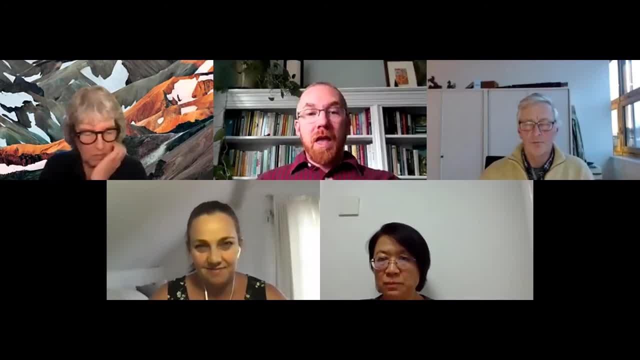 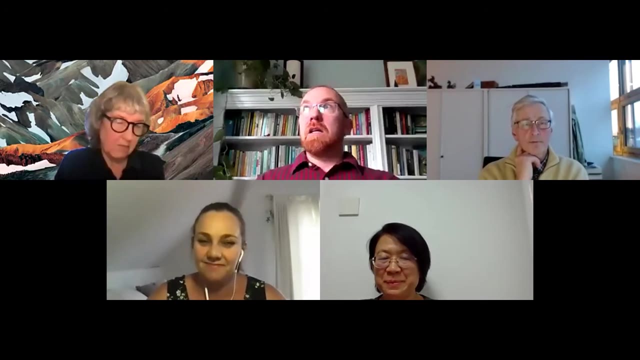 That's what I'll narrowly focus in on this question. for that and ecologists and soil biodiversity specialists, it seems that soil scientists often forget about the soil organisms, So I do think that this is a challenge connecting professionals and other types of scientists with the soil biodiversity. 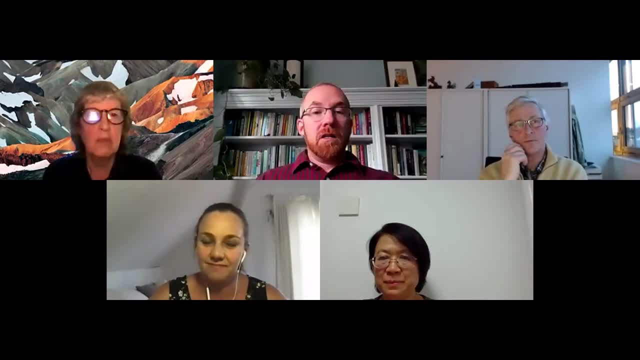 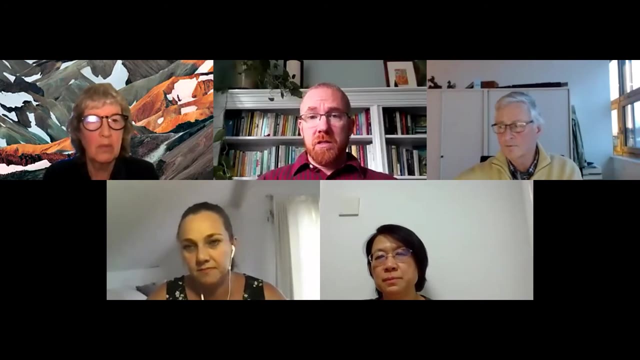 And maybe some of what I've already said could be applied here. you know, getting them to come to appreciate and respect the soil organisms and what they do in the soil in terms of formation over the long term and aggregate stability, and so forth. And then the second thing that comes to mind about methodologies and tools. 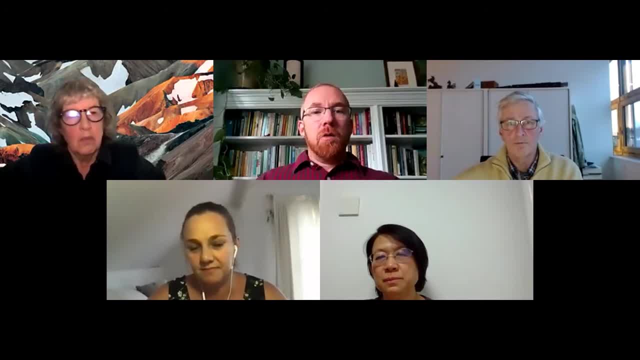 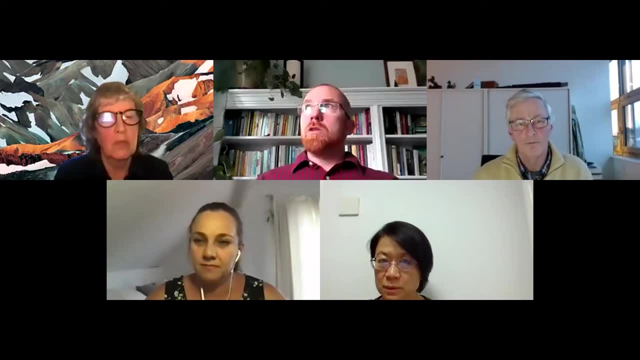 Wim mentioned that paper that just came out last week which I think actually lays out a framework for some possible methodologies And maybe he can speak more to that. And there was also a recent paper in one of the Nature or Science Journal groups about soil health. 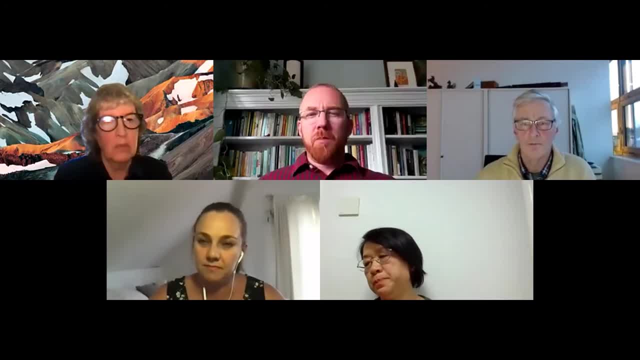 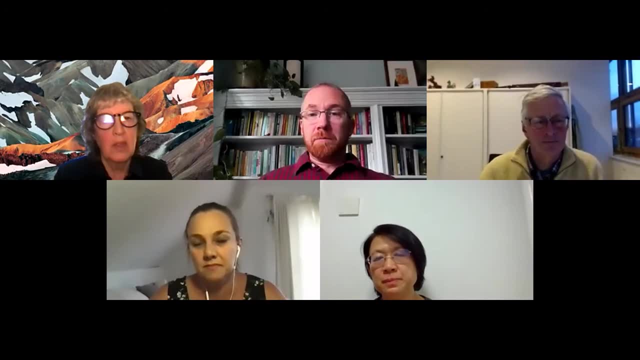 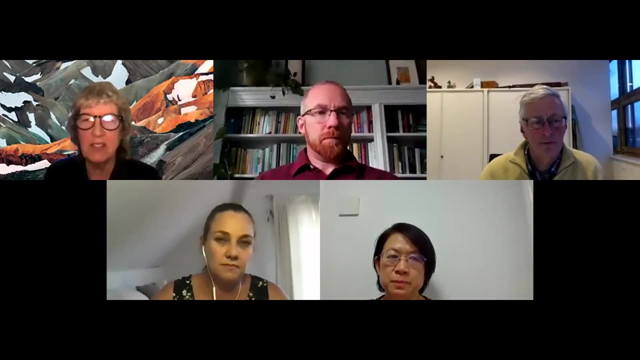 And new tools and techniques for soil health. that I think can provide some of those specifics. So those would be two resources to look at and maybe others can say more about them. Yeah, does anyone else want to add anything just briefly to this answer? Any other panelists? 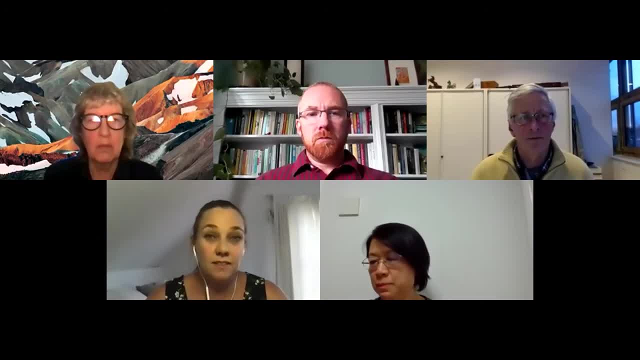 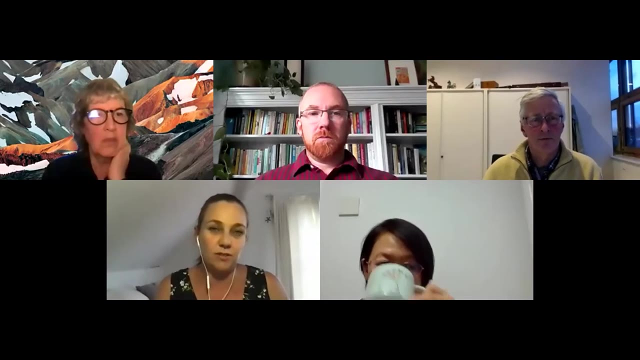 I can just add that I think Lauren's completely right. There's a complete. I'm battling with the same issue And I think it's perhaps at an undergraduate level, in the formation of a syllabus at university level or even in high school, that soil science and soil biology needs to start integrating. 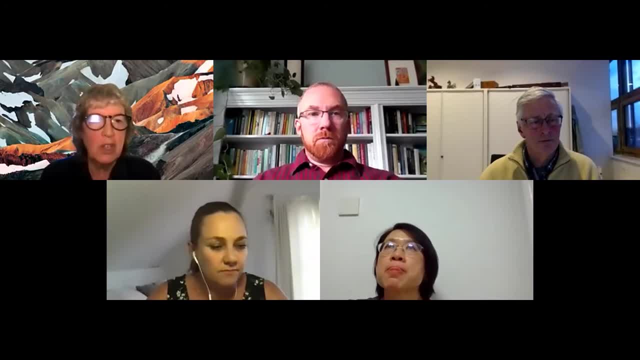 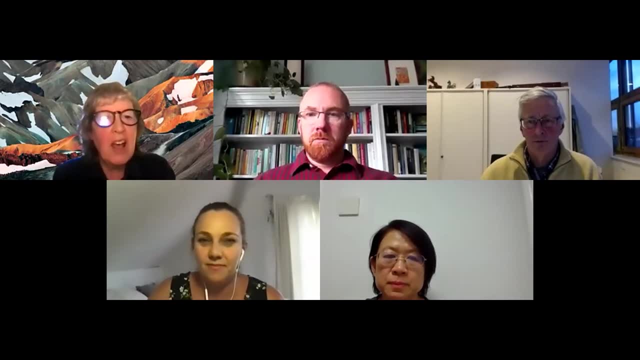 Yeah, Good, Okay, thank you, Charlene. this question is for you. It's about soil taxonomists, So I think it's pretty relevant. How can we reverse the tendency of a gradual lowering in the number of soil taxonomists, as we still face a worldwide problem of taxonomical impediments? 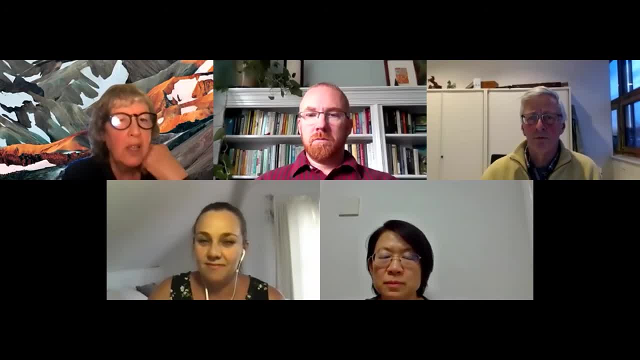 This is from Gabriel Quiraz. In addition, in a time crisis, how can we avoid taxonomists from giving up their research careers due to grant shortages? Now there's specific grants for soil taxonomists. There's specific grants for soil taxonomists that are supported or encouraged by GSBI, for example. 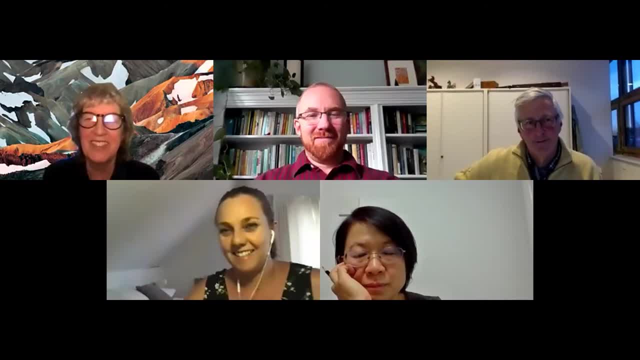 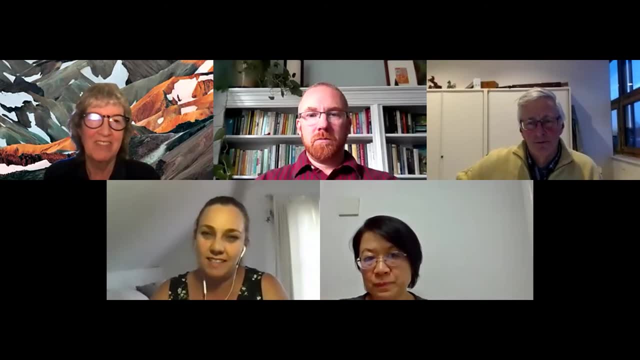 And I know you probably have felt lonely at times. Yes, Bom dia, Gabriel. Good to hear from you. Yes, there's no dispute. There is huge financial implications. Not only soil taxonomists, taxonomists all over the world are battling with pure taxonomy. 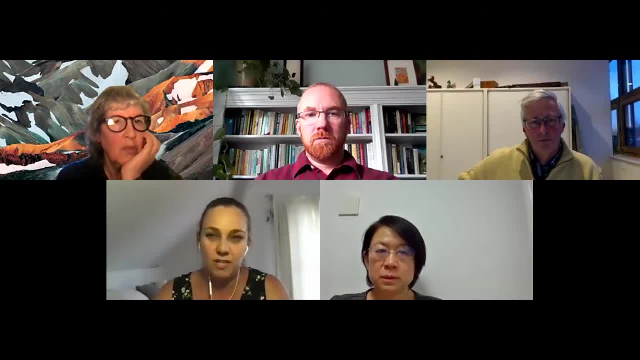 I don't think we can reverse the situation, But we can definitely adapt, And by doing that I mean diversify using molecular methods. Taxonomy can never be replaced- That's a fact, And we need to convince governments and funding agencies that it is inherently important to employ taxonomists. 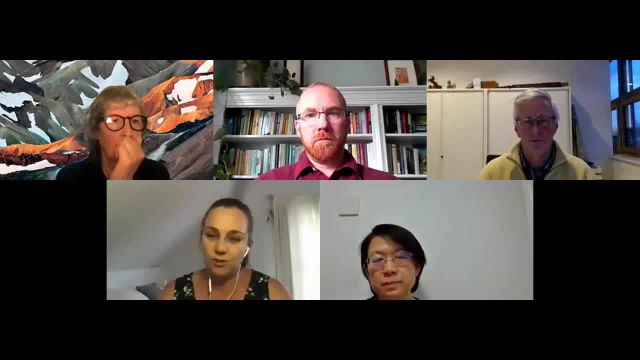 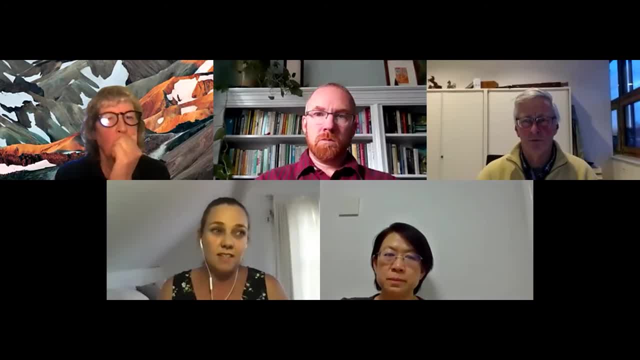 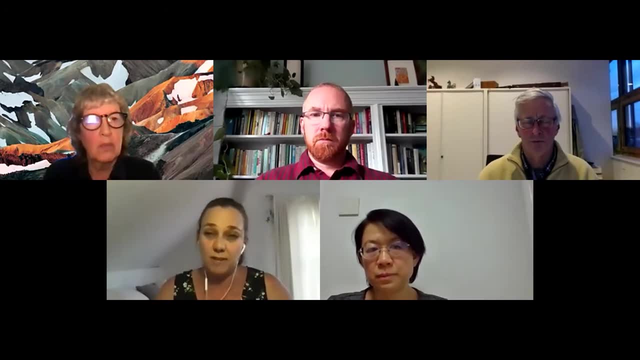 do taxonomy on the side um museums, uh, it actually starts at institutions like museums or or research agencies or collection management agencies. they also don't have the funding. so i think the main message is to diversify, but also just to keep on at it and publish, and publish. 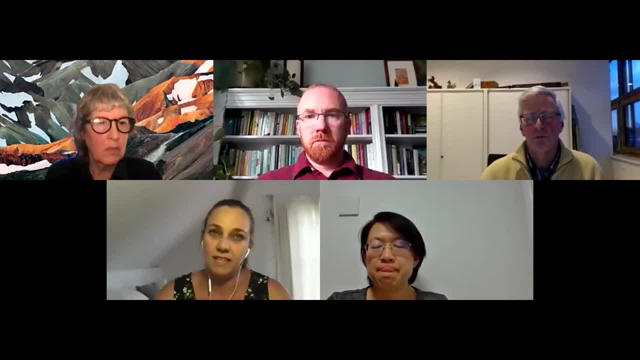 and again collaborate by, by gaining high impact factor papers, which is often the problem with taxonomic work, that you don't really get really high impact work. so perhaps by large projects, collaborating, inviting more other types of people to work with you, i think, is the way forward and 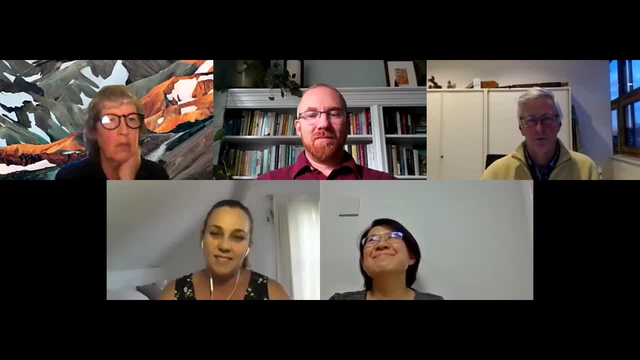 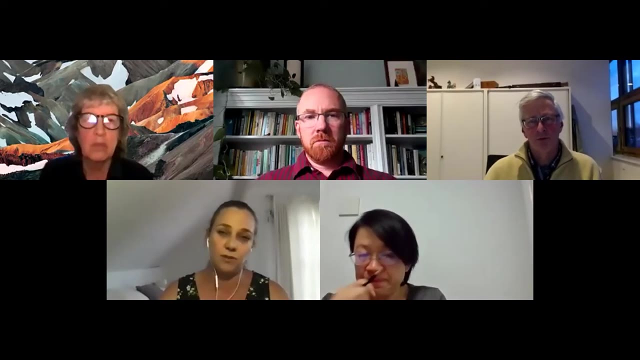 and gabrielle, just don't give up, you will. there will be something, because, um, people do always need taxonomists, and especially, um, if you also, like i said before, promote the services that the soil animals provide and diversifying into other ecological studies. so i hope that helps. 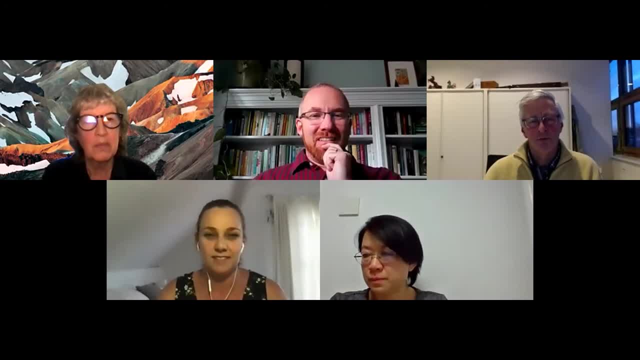 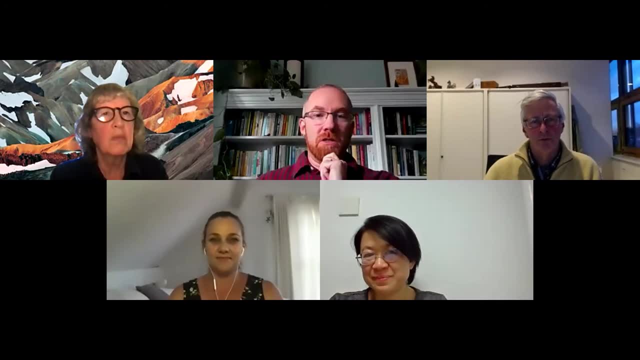 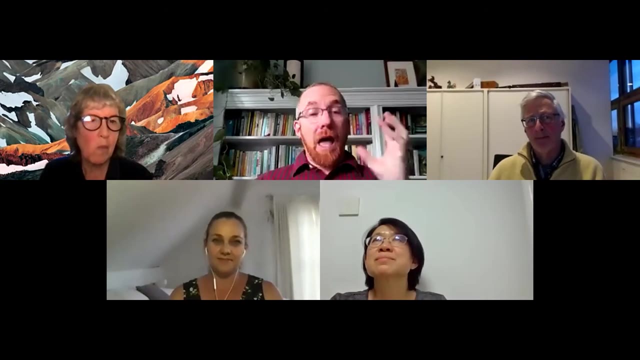 but i feel for you it's a very, very tricky situation. if i could just jump in here briefly because i i love taxonomy: one of my phd co-advisors was a taxonomist and he he really emphasized the value of knowing your organisms and at the whole level, the whole organism right, and that's where 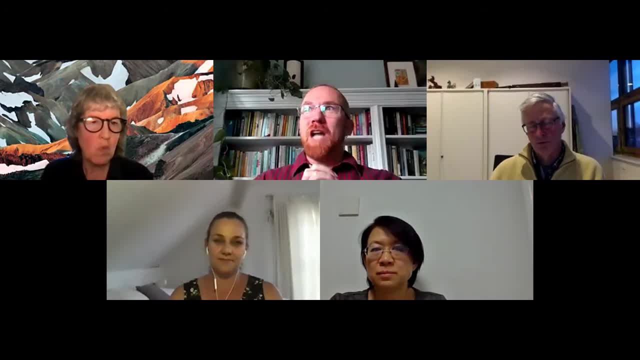 i have done my work. so the the challenge of molecular taxonomy is um is before us and- and there's a lot of emphasis on that- but as an educator i feel confident saying we will never engage students and people around the world in loving soil. biodiversity with dna sequences. 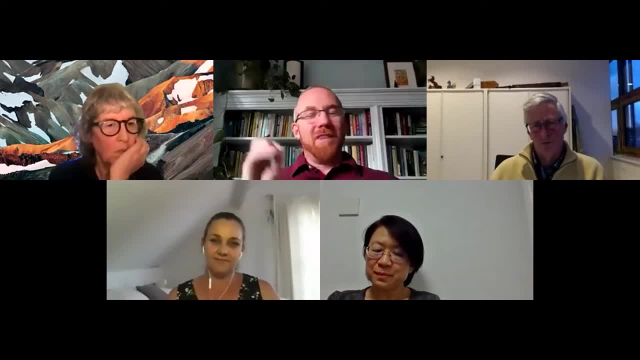 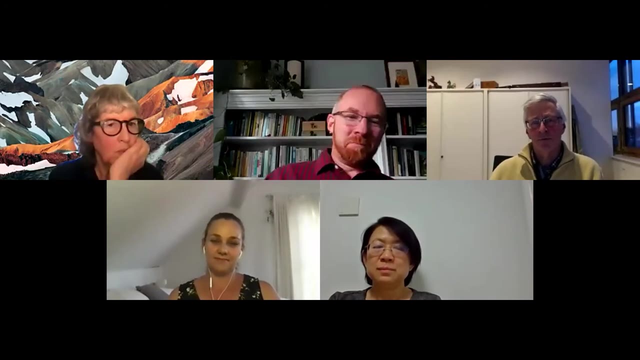 we need to focus on the whole organisms. they're jumping around in a bin before students and under a dissecting scope, so i hope that, um, that charlene's right and that we all will persist and and caring about the whole organism and knowing their names. and can i just add one more thing? it's, it's, um, i find, with my experience with 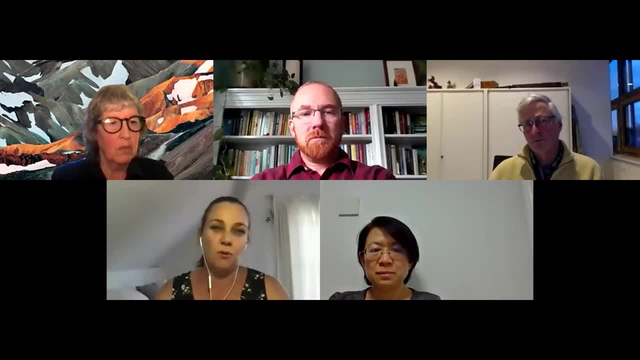 students. they think taxonomy is very old and boring and and it's our job to make it interesting and exciting. and we have the tools. we have scms, we have amazing pieces of equipment to measure, um, how these organisms look under the microscope. so it's also about getting people to. 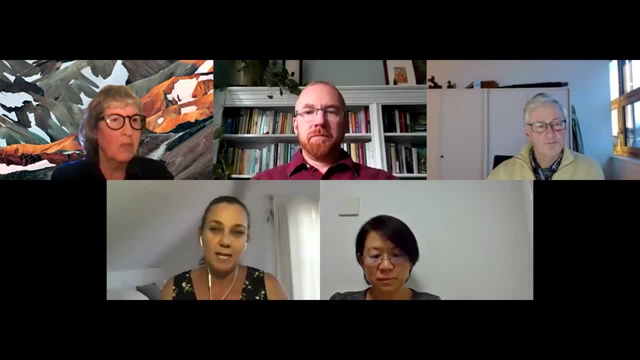 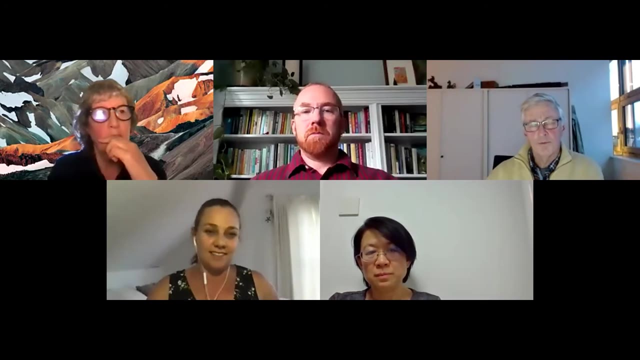 look through microscopes. students to look through microscopes? um, yeah, so you're right, but definitely it's definitely never a replacement. molecular methods won't replace- i hope it won't replace- taxonomy, but it's a very valuable tool to aid in um identification. great, thank you um you mentioned. this is from carlos guerra, you mentioned in your 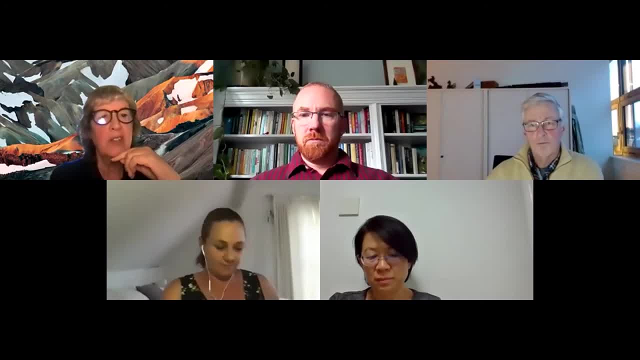 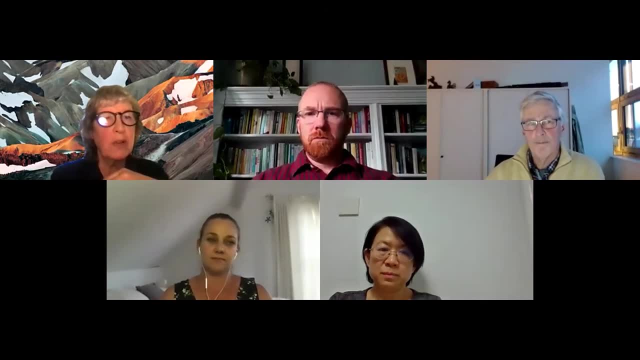 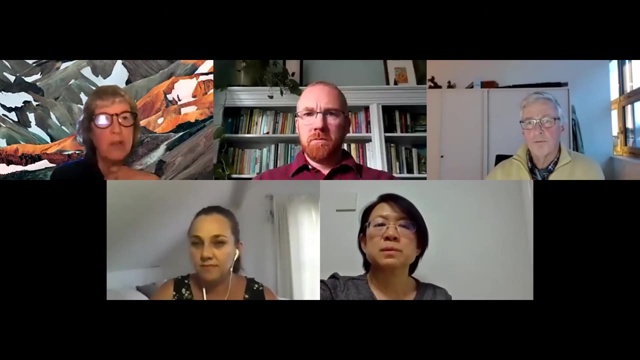 bucket list the need to go beyond what we have, focus on understudied continents, ecosystems and access, and one take a wider group of soil organisms from microbes to macrofauna. so the question is in the recently formed global soil biodiversity observation network and its collaboration with glossolan. 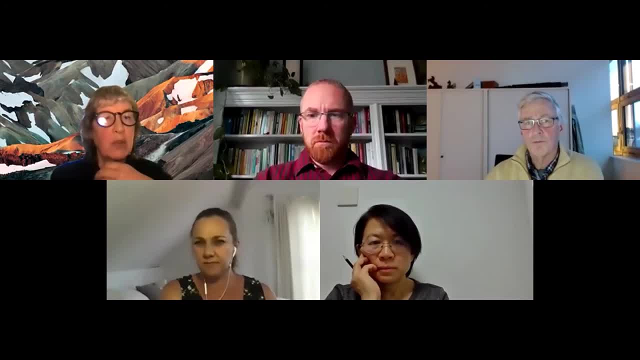 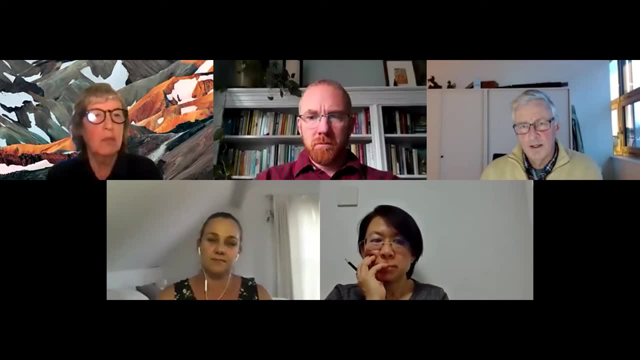 gsp fao a good. is that a good step in that direction, or what do we need more to do to achieve this goal? yeah, it's a. it's a nice question. um, i don't know exactly how the network sites are distributed across the world. um, i've been thinking about this from. 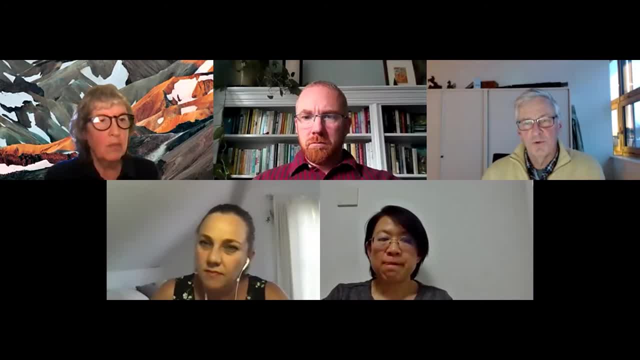 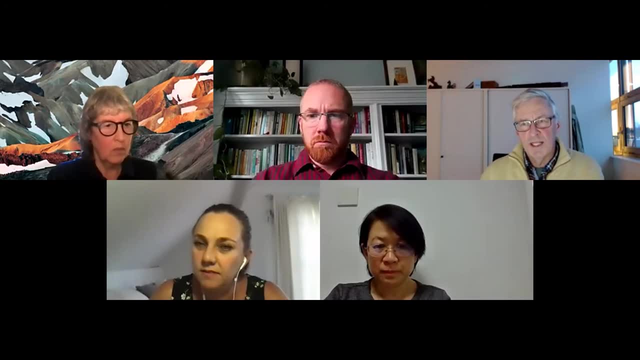 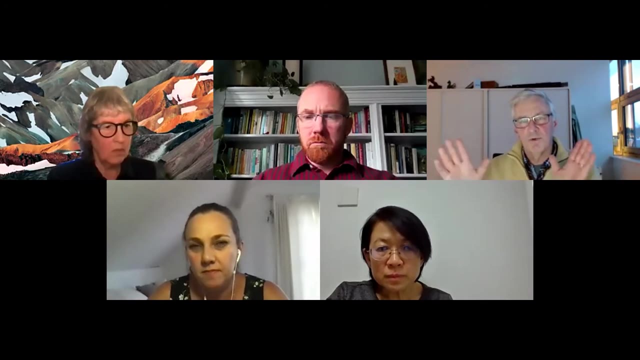 well, so this could be a good stepping stone. first of all, but i've been thinking about so, if you have to sample, if you have to to lay out the sample sampling design, then what is the first step that you can take? you can just, for example, do everything random, or you can do a stratified 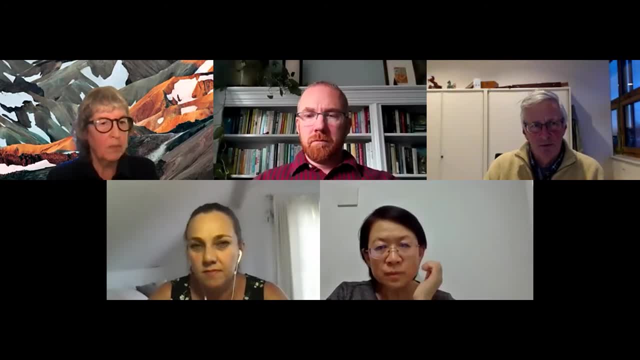 random sampling. so i've been talking about this with people from israq, which is just across the road, which is a soil information organization here, and i've asked him if he would stratify the soils of the world into units that can be considered for sampling. how would you do that? i'm still waiting. 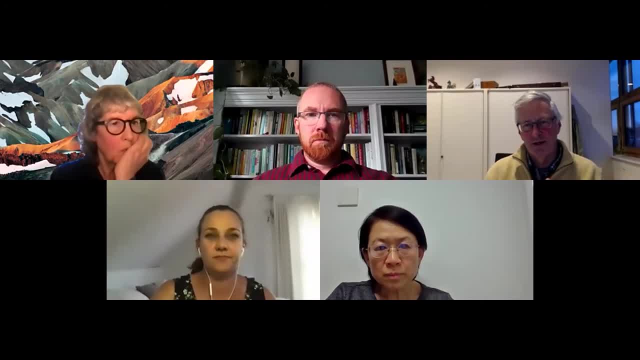 for the answer, but that would be another possible step and maybe you can combine the two so you have this observation network. i don't know where the observation points are and and how they were just chosen, but, um, actually, if it, if it, if i could just start from scratch, i would say: let's look at the 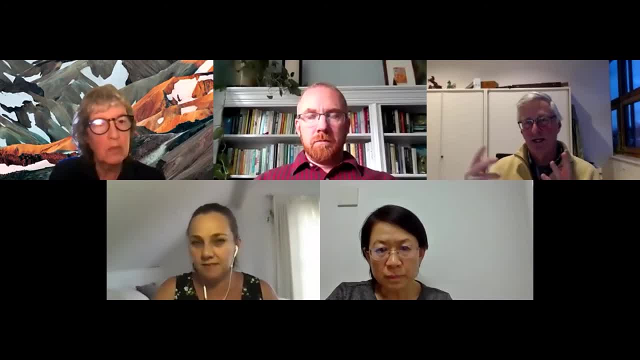 soils of the world, the vegetation types and climate conditions and other factors that need to be considered, and then just lay out the sampling design and then see where we have to take the samples and to identify them and then maybe there can be sort of partial overlap with a 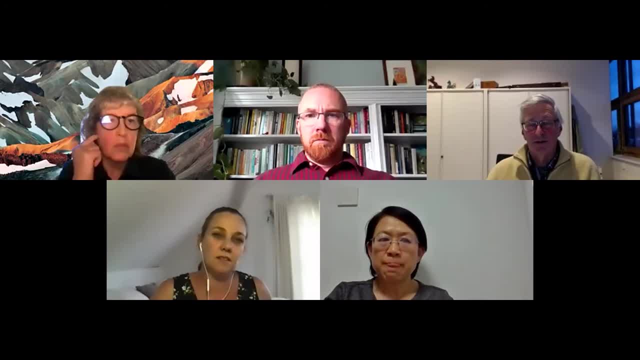 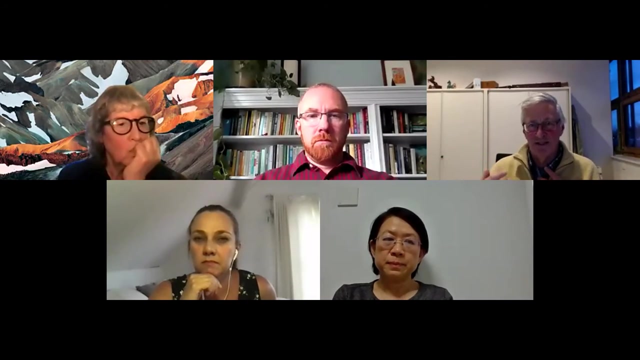 closer land and then we should use that, of course. and then, coming back to the african situation, so the person who said, well, i have few, i have little possibilities or a little, i don't have much funding or so. so for many of the questions we are looking for people who are just in parts of the world where we don't have much access to. 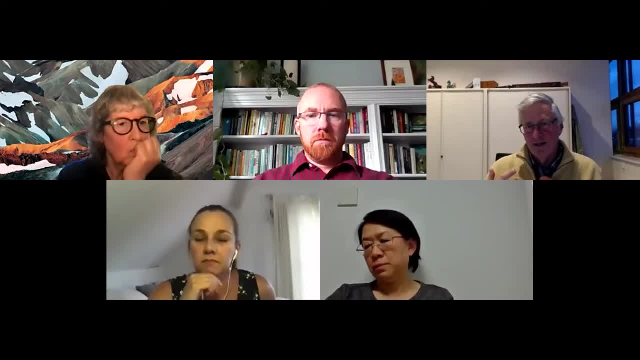 and if you register for the global soil biodiversity to become a member of the global soil biodiversity initiative, it's for free. the only thing that you need to do is to put up your name on the list and then, if we, if we're going out for sampling or for 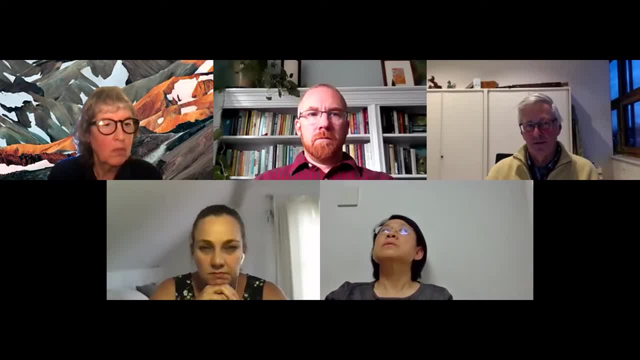 activity. we at least can find you, and that that's so very important. so we need to to be able to locate the people so that if we go out for sampling or for large sampling programs, that we know who is where. great, thank you. so, uh, john ling. uh, there's. this is from michael or chavo, very interested in. 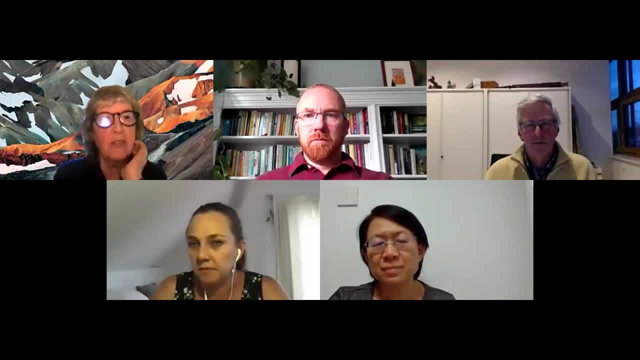 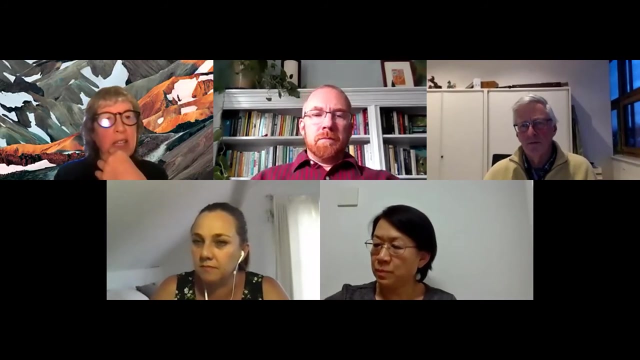 rich studies, researchers, how? how do we package the findings of um soil, biodiversity and agricultural systems and present them to the farming communities where most of the action and interaction with soil actually is happening? and and how can we emphasize the close relationship between soil biodiversity and and productivity, the things that farmers, immediately, you know, are looking for any? 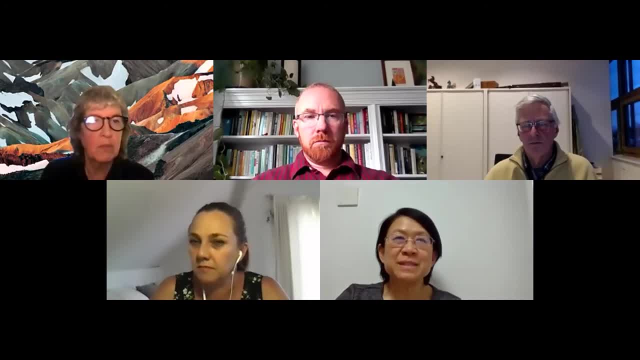 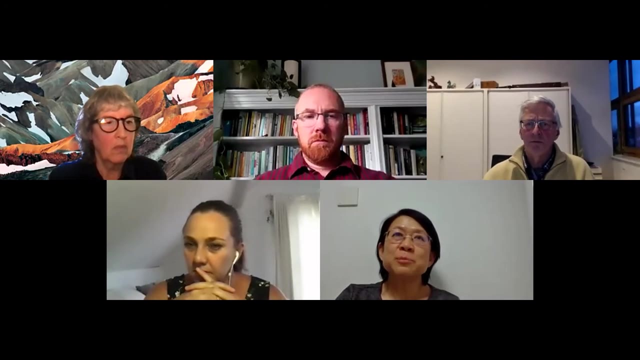 thoughts on that. yeah, this is a very good question. i think that, uh, at least here in china, what we do is that we have small farmers and then we have cooperative farmers. there they have bigger lands. so for those small household farmers, they're actually they're, they're very smart, they know the their crop very well, they know that their soil is. 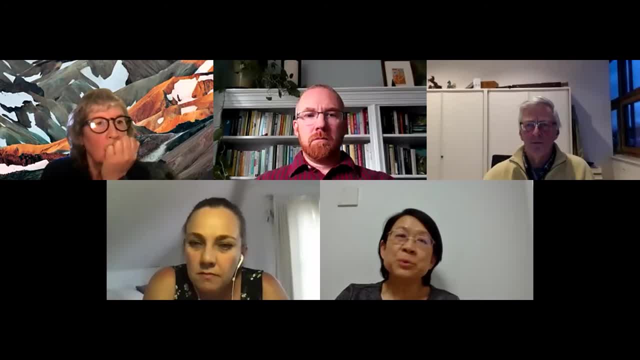 sick or not, it's healthy or isn't unhealthy. so what do we do for the small household farmers right now? is that uh for um each cropping system? in our lab i said for for the uh each cropping system. so we try to establish a correlation between uh so pathogen abundance of soil passion with crop yield or with the disease. 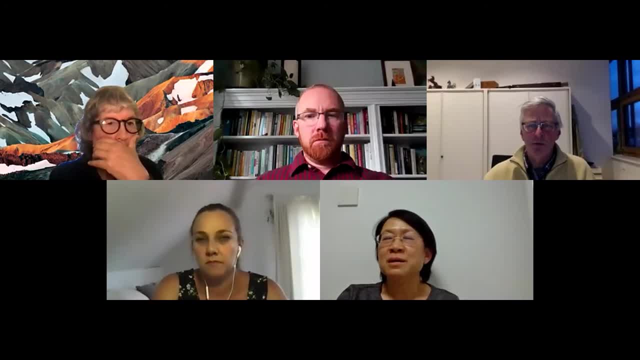 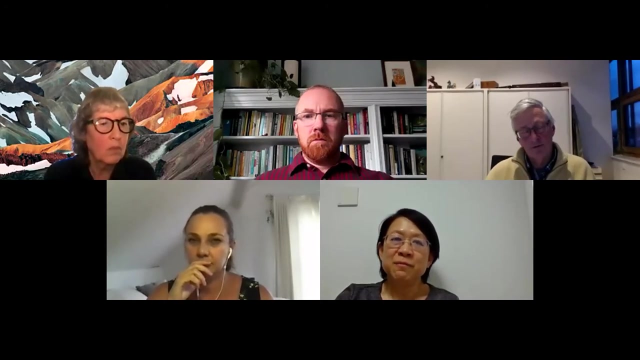 incidence so that it can be a early indicator, or it's like earning warning indicator for for the conditions, for the soil conditions, to indicate whether it's a potential uh damage to their crop. um, but for the for the small farmers, um, it's difficult to do sometimes, but for the club cooperative farmers, they are willing to do it. so 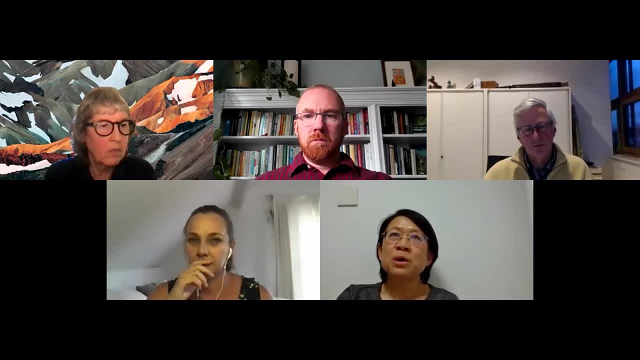 they kind of they're, they want to know more about this soil. they send out their samples to the lab. um, so we, we kind of work closely with them and even some of the- uh, the collaboratives. they have their own lab so we teach them how to, how to do such kind of tests. um, yeah, so i think that's um. 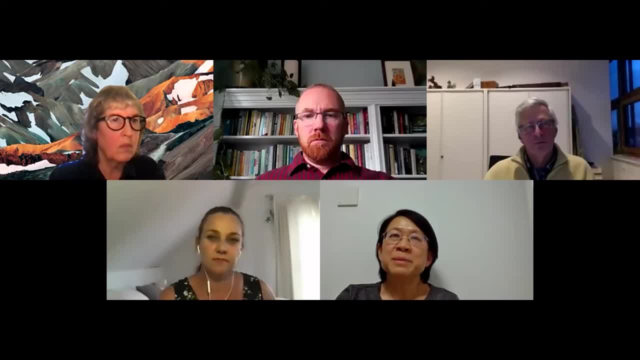 as scientists. you may need to um, because here in china agriculture university we have the advantage that we establish kind of um, which is called um, a science technology backyard. there the students, they, they stay together with the farmers, they work together with the farmers, they know what's happening in the, in the fields. therefore, those 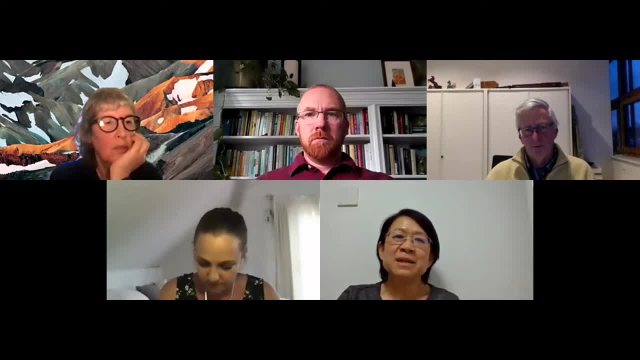 kind of problems: feedback to the lab and we do the science in the lab and then the science will be trans, easily trans, transformed to, transmitted to the, to the farmers. so, uh, i mean, uh, basically it's do that the scientists really need to get close to the farmers, to the growers, and 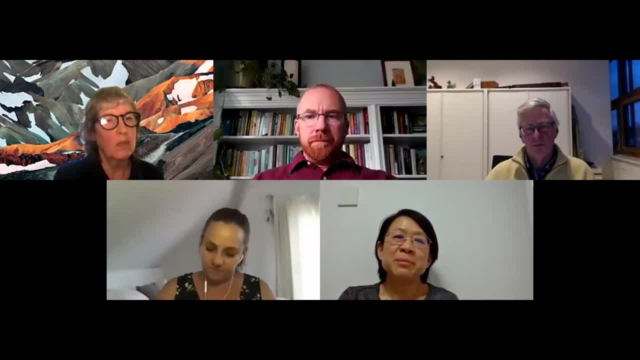 then you know what's happening in the field and then you come back to the lab and then do some scientific work and then those knowledge is easy to be transmitted. So I think that what we can do in the lab is to help them to recognize the problem and to find the solution. 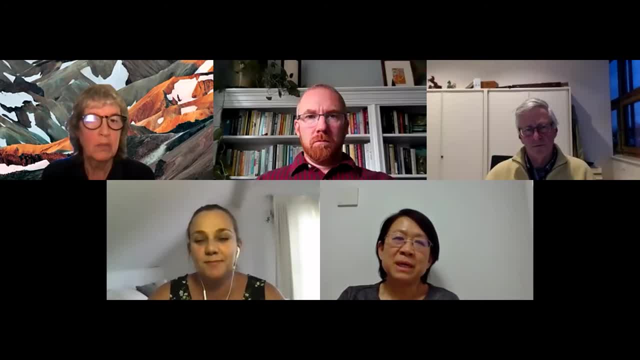 for them. By doing so, then we can help the growers to optimize their management on time. Let's see. Do any other panelists have anything to add to that from your own country's perspectives? Okay, So, Lauren, this is like the burning question. 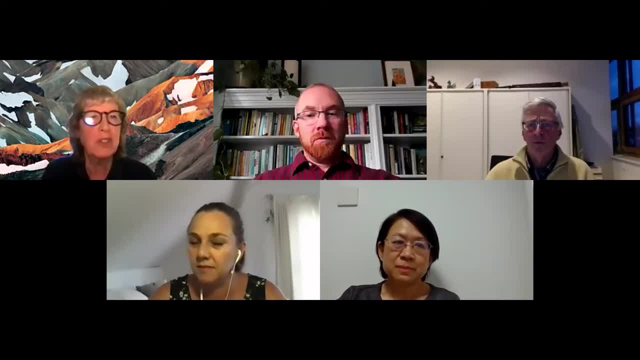 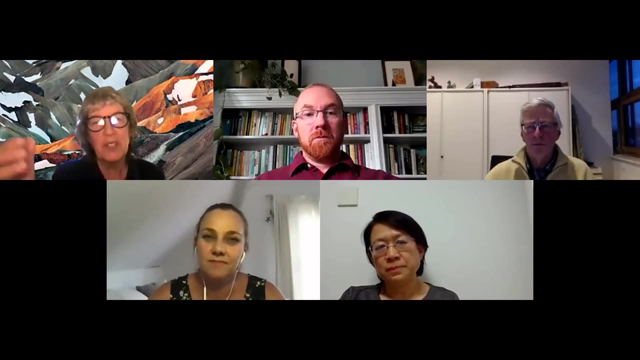 But it question- it'd be interesting to hear about it from your perspective. Soil biodiversity is important- How to integrate soil biodiversity, the knowledge of soil biodiversity, with the ecosystem services that they provide, And not necessarily, maybe from a research perspective, but anyone is welcome to contribute to that. 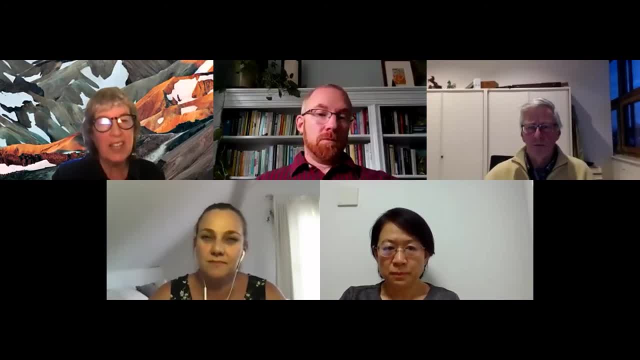 But maybe in the outreach and education, because it seems like that linkage is extremely important And any thoughts about like developing that and is that like a necessity when you can make that link, will then people come to appreciate that actually there is something underlaying these processes that we value. 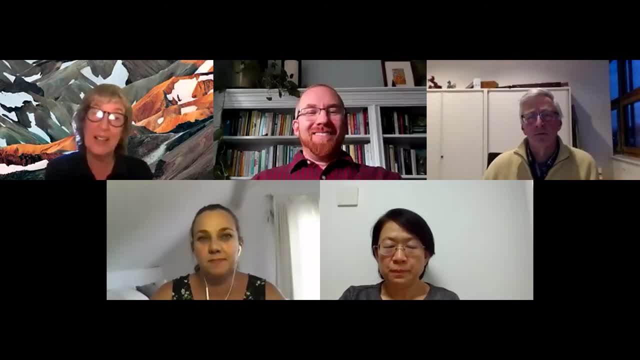 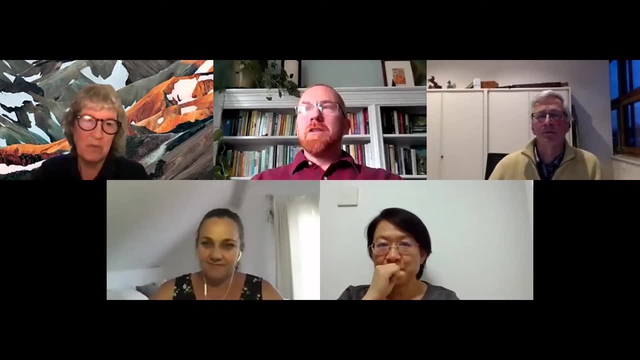 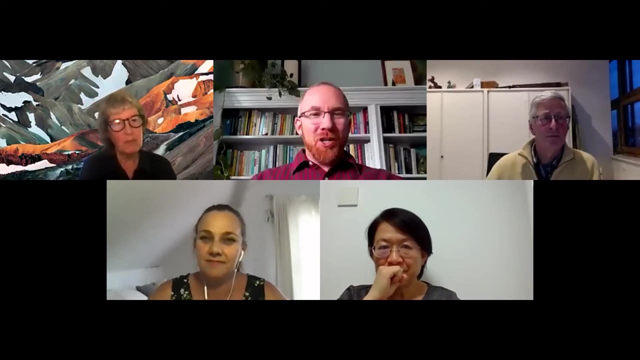 these functions and services we value? Yeah, any thoughts on that? That's a tough question. As I let it incubate, I'll just say that I think ecosystem services are a very powerful idea, Like Charlene said, the Millennium Ecosystem Assessment. 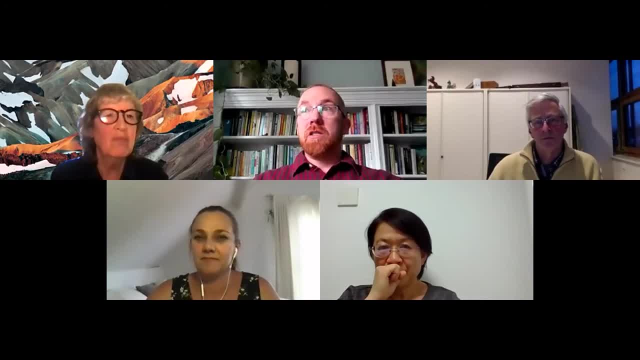 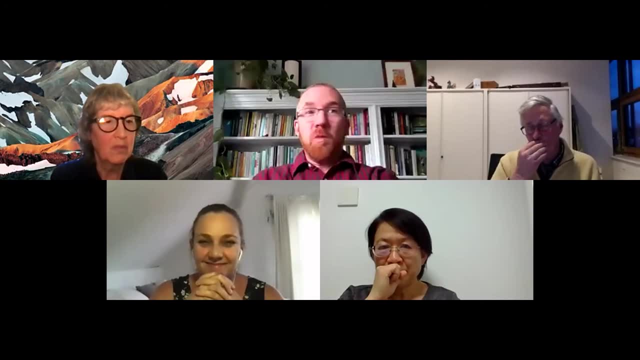 was kind of a transformative document for me. I actually still use it in many of my classes. I say to the students: it's a little dated perhaps, but it is one of the most important documents of the past hundred years And I require that they read an excerpt from it. 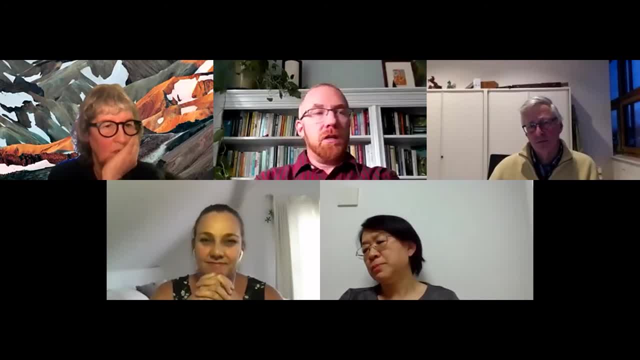 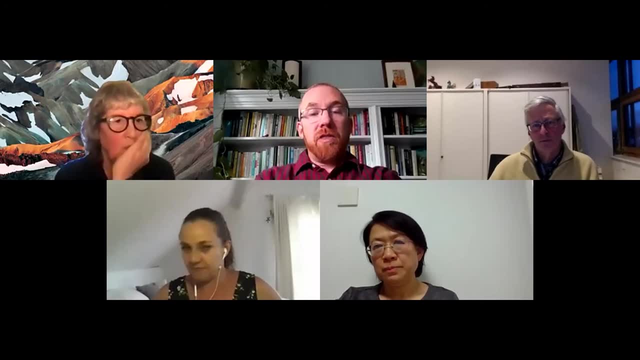 There's some debate about ecosystem services in the literature and how powerful it is. What are the downsides? And I love to engage in that debate but I do use it. So I do think it is an important educational concept And I actually start my soil ecology class with it. 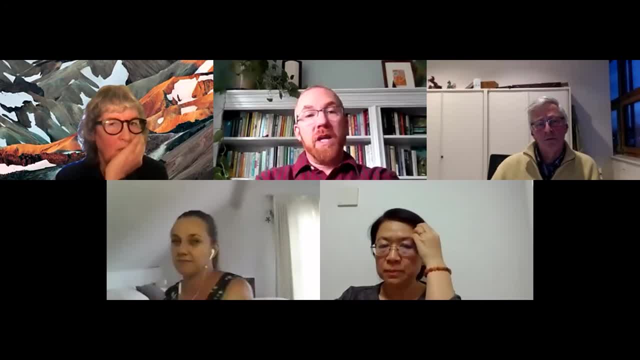 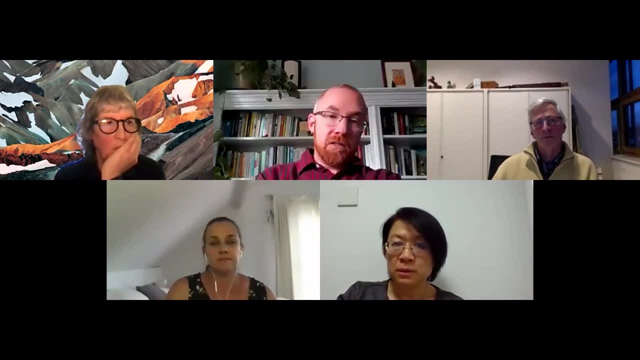 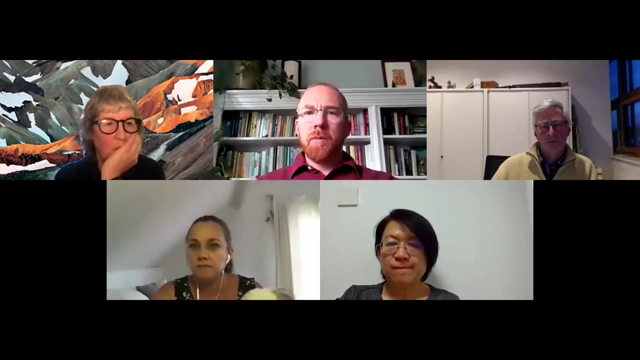 I say to students on the very first day: let's brainstorm. why should we care about soils? And that is the entry point for talking about then the biodiversity that provides the services that we need. And there was another question earlier- I don't know if we really got to it- about. 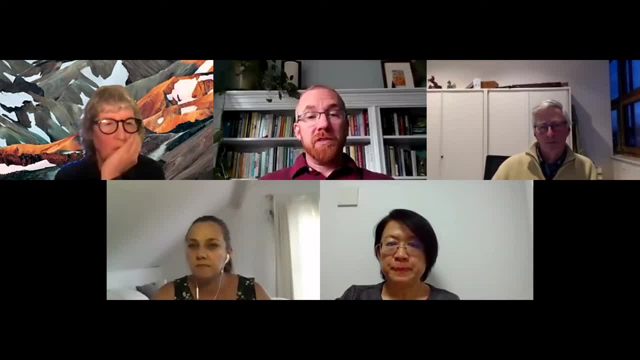 integrating soil biodiversity with other ecosystem services, And when you think about what soils and their biodiversity do for us, it is often about non-soil things. It's about carbon dioxide in the atmosphere, It's about water flow. It's about growing the plants that we see above ground. 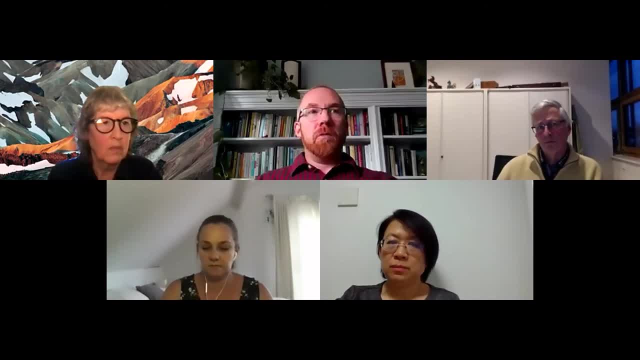 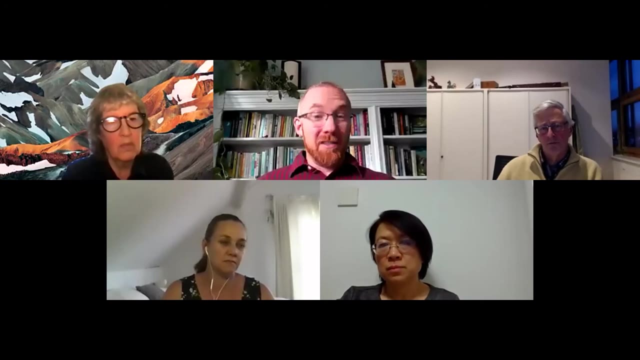 So I think there are ways to engage people with where they are in their communities. Are they worried about flooding? Are you talking to a group that's worried about climate change? Are you talking to a group of people who manage lawns and turf grass? 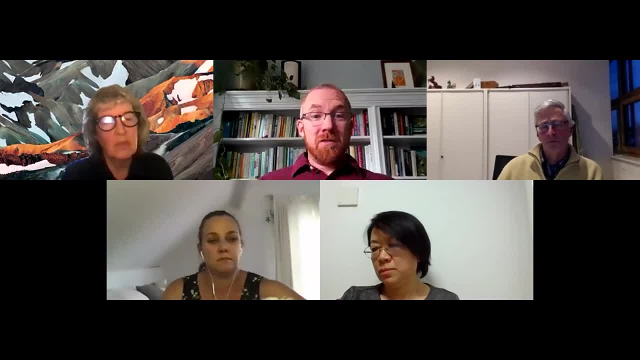 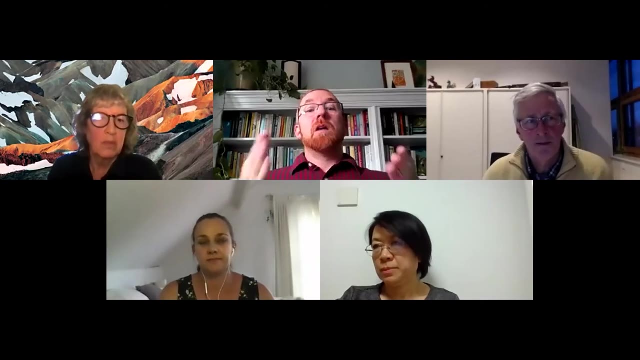 And certainly in the age of a pandemic, health concerns in soils and pests and diseases that can be suppressed by biodiversity- All of those are ecosystem services in that framework. So I think, opening the dialogue with ecosystem services and then making the very clear direct link to the essential nature of biodiversity, 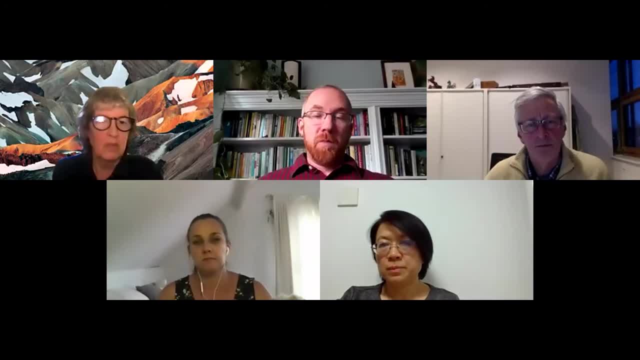 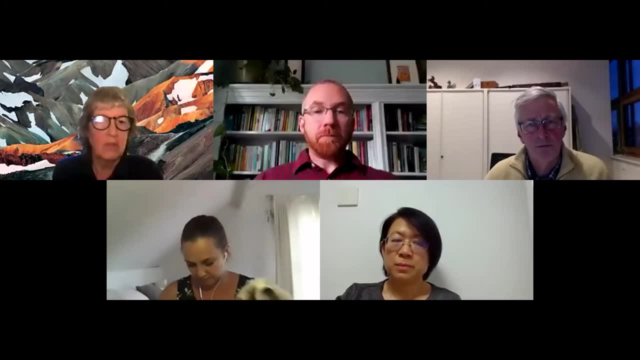 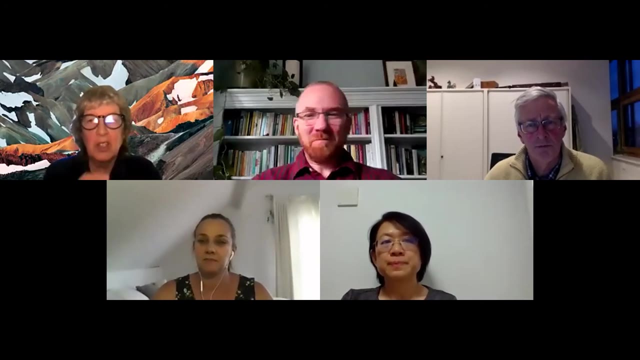 providing those services is really a powerful way, especially for policy makers And as I've seen in my classes with students who do care a lot about human wellbeing and sustainability. Great, thank you. Hopefully that's what you were looking for. Thank you. 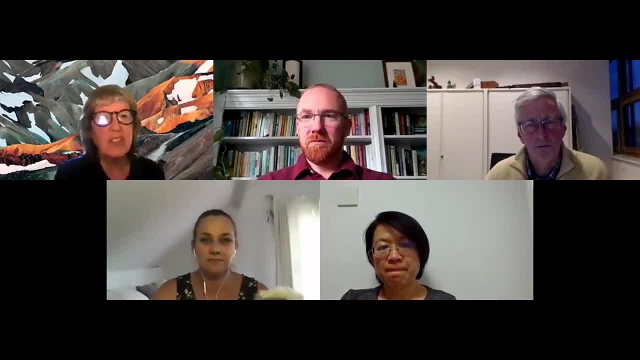 Charlene, in agriculture we have growers advisors, who are very interested in management practices that optimize conditions, For example, if you're looking for a beneficial soil microbiota- but there aren't great methods to share with them to assess if their management practices are working. 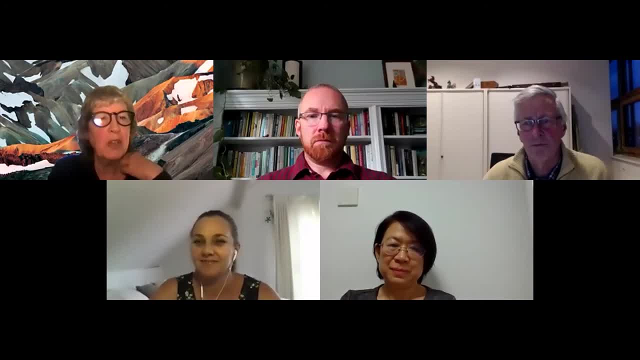 And if this isn't a good question for me, just for you to let me know. But as a community, have there been efforts to link our approaches to understand microbial ecology- but maybe not just microbial as well, fauna as well- to soil testing labs? 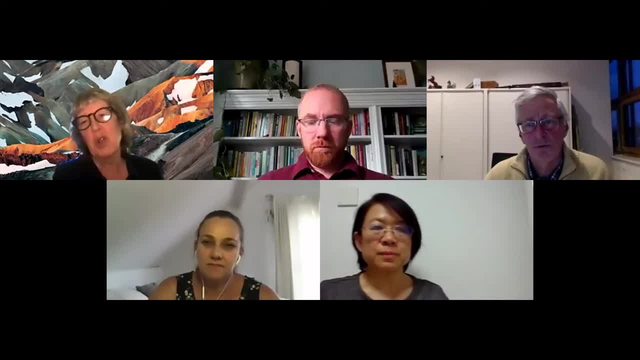 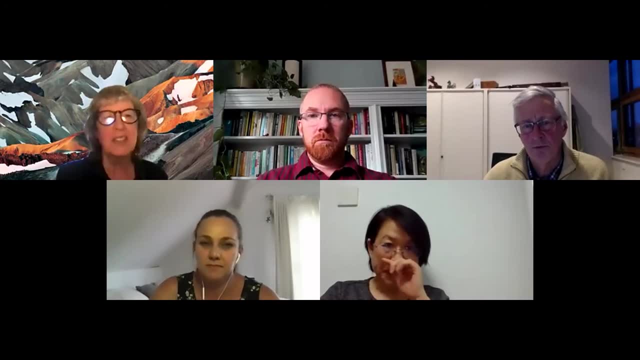 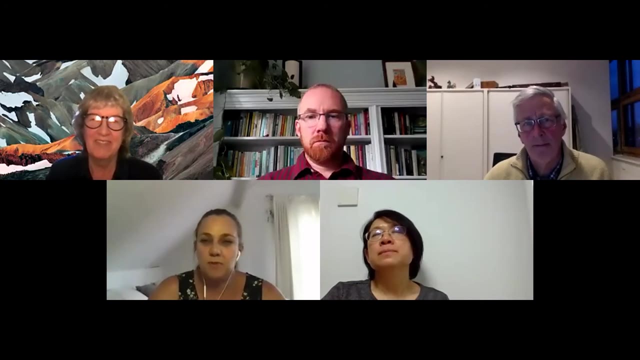 to offer better support for these growers. I guess it's providing access to tools so they can assess whether or not there is something good coming from these changes in their management practices, If you have something to say about that. Well, from my experience, there are more work- 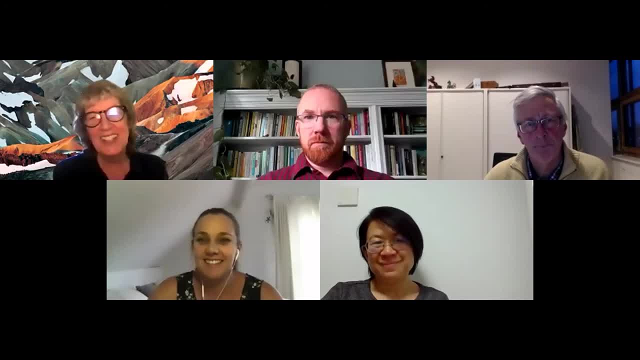 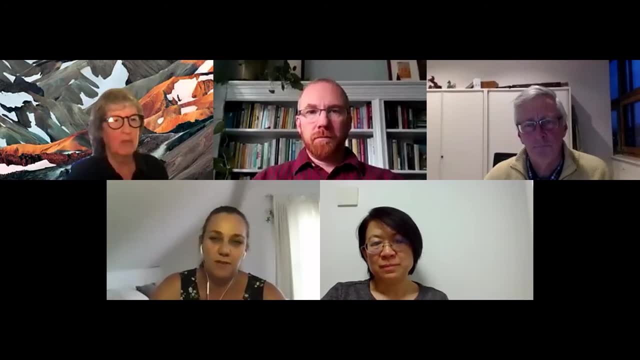 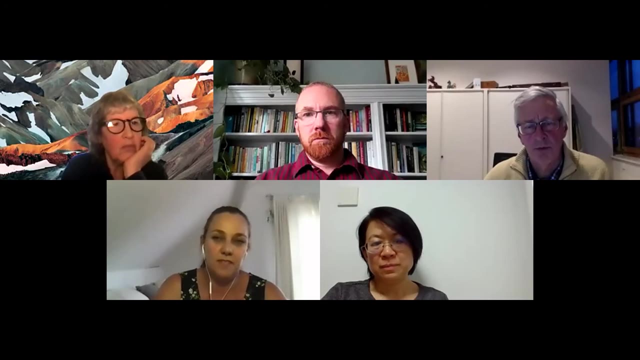 Lauren Hale ask that question. I'm sorry, Lauren Hale. Okay, go on. Thanks, Lauren. From my experience, there are methods, of course in here. farmers will send you know, they'll send you know a sample to a lab, for example, to test the bacteria. 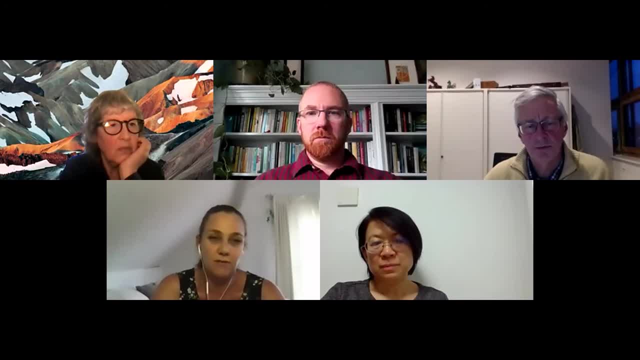 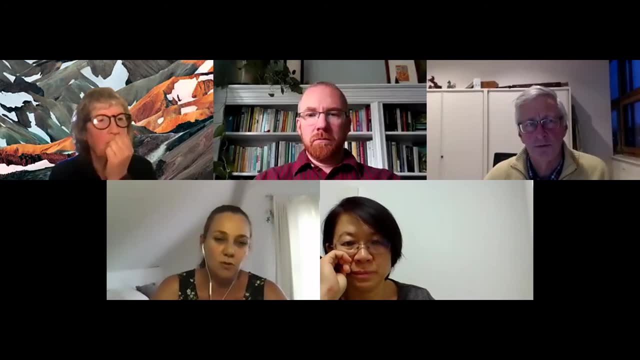 or the nematodes. our nematodes are very well known, of course, and very well indicated For other groups. it's not so easy. I always- for example now with Calembola- we're not even sure if we have invasive species. 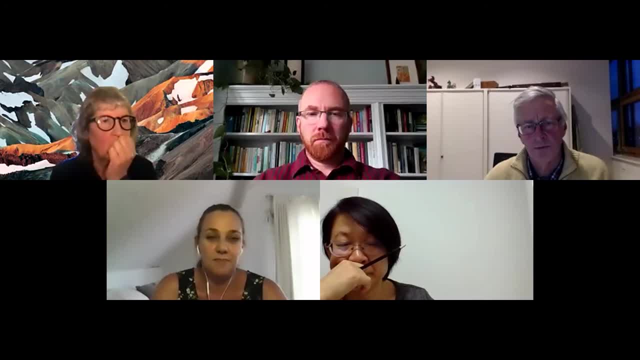 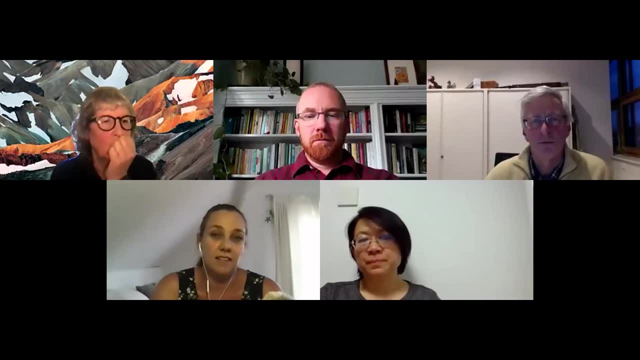 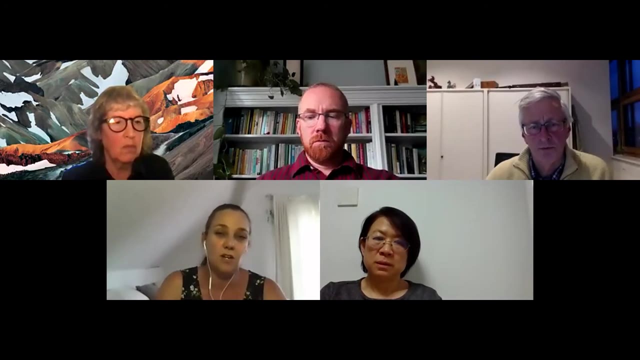 or indigenous species, which is really tricky. but I always find that the measure of diversity can really help a farmer or a landowner to see how healthy their soil is. So, for example, very degraded soils might have just one or two species of Calembolans or other taxa. 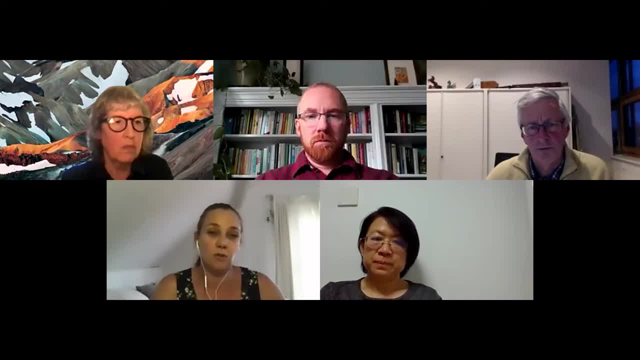 while very healthy soils that have built up the soil organic matter they can actually see in a tray where you show them by sifting leaflets that they have spiders and centipedes and Calembolans and pseudoscorpions and that's sort of. 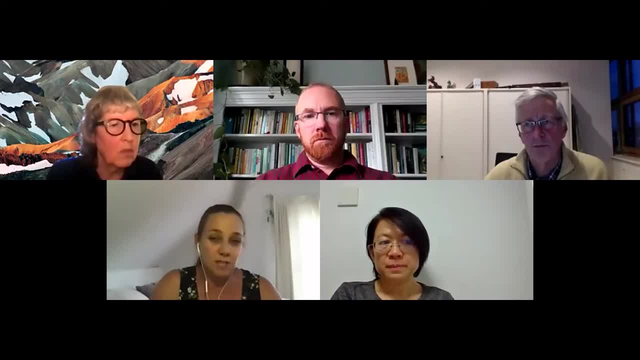 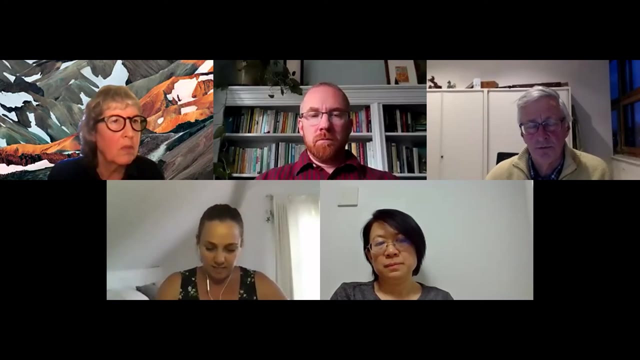 been my approach with landowners to tell them: go have a look, go look at your organic matter, go look at your soil. But in terms of a bit more scientific methods, there are ways to. there are some tests and I'm sure some of you actually have it here. 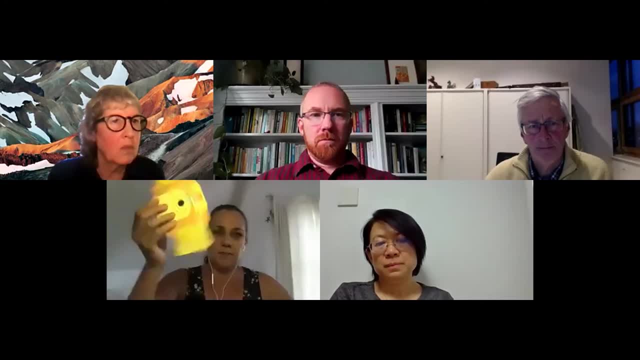 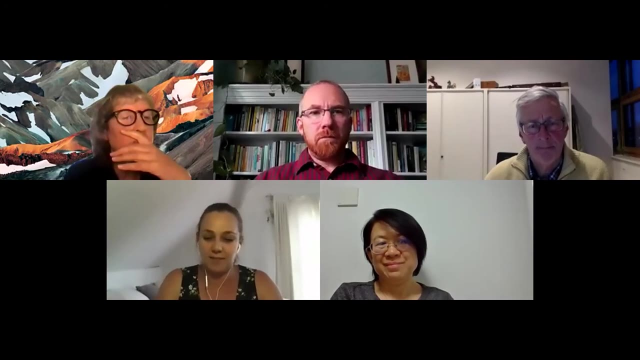 they're familiar with this fold scope- I'm sure you all know it- where you buy this little microscope, and this is a way we're trying to actually give farmers tools that they can use to, because farmers, all farmers- are scientists really. 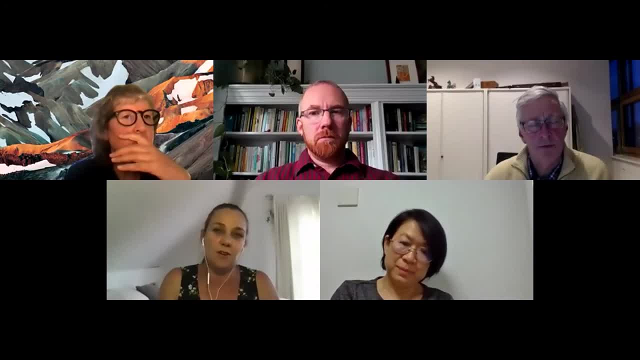 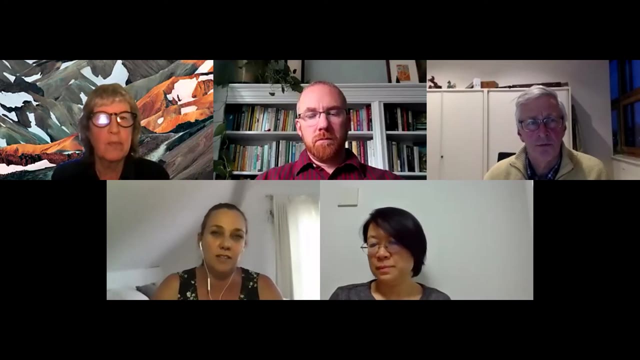 where they can look at their soil, look at the microbes in there, find any tardigrades. So I think it's just enabling people with the right tools and definitely the right knowledge in their language to appreciate if their management system is making a change. 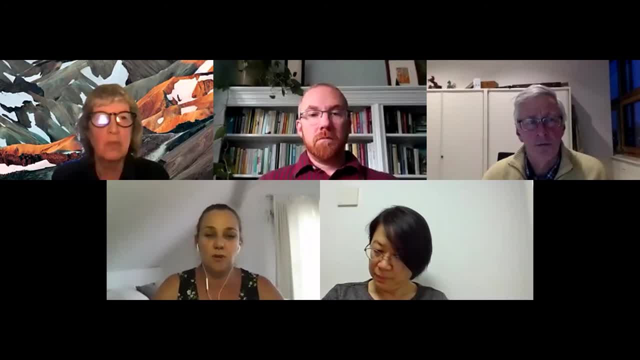 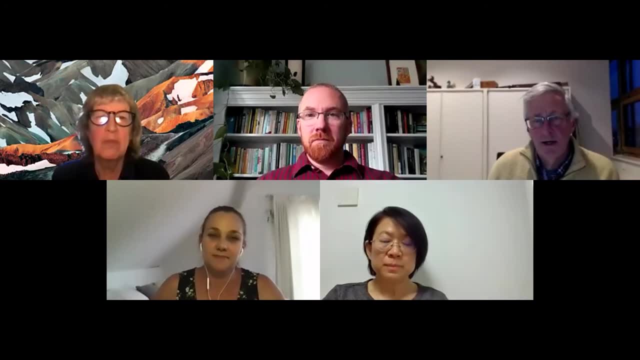 I don't know if the other panelists might have a bit of a more contributions. I think there are some. maybe I can add something there. So I fully agree with you, Charlene. And another thing is that for more than 25 years, 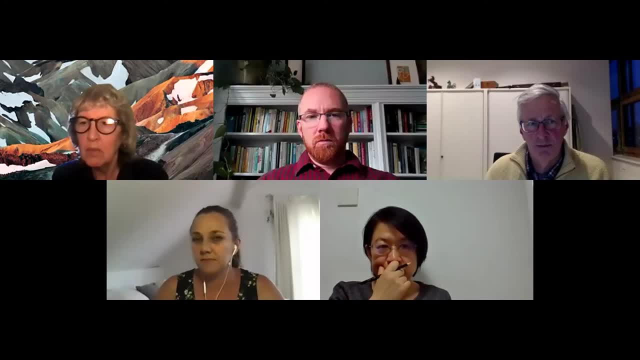 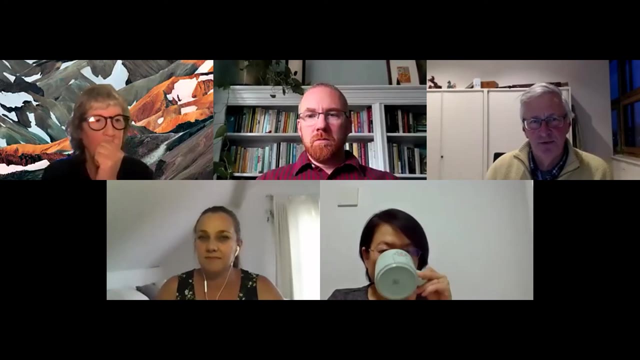 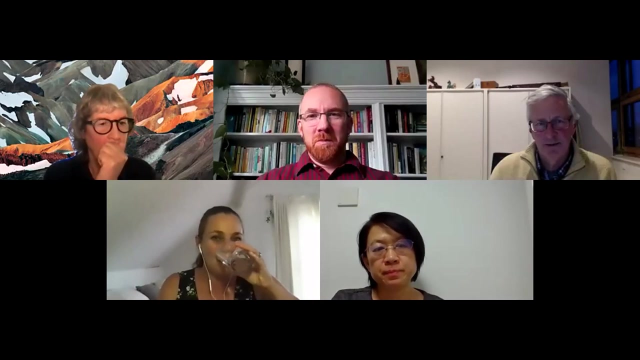 people have been wondering whether there are indicators for soil biodiversity And I'm quite pessimistic. I think all this searching has not really worked out so that it delivered an indicator. If you ask a nematologist, the person says. If you ask an earthworm person, the person says earthworms, and so on and so on. 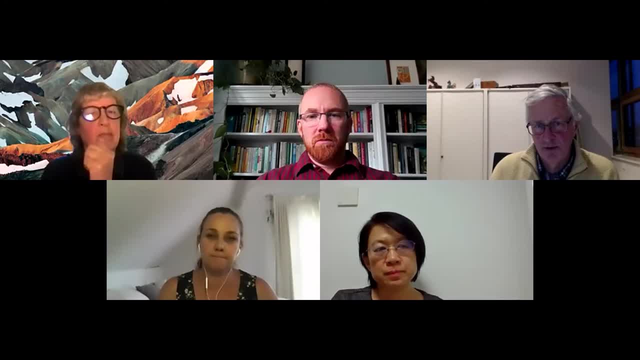 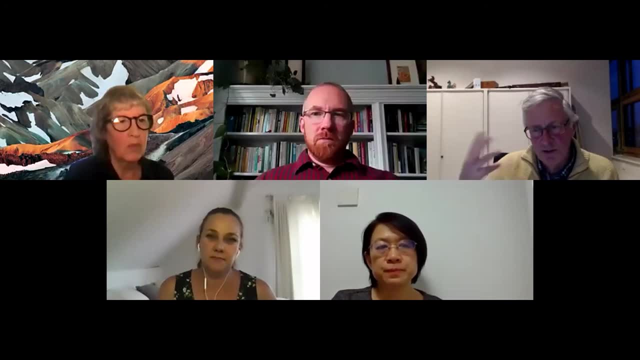 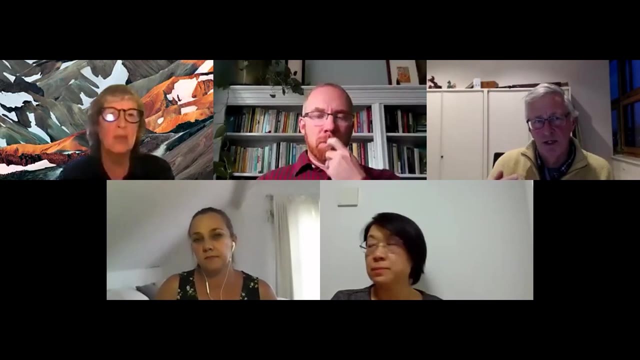 And if you do a full soil biodiversity assessment over soil, that is really very expensive. It's far too expensive for a farmer. So one of the things that I'm sort of playing with is that maybe it's better that we have a good scientific understanding of what sort of land uses and vegetation cover and soil. 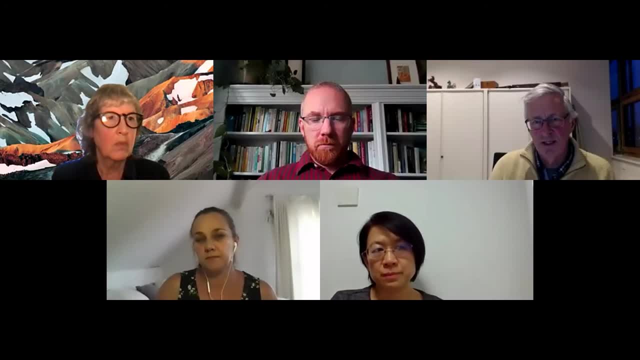 management what that does for soil biodiversity, And then you can sort of show what action perspectives are doing for soil biodiversity And then you can tell farmers, well, if you have this or that action perspective, then your soil biodiversity will most likely look like such and so 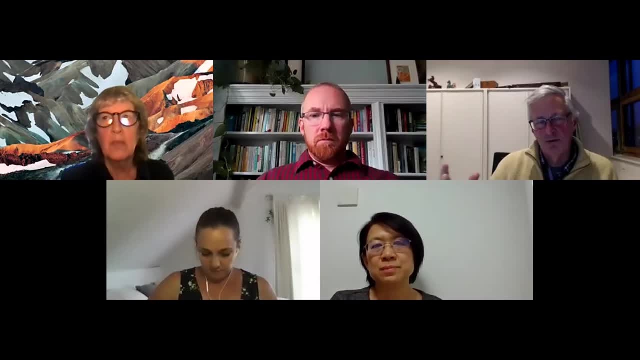 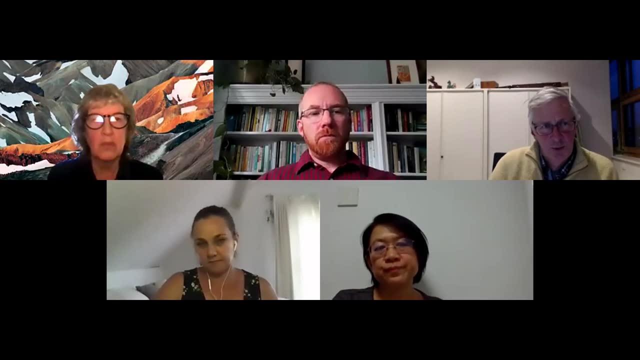 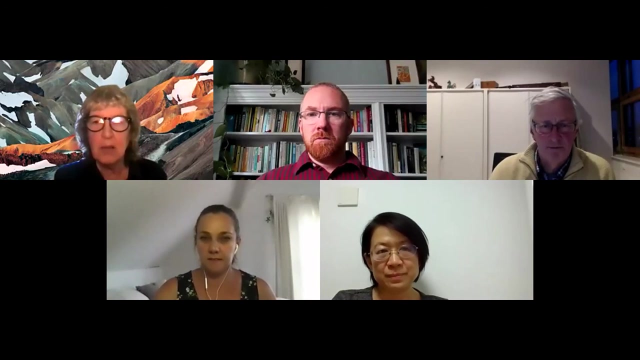 So maybe that is something where we can go around the real complete identification of all soil biodiversity but sort of make a shortcut For what it is worth. Okay, So I want to just note that we have three minutes left in this panel And I wanted to also make sure the audience realizes that this is being recorded and will. 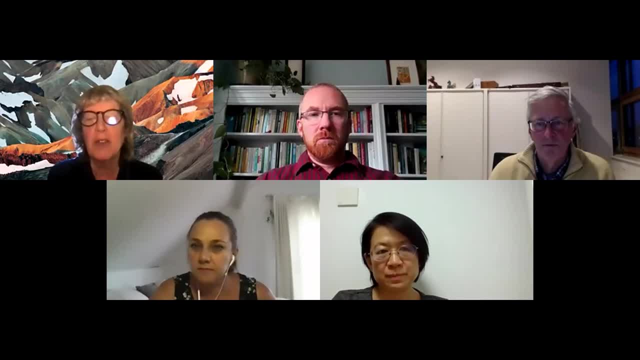 be available at the GSBI site to view. if you haven't been able to see the whole thing, I guess there's one maybe sort of integrative question here. It's from Ladislav Mikko that talked about. you know the disappointment in trying to. 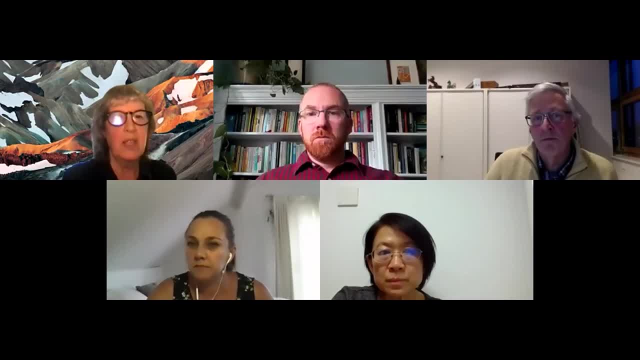 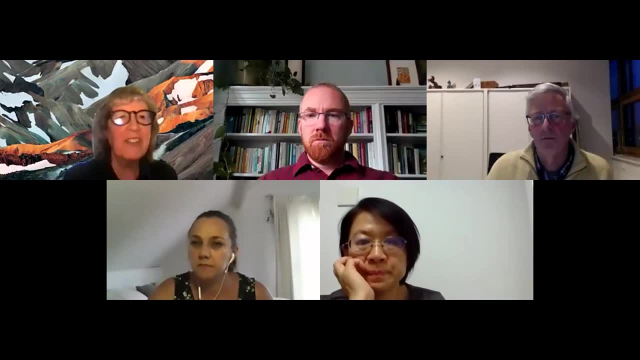 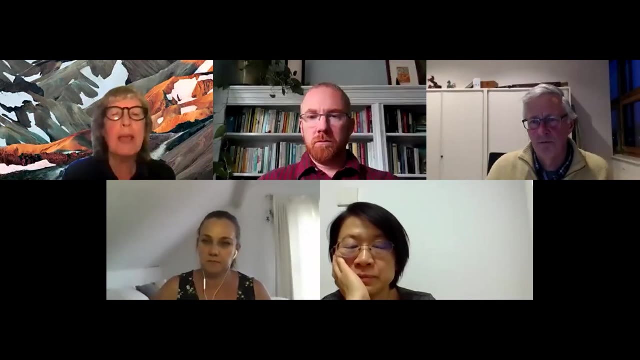 get the soil protection strategy in the EU and that failing, And so he's wondering if a new attempt is made. can the soil biologist community be able- now, you know, and perhaps with this report- be able to- and this is more than 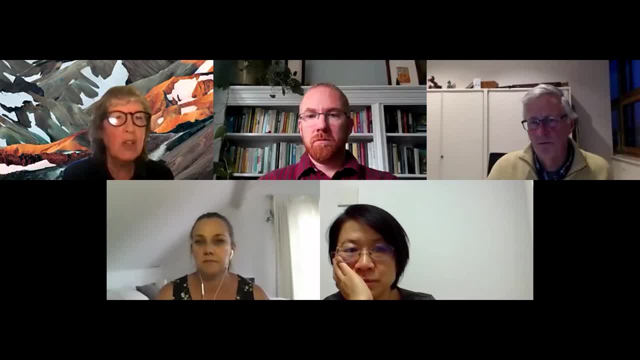 EU. I mean other countries as well. Could we communicate at the national level to get support for a broader initiative to protect soil and thinking that perhaps demonstrating linkages of soil, biodiversity, ecosystem services and economic impacts might help? Any thoughts on that? 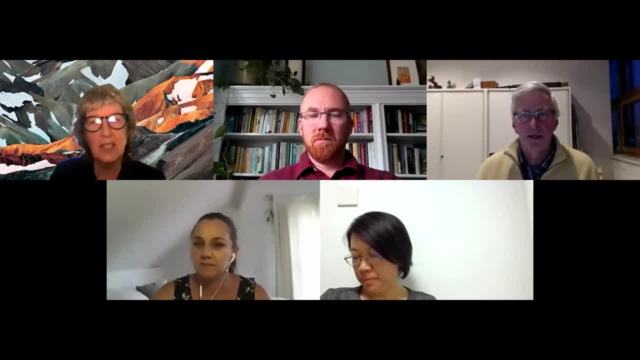 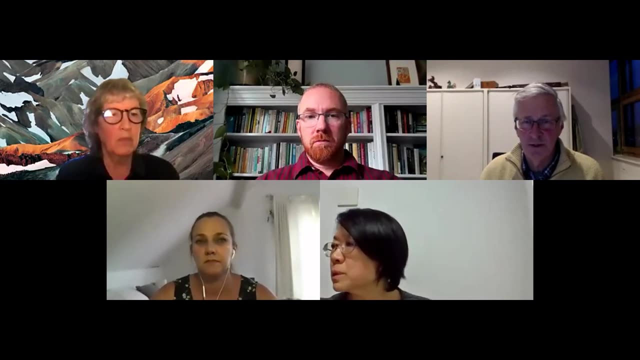 Wim, I know you might have something to say. Yes, Yeah, I know Ladislav very well, And if the fact that he could not get The soil um, um, um legislation through, I, I think hardly anyone can do so. 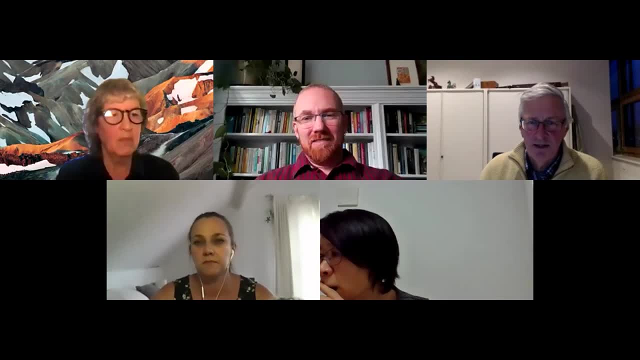 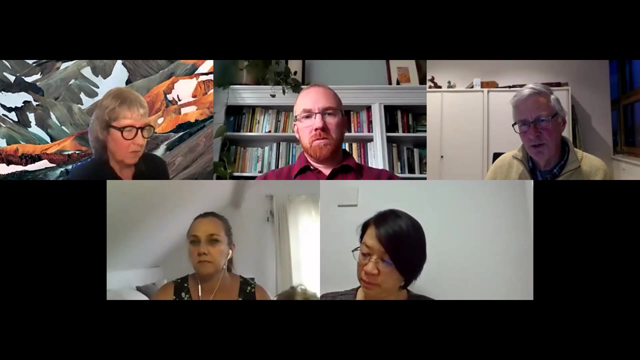 So, um, so I think the and and that is actually the. that is actually why we just went for soil protection through other policy areas. Um, and I don't think that good knowledge about soil biodiversity will lead to soil protection unless something really uh amazing would would happen that people will say: 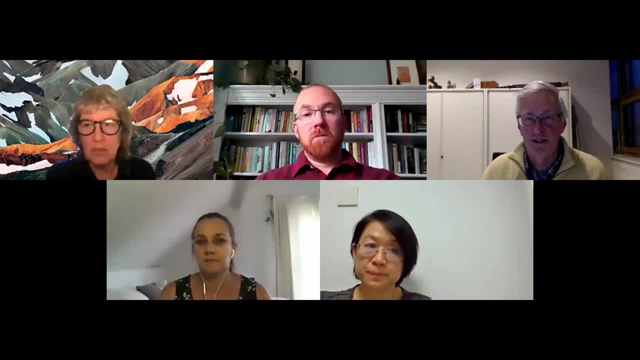 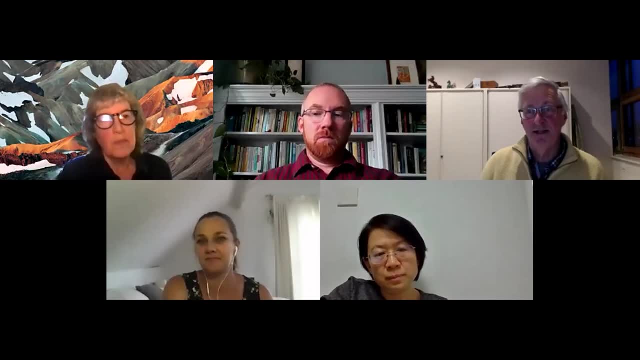 oh gosh, we are doing something bad for the tardigrades. let's protect them. And I think that the the fact that the different states, or the difference- and Ladislav has explained me in detail why the different states- were not collaborating, uh or not, um supporting 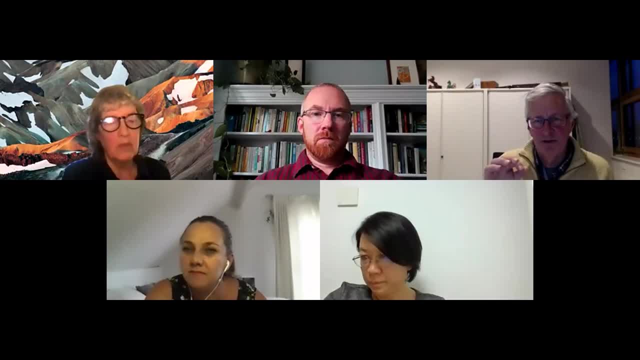 this, this legislation, and different states had different reasons not to do so, For example, the Dutch government. The Dutch government said- and I think that's arrogant, but it said: well, our legislation is so good. If you're going for your European legislation, then we are. we are going backwards instead. 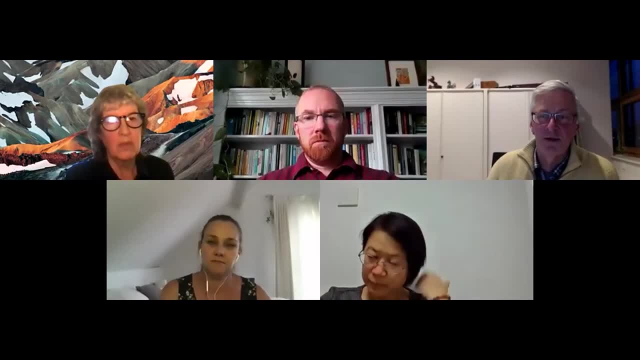 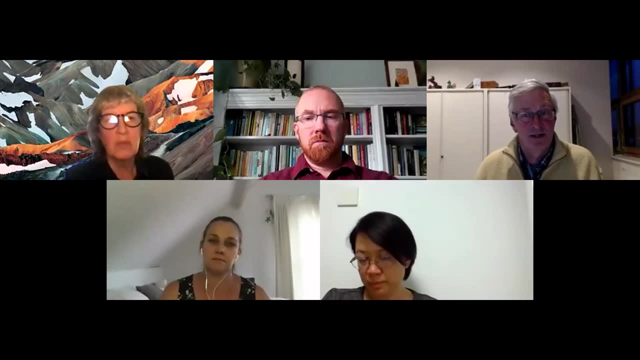 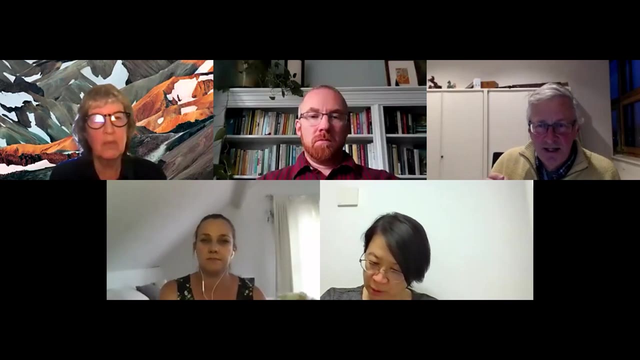 of forwards, And I think this is nonsense, because it's better to have everything, uh, better than only the Netherlands. very well done if it's very well done, And I tend to doubt if we do the best job ever. So, um, so I I think that, um, trying to go for a soil.